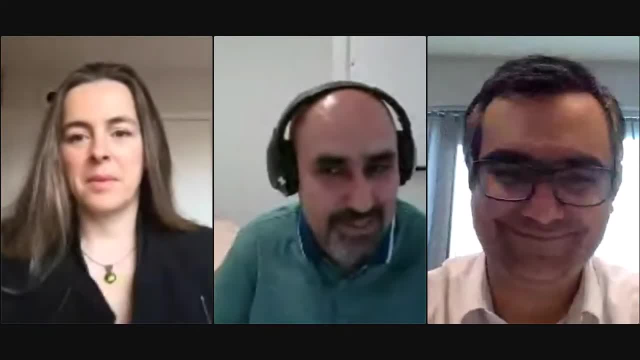 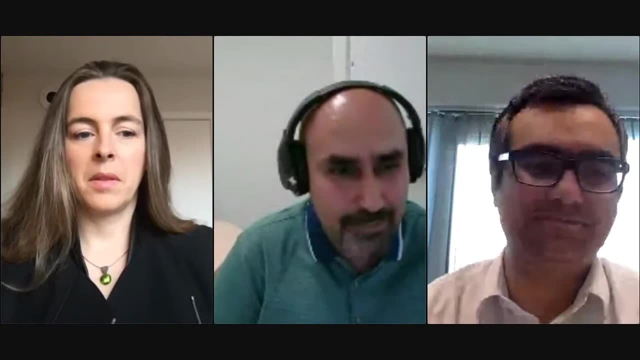 her PhD from the Harvard-MIT Health Sciences and Technology Program in the United States. She then completed a postdoc fellowship at Ecole Polytechnique in France before starting her laboratory in 2007 at Polytechnique Montreal in Canada. Her research topics range from: 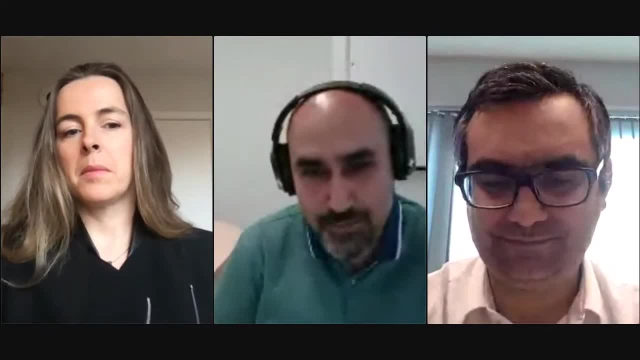 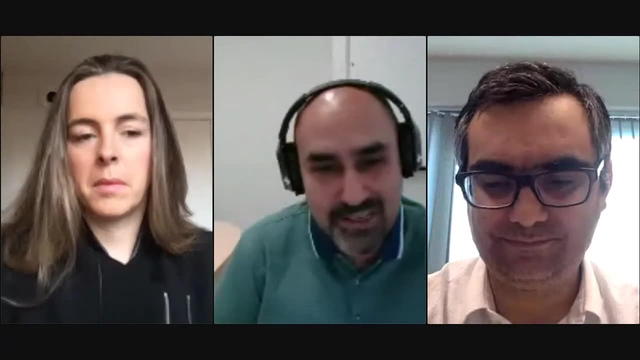 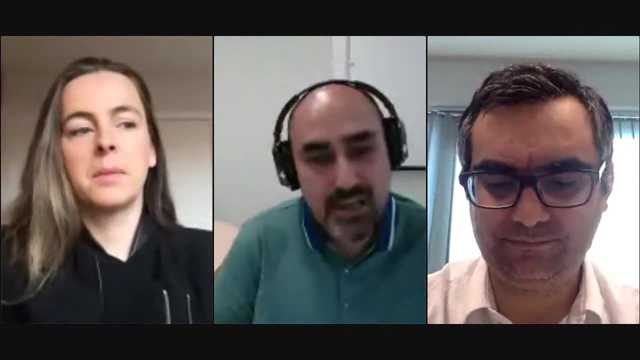 laser tissue interactions to non-physical level research to novel instruments for biomedical imaging. With a colleague and strategic investors she later founded Castor Optics, a spin-off company commercializing a new line of double-clad fibers couplers. Professor Bodo also has a book, has a textbook. 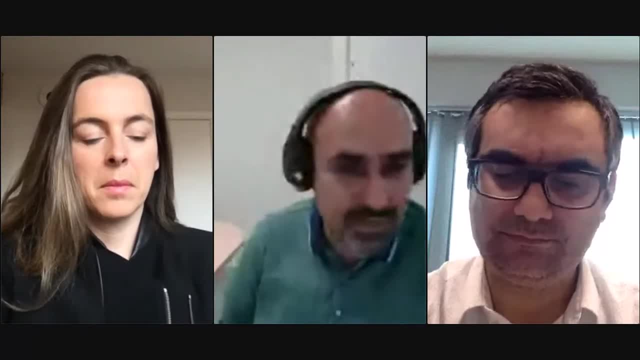 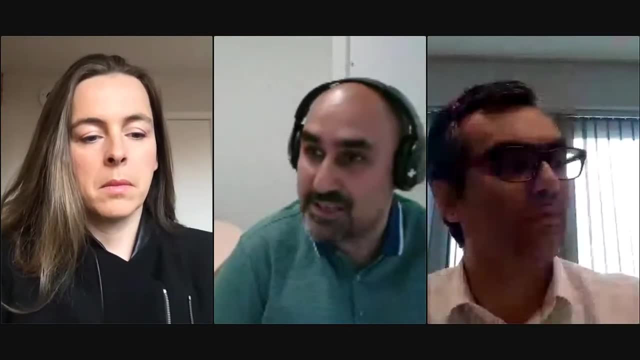 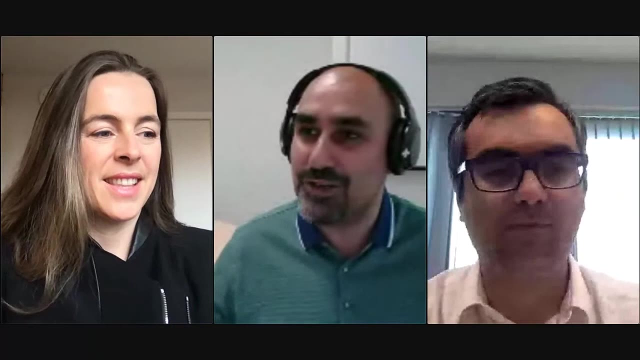 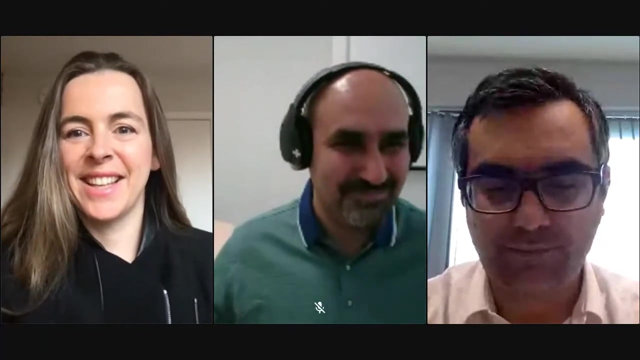 that covers a comprehensive range of topics in biomedical optics and biphotonics that is now taught in different schools and by herself, And by that I want to invite Professor Bodo to share her screen and start her presentation. Please, Let's see. 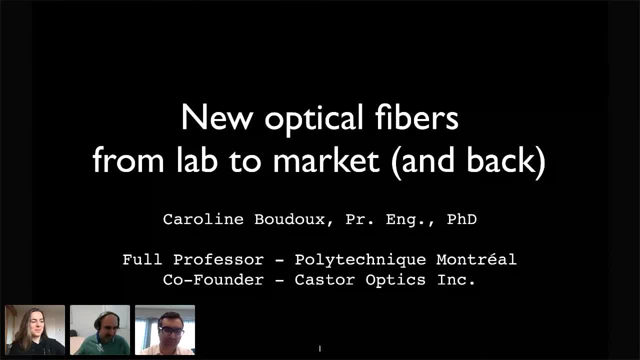 Is this working properly? Yes, perfect, Perfect, Thank you. Perfect, So you see my slide. Thank you so much, both of you first, for setting up this translational biomedical engineering e-seminar series I think desperately needed in these times of COVID. 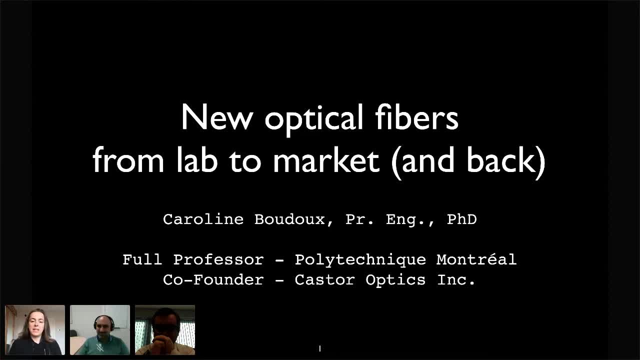 And I'm absolutely proud to be part of this seminar and thrilled to present to you today. We're going to talk about not just optical fibers, but optical fibers for biomedical engineering. So we're going to talk about optical fibers for biomedical applications. talk about innovations from the lab to the clinics. 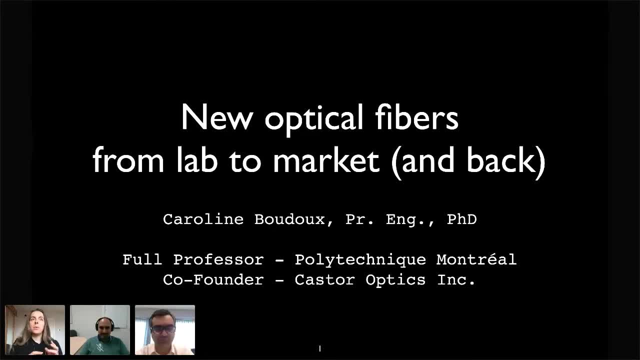 to the market and back. So how we started, as how I started as an engineering physics student, developing new techniques for the clinical applications, and then wonder how we can look at every individual component, make it better, sometimes patenting it. 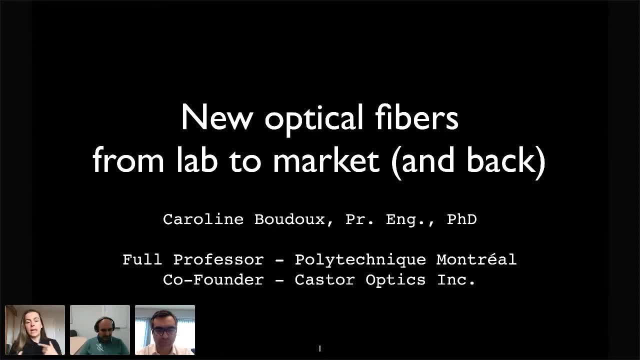 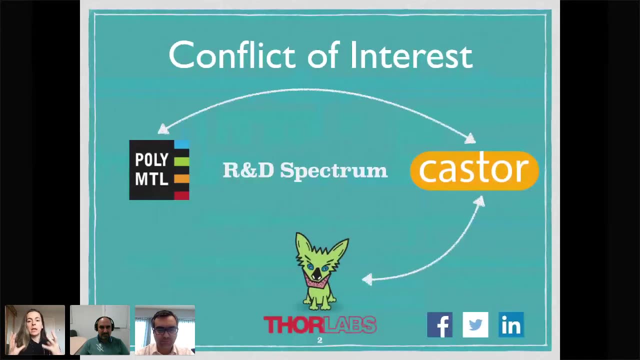 and commercializing it, and then hear about what the industry is saying about our products and go back to the drawing board and how essentially, the experience in the clinics and in the company is feeding my research. So I need to start with a slide on conflict of interest. 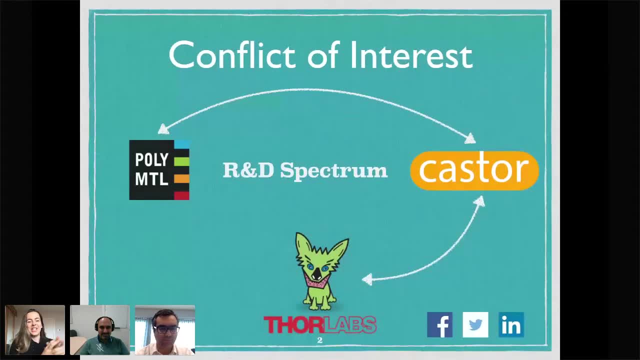 I have, as was said in the introduction, a lab at Polytechnique Montreal. I tend to see myself as a rookie professor, but Hooman reminds me that I've been there since 2012,. and I've been there since 2012.. 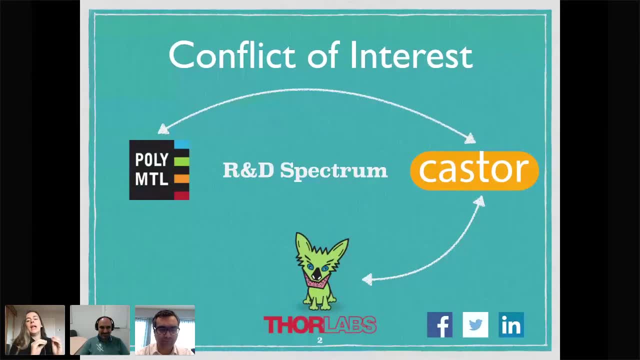 Since 2007,, so it's been quite a while now, And in 2013, we started Castor Optics. So Castor is an R&D firm and also manufacturing here in Montreal, in Ville Saint-Laurent, and we're strategic partners with a distributor. 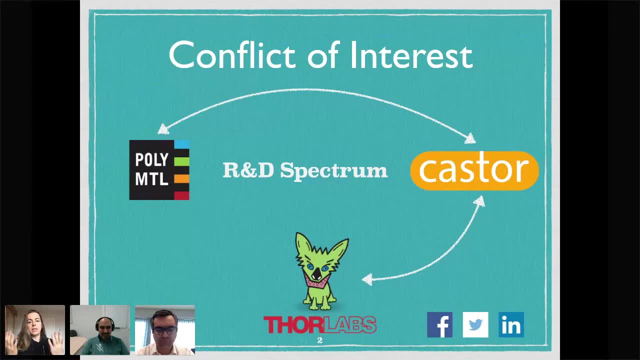 worldwide distributor Thorlabs. Essentially, how do I split my time? But, most importantly, how do I split ideas? If ideas lead to a publication, it typically is a performed carried through at Polytechnique Montreal. If it's a me-too product, so, for example, 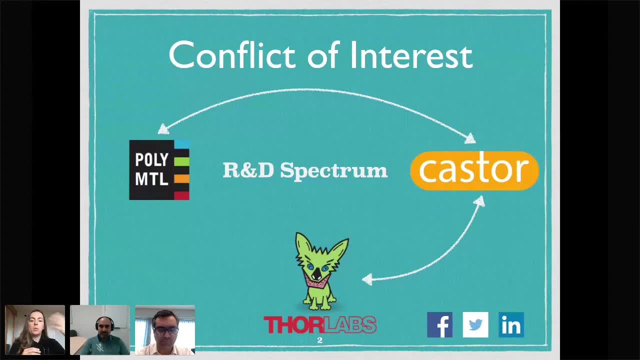 a fiber optics, a special fiber optics, but at a different wavelength. that is essentially a copy of a previous publication. the research and development will be done at Castor. But it turns out that now Castor is its own lab, its own entity. it creates its own IP and own patents. 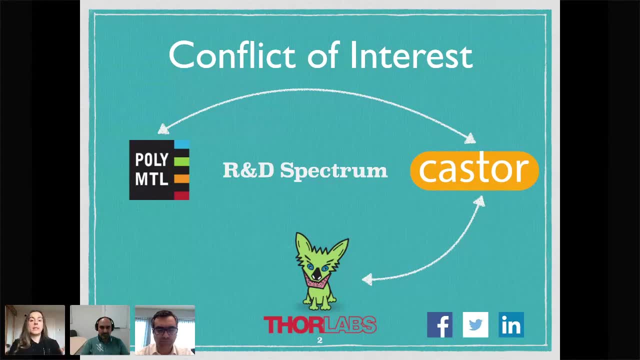 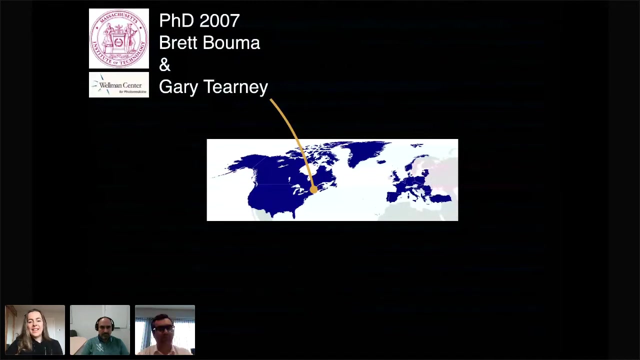 so now the separation is much easier to do than it was in the early days, But we tend to have a clear separation between the two and given my attention span of about 17 seconds, it works quite nicely. So I like to travel now with COVID, of course. 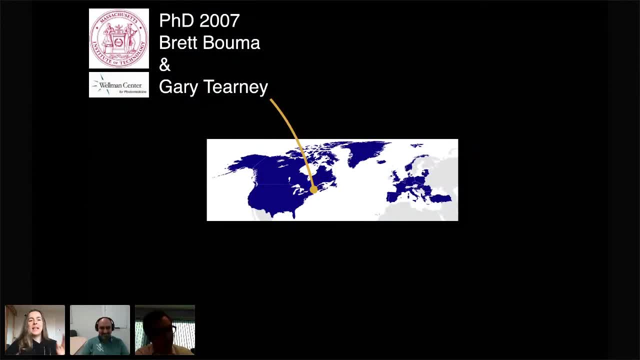 I'm a little more stay-at-home person, but I did my PhD in Massachusetts, then went to Polytechnique Paris to work on nonlinear microscopy- they call Polytechnique. My PhD was on biomedical optics, so optical coherence tomography. and then I did my PhD in bio-medical optics, so optical coherence tomography. 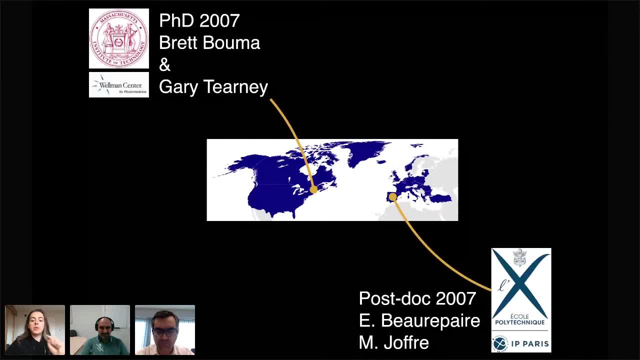 and then I did my PhD in bio-medical optics, so optical coherence tomography. and then I did my PhD in bio-medical optics, so optical microscopy. And then I started my lab in Montreal and I also took a sabbatical to finish my first textbook. 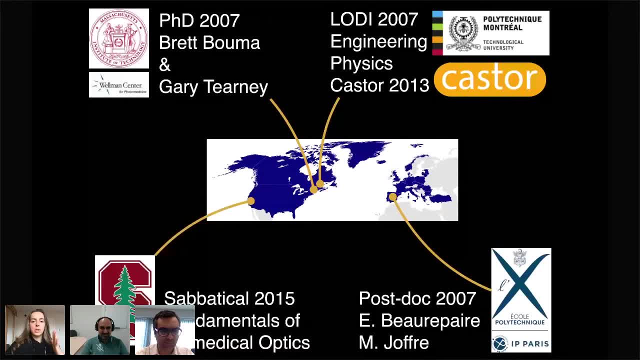 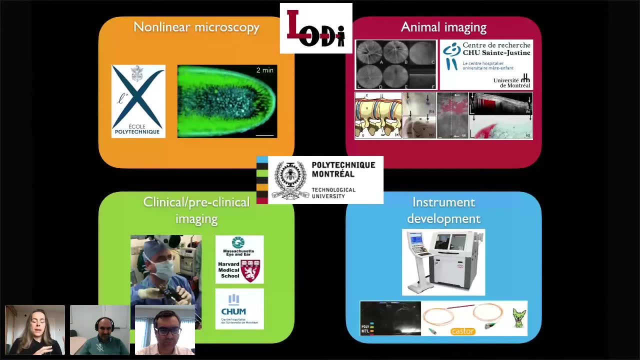 and I just got completely hooked to writing textbooks, so now I'm writing my fourth textbook as we speak. There are several activities in my lab and I'm not going to go in detail about every one of them, but because of my post-doctoral years, 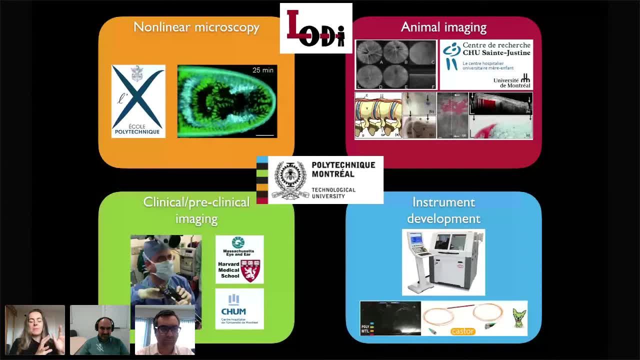 I tend to have nonlinear microscopy. Non-inner microscopy has a fond place in my heart so we are equipped to do rapid multiplexed non-inner microscopy at the school. I'm a full researcher at Centre de Recherche de Saint-Justine where we do our animal imaging. 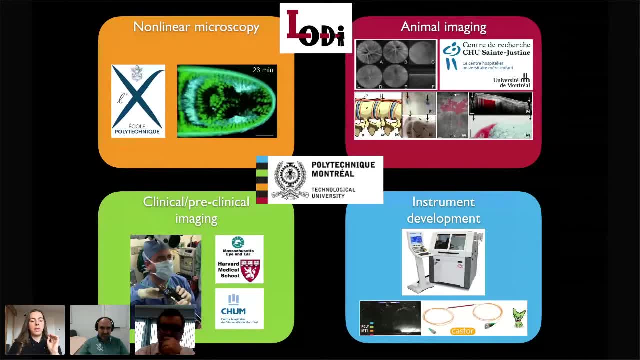 I was very much involved with Massachusetts Eye and Ear Infirmary back in Boston where we do clinical and preclinical imaging, And as part of my work within Polytechnique and at CASTOR we do instrument development. So those are the axes and you know, depending on the interest of the student, if it's hardcore physics versus engineering, physics versus biomedical engineering or even some clinical fellow, I can. there's one axis in my group where they can thrive. 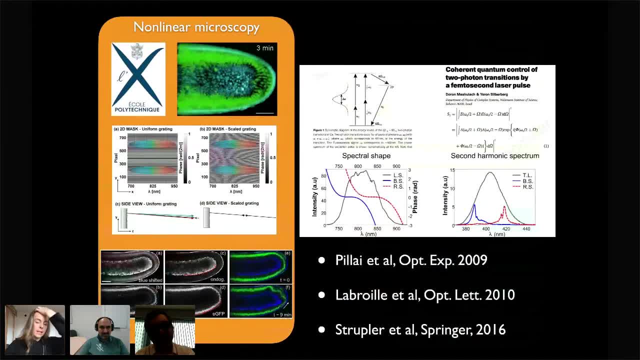 So we've done some work on non-inner microscopy, where we essentially exploited properties of light. So we've done some work on non-inner microscopy, where we essentially exploited properties of light, Especially ultra-fast pulses, to be able to excite simultaneously two different fluorophores with very high speed, switching speed between the two such that we could take 4D video- so 3D over time- of a developing drosophila embryo here with EGFP in the nucleus and natural autofluorescence in the yolk. 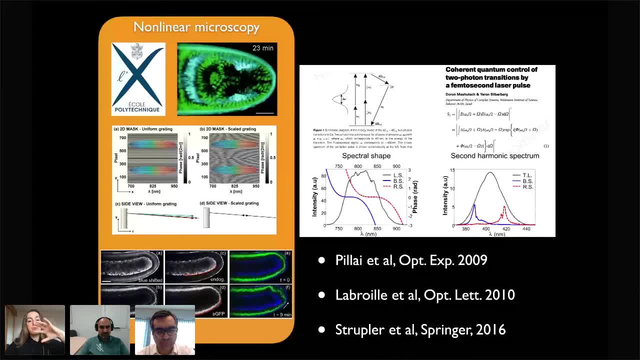 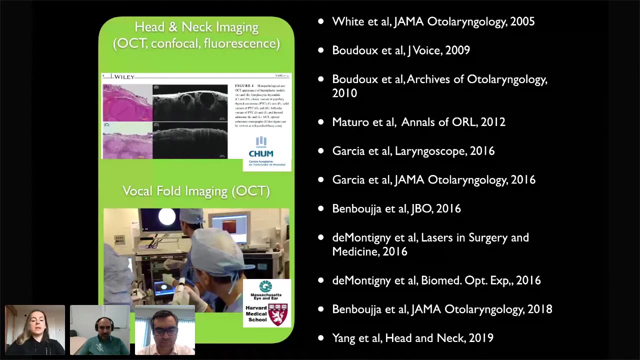 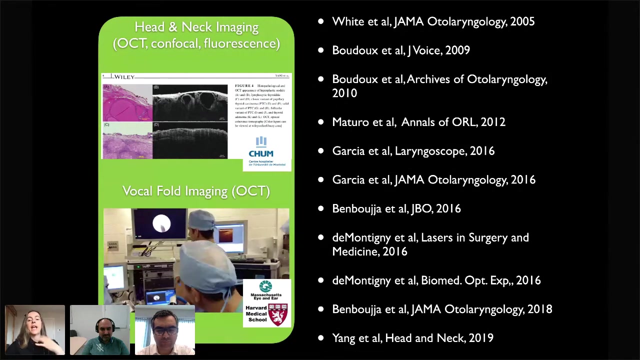 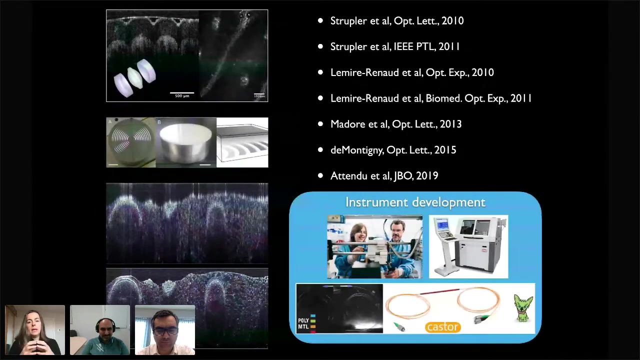 And so what you see are angiograms, And so what you see are angiograms, And so what you see are angiograms. And this one right here here in the middle, the, So, and this one right here here in the middle, the. position that's kind ofoulder's, where I'm gonna show you with a visual effect. but again, this is a beautiful, this is an amazing model where you, the students, can take soft возв決ions and light with a shooting light. time to be felt. 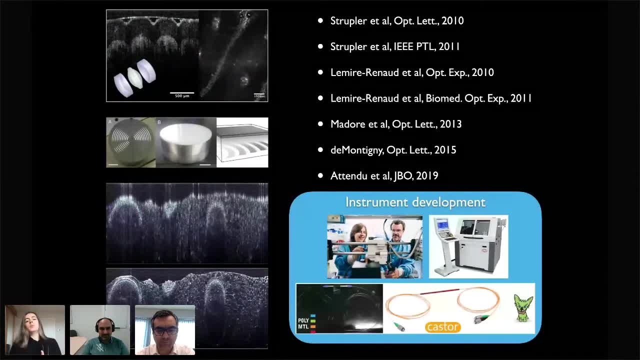 I'm safe. Yeah, Yeah, Yeah, Right, Yeah, yeah, the switch to go to the clinic to be translated. we also work on designing pieces that are going to be part of the next generation of those systems, and so, with professor nicola good, 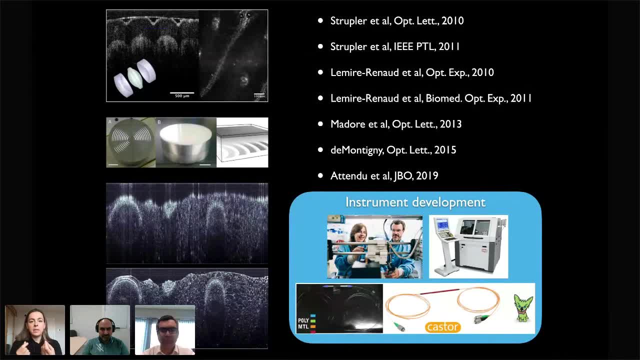 we come up with new fiber optics components. fiber optics allow you to bring light from a laser inside a patient and carry and and collect the light back to form an image or send a higher power laser and to do therapy. and we also do custom lenses. so we can do, we have a system to make. 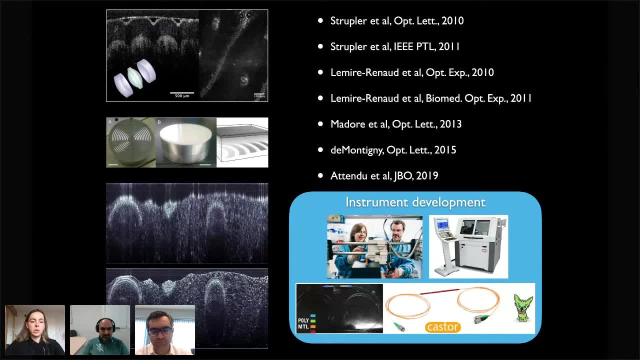 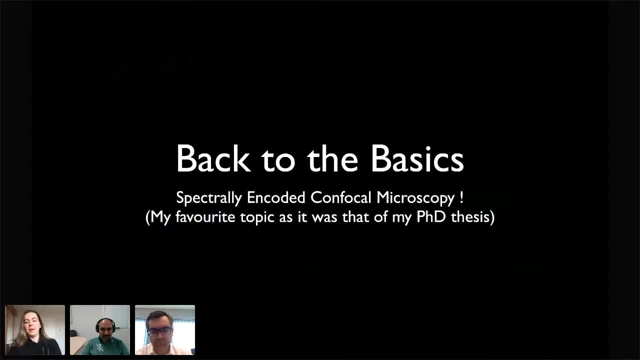 custom optical components to improve the quality of imaging, to remove dispersion, and so on and so forth. so back to the basics, back to my favorite topic, my, my phd thesis topic. let's start with one example where we started with an idea to very rapidly go to the clinics, learn from the clinic. 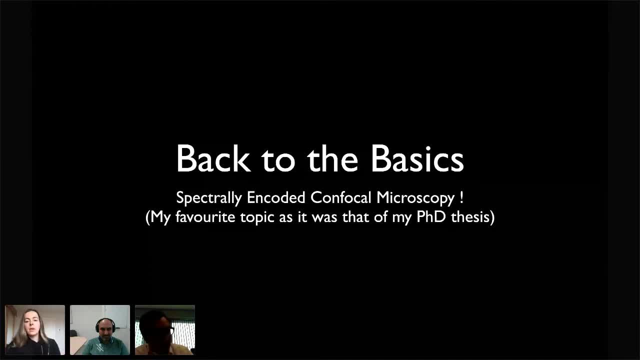 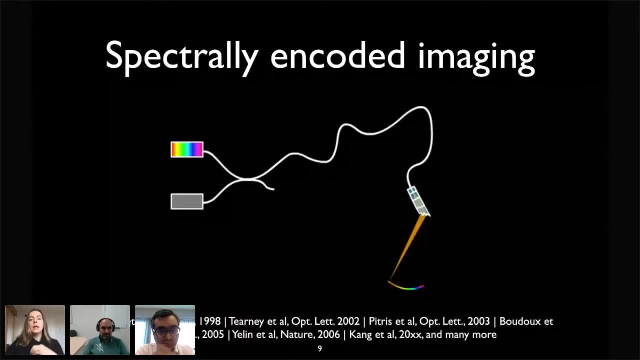 and then come back and say: what can we improve on? so an idea here was to perform rapid imaging within the body using the smallest instrument, and if you're trying to do imaging, some of the the challenges that you will see is: how can you miniaturize the scanner at the tip? 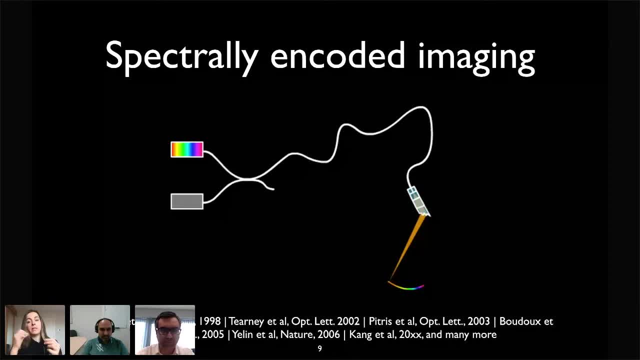 of your instrument. a fiber optics is very small. it's the size of my hair, so that essentially is the size of the instrument you can have. but how do you make the tip, how do you make the optics on the tip and how do you have a scanner on the tip to be able to get a 2d, read a 3d image and 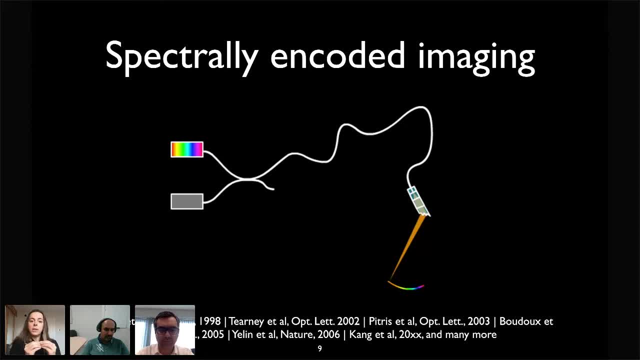 spectrally encoded imaging was one of the tricks that we played. we essentially said we started by dreaming and said what if we had a laser that were was changing in color very rapidly in time? and at the tip of the, the fiber optics, we put a prism. 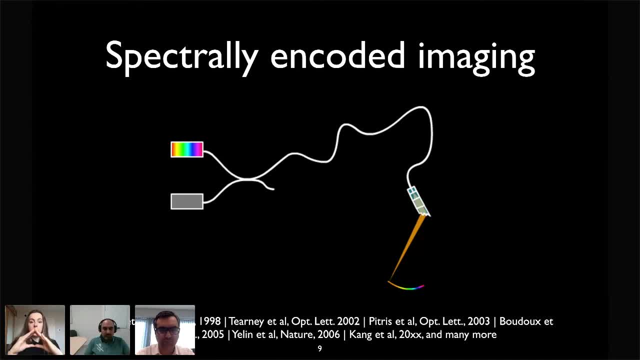 if we change in time, the prism will change the location of the light and if you have a scanning laser in terms of wavelength, you and essentially have a scanning onto your, your sample, of course. this is the image. uh, the the laser did not exist and the prism does not deviate enough, so we, we went with a diffraction. 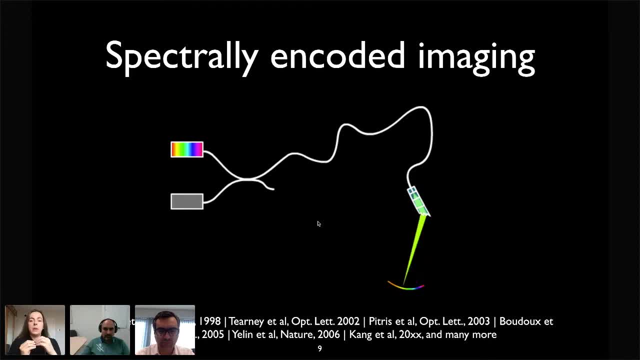 grading. this is what's displayed here and this is where we started. so my first contribution was designing a laser that was going to be able to measure the length of the wavelength of the light. so that's the first step, um a combination of light and light, and light using the laser that. 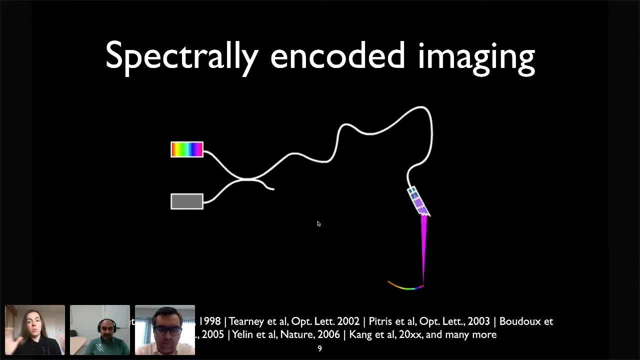 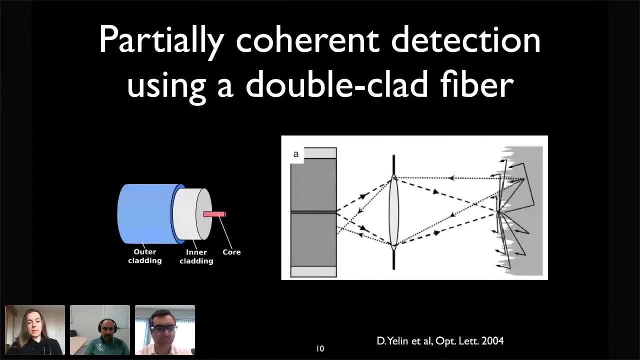 changes rapidly in in in time. so we now have lasers that can change a hundred thousand times per second, so we can do um imaging that is very rapid. but we also looked at the fiber optics. the fiber optics, as i said, is what brings the laser, the light, inside the body. so you go from the laser. 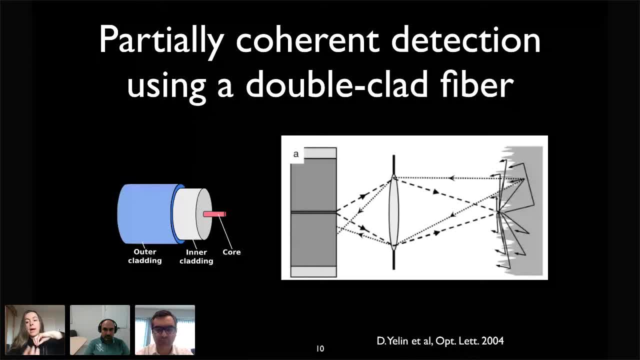 you. you bring the light through the body and then light will be reflected by or backscattered by your sample and collected by the fiber, and one of the problems that we had was that, in order to preserve all the properties from the laser, light could only be carried by. 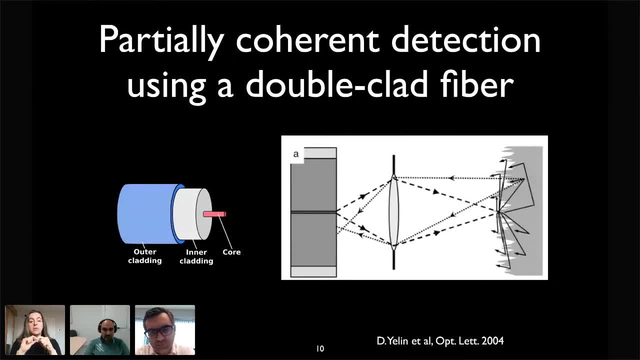 a single mold core, so a part of the fiber optics that is very, very, very small. when it hits the tissue, the tissue- and when i say tissue i mean any organs, it can be the esophagus, the stomach, any, any type of human material. it's not like a mirror. you don't have a straight 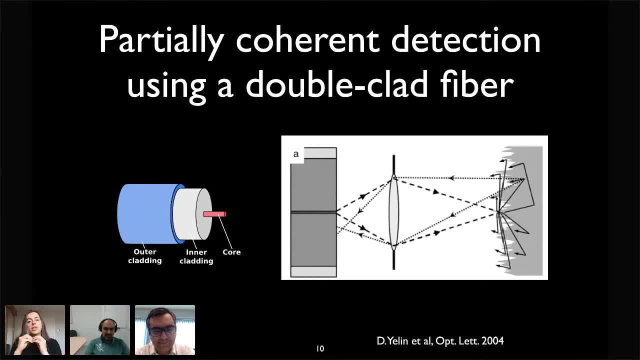 reflection back into this very small core. the tissue scatters quite a bit, and when it does you, you lose the face, but also you lose the directionality, and so very little light comes back into the core. in addition, since we are using a laser, what we observe is speckle, noise. 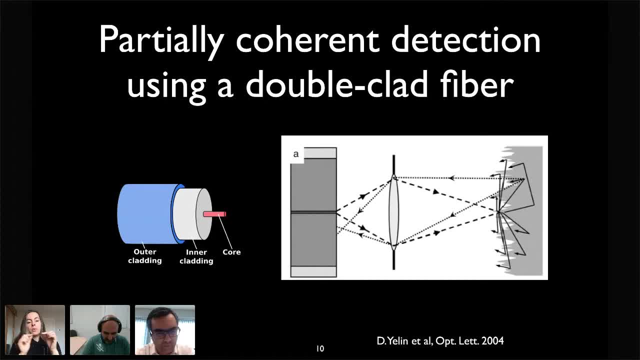 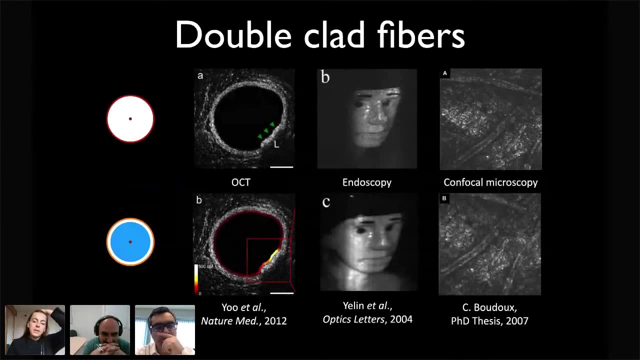 because our, our, our, the laser is coherent. if we only select through this very small pinhole the core of the fiber, the light, that is coherent, we are going to get interference noise that makes the image very tricky to observe. so if you look on on the top, you will see the kind of medical imaging that we do. 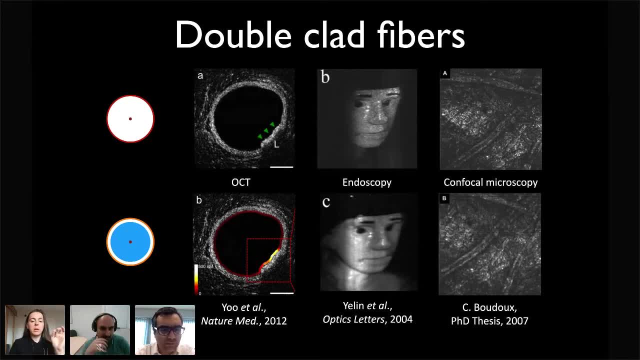 with optical fibers. with the single mode optical fiber we get, we can get oct images, so the new type of imaging that allows you to get imaging in depth, so you get sections of tissue. you can get a single fiber endoscopy as well where you see the face of this figurine and you can also 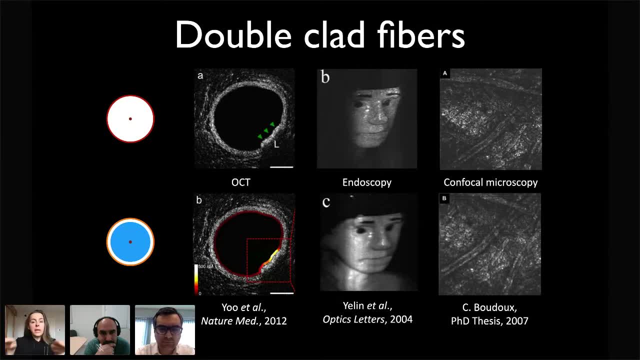 get confocal microscopy, but on all three of the top images what you notice is the speckle, noise right. the images are not smooth and that's due to using a laser but also a single mode fiber. so what we decided to ex explore was a new kind of fiber with labor- свой 16 and also poly�-q1 and 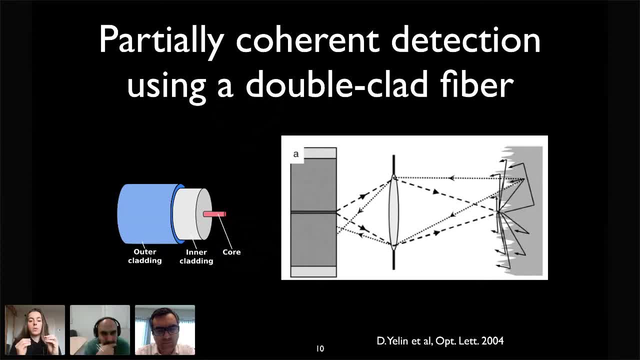 what we decided to explore was a new kind of fiber, that williska, that is laid based on the fibromyalgia lesion that has been already tested, we'reanga, and with a harmful abnormality. we want to include Caucasian cringe in order to show, cutting and tearing unnecessary breaks. 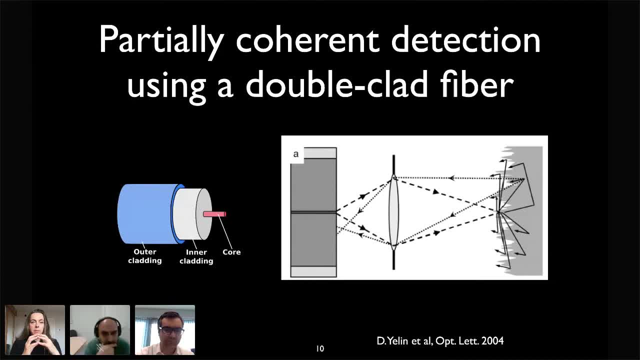 fiber called a double-clad fiber. It's a fiber with two zones, two concentric zones. You have the core, shown in red here, bringing the laser light to your sample, and you have the inner cladding that collects those scattered photons that have somewhat lost their phase, and so they 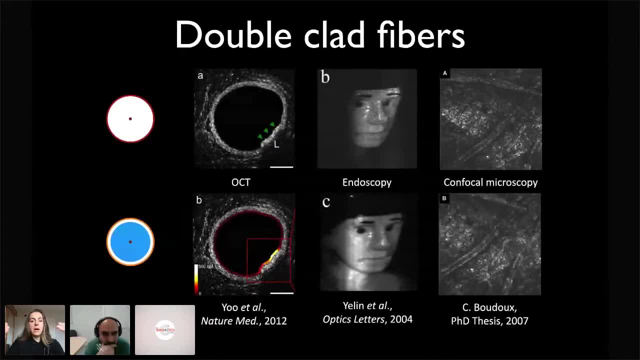 can scramble in phase and get a smoother image. So now if you implement the double-clad fiber into your imaging system- that's the row in the bottom in your endoscopy, in C in your endoscopy image- you see the image is much smoother. You get a much higher signal-to-noise. 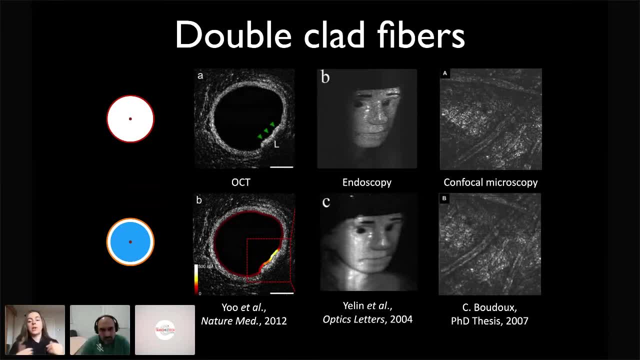 ratio, because you have a much higher collection efficiency and your confocal microscopy image is also smoother In OCT. what it allows you to do is collect spectroscopic information. All those photons that were lost in the core can now be collected by the inner cladding, and because 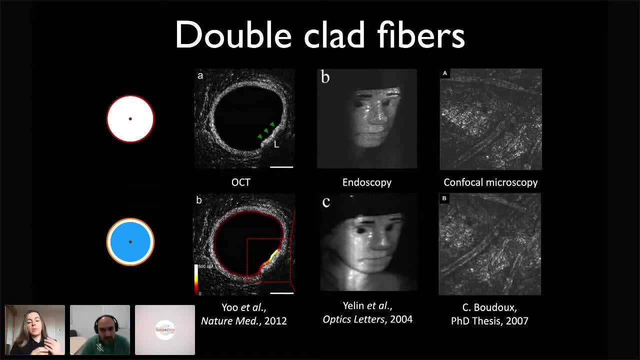 you have so much more of them, you can analyze them with a spectrometer and then find some molecular information. So this is where, starting with this very simple idea of an endoscope being a new laser, a fiber optics and some imaging head, we do the imaging on biological tissue. 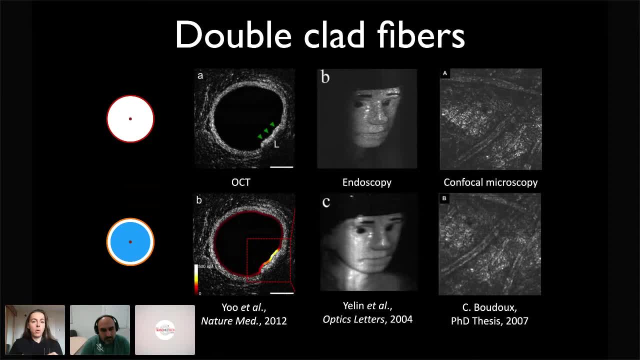 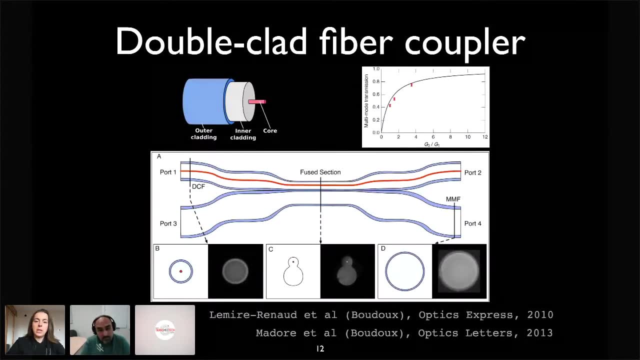 notice the speckle and go back to the drawing board and say how can we make the fiber better? So this was essentially the conclusion at the end of my PhD. Conclusion is: we need better fiber couplers and we need dedicated fibers for imaging, not just to carry signal under oceans for telecom. 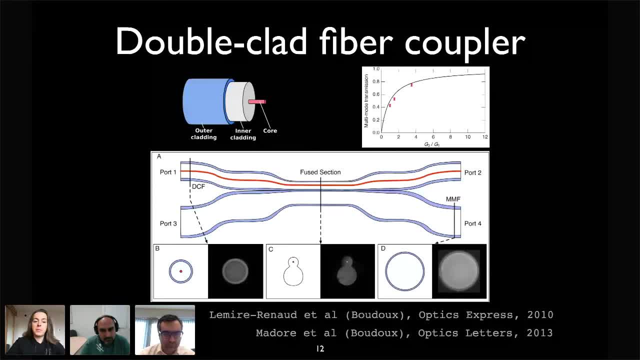 but new fibers for imaging. So this is where I joined Polytechnique and then I moved to Polytechnique because of laboratory For 25 years. then there was a laboratory called the Optical Fiber Lab And they were experts at making fiber couplers. So those are fiber arrangements that allow. 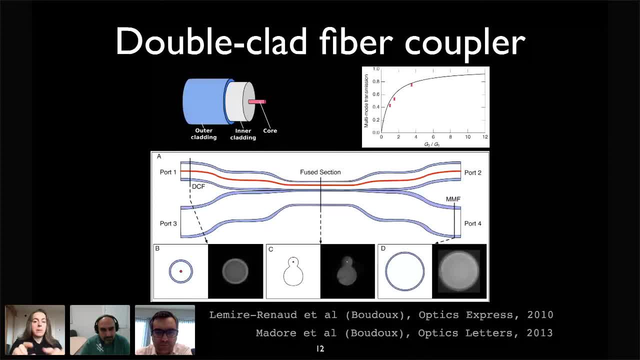 essentially communicating with different areas of the fiber very selectively and very efficiently And, as I said, this is not an easy task because the fiber optic- the core, is essentially the size, not the core, but the fiber optics is the size of my hair, And if this has three different areas, 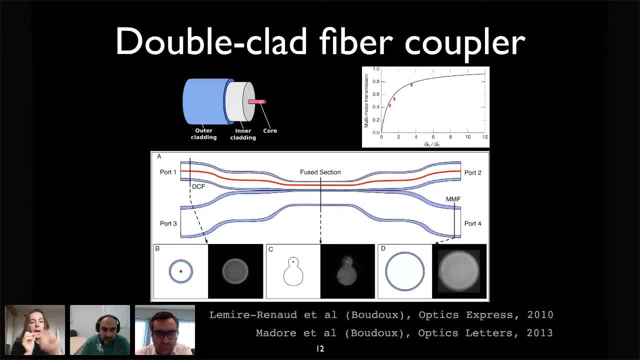 so the core is nine micron and the inner cladding is 100 micron and the outer cladding is 125, how do you only talk to the core or the inner cladding without talking to the other sections? And this is the specialty of Laboratoire des Fibro-Optiques. So we came up with a coupler. 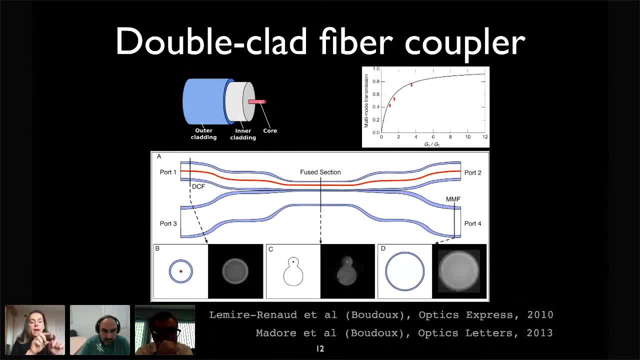 that allows us to go from in schematic in A, from port one to port two in red. So that's the laser delivery path losslessly. So there's no loss in your fiber delivery. Now, if you have some of those ballistic photons who are coming from the inner cladding and you're not able to talk to the 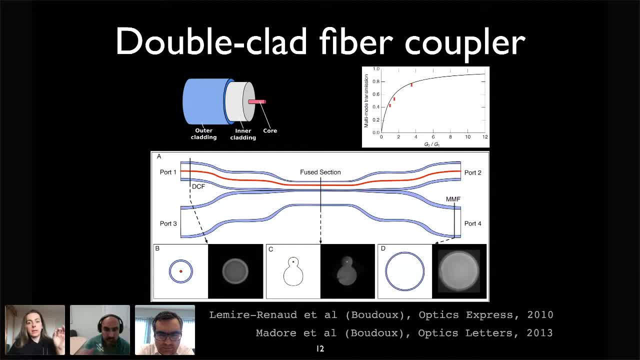 outer cladding and they're coming back from port two. those are very precious and you can collect them. They move from port two in the core to port one losslessly. So you still collect those very high information but low throughput photons. So you have them, But all the photons that are. 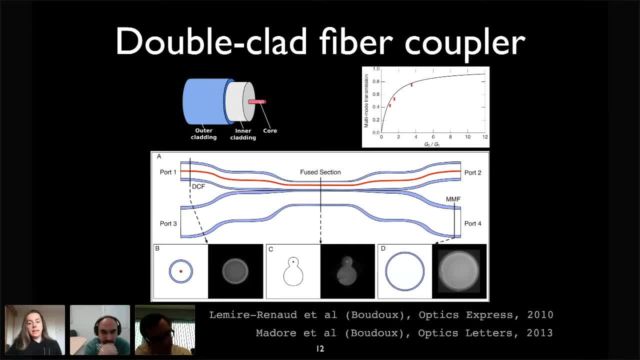 backscattered from the tissue. they are collected in the inner cladding at port two, shown in white, and most of them will be redirected to port three. So by inserting the inner cladding, this new device, into a fiber optic endoscopic system, you can collect a hundred times more. 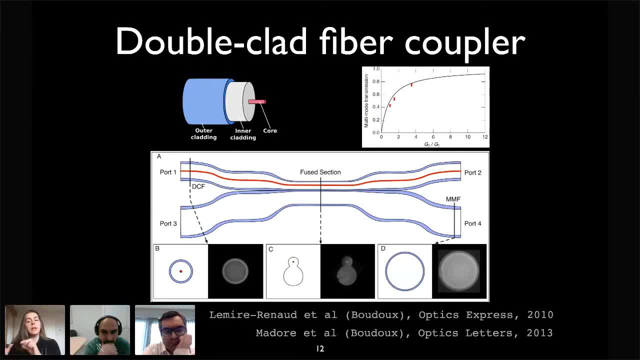 photons and they have different properties granted. but you can exploit the second channel that comes for free, the second channels, and you can, if you know the properties of light, you can exploit them for different clinical applications. So this was our invention. 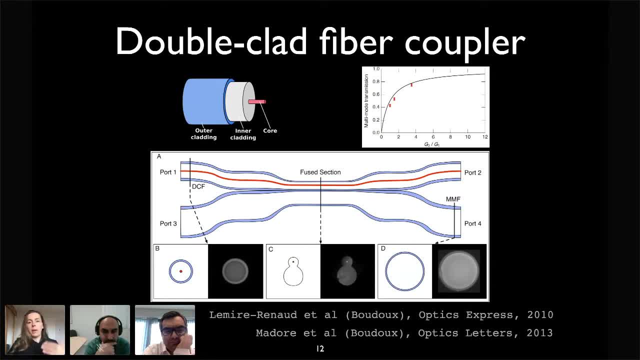 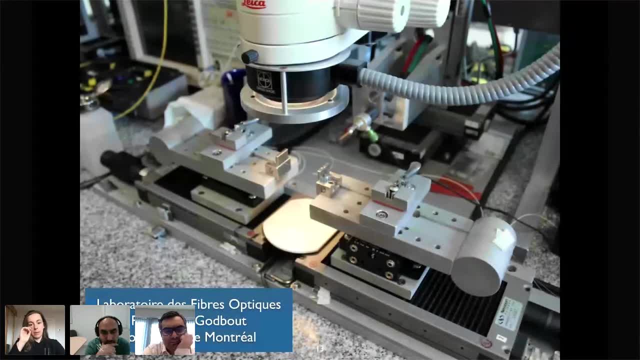 and we spent three years refining it. So you see several papers: 2010,, 2013.. This is how it's done and I can tell you how it's made, but then I'd have to ensure you keep privacy, So let's not discuss this too much. but this is the pooling, the diffusion. 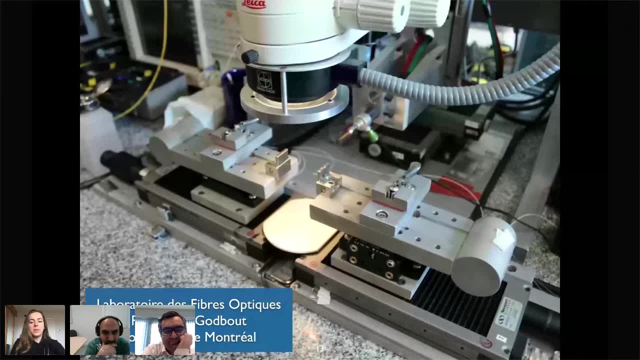 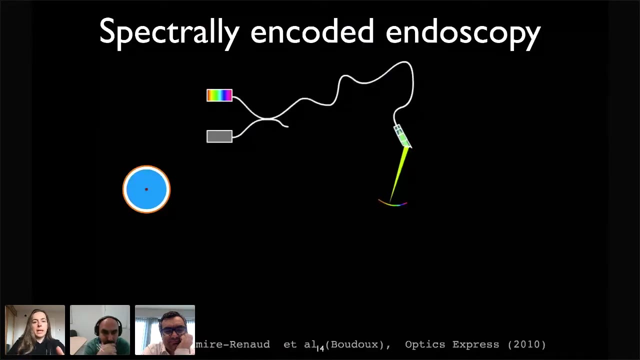 tippering system in Professor Godbout's lab, where you see exactly in the center that the bright filaments are the two fibers put together and this is where the coupler is being made And it allows us to do the same type of imaging. but we can. we have still access to light from the core. 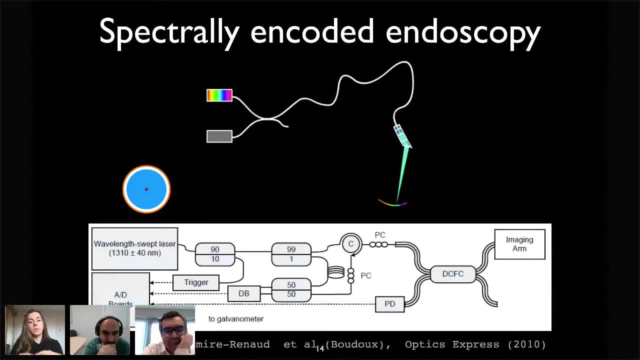 which is great, but we can now have the light also from the inner cladding, So we're essentially adding an extra modality that exploit photons coming back from the tissue that are a hundred times more intense, And of course, I'd be happy to discuss for an hour this particular schematic. 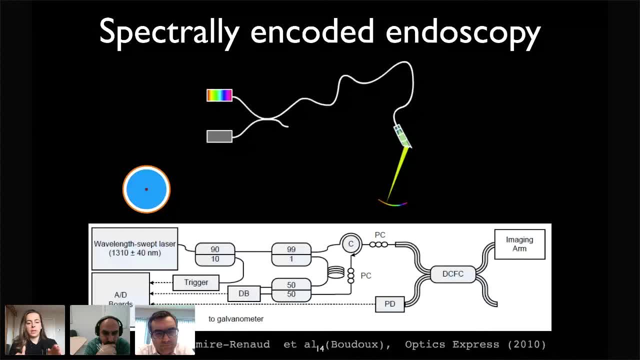 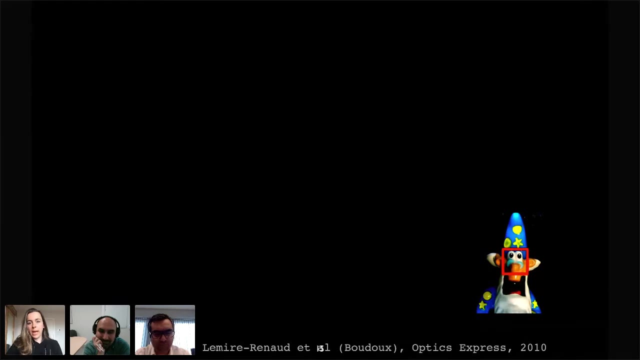 This is how we we make the circuit. but I think the important point for today is to show that all the black lines are fiber optics and this is an entirely fiber based system, So there's no free space. this is robust, you can go to the clinics and back and you don't have misalignment. So before going to the clinics, we test in the lab and we, we, we are chocolate lovers in the lab. So we have in Canada what's called in Europe, what's called a kinder surprise egg, So it's a chocolate egg with a toy inside. 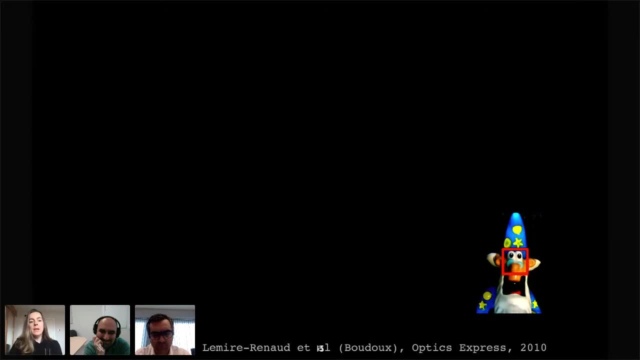 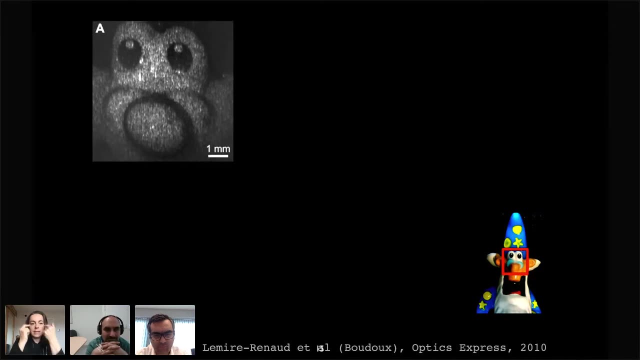 so that gives you essentially the dimension of the little toy that we have. this is merlin. so with our previous system we take an image of merlin. you see its nose, its glasses and its eyes, but again you see how much the speckle, uh, how intense the speckle noise is, and for you it's easy. 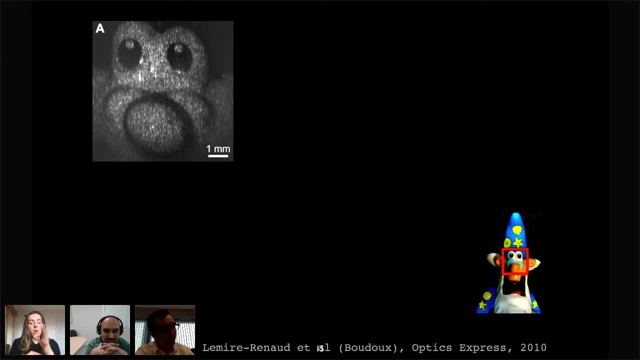 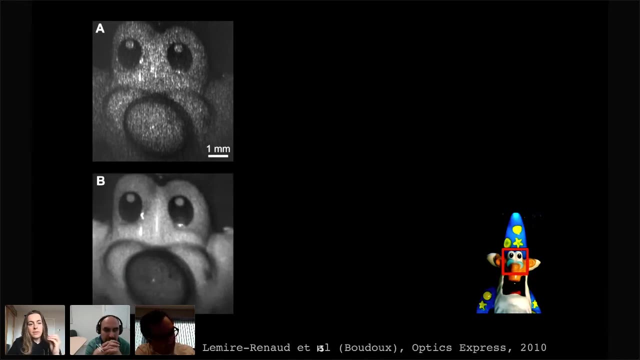 to see that it's merlin, because you've seen merlin. but if you're doing endoscopy you're going blind and you don't know what you're you're looking at, so the speckle noise is really disturbing. by changing the fiber, you get still the same illumination from the core, so your laser goes. 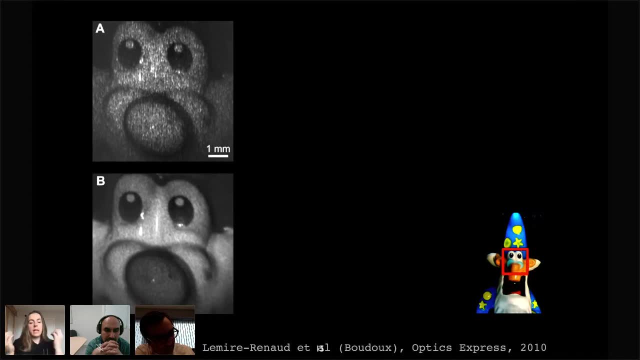 losslessly to your sample, but you can scramble the image coming back and you get a much smoother image and a much more intense image. the signal to noise is a hundred times greater. the photons in a are still available, though you collect these two channels, a and b, completely. 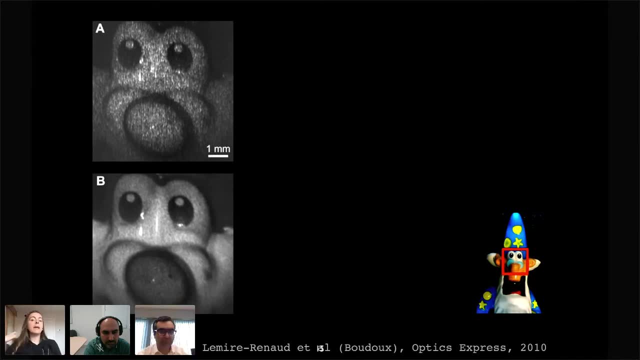 independently and because a has speckle, it has some phase information and if you remember your sophomore year physics, or even maybe some some interferometry that you see in college in wave and optics, you know that from the phase you can reconstruct the depth. so now, by just adding this coupler to a single fiber endoscopy system, we can get. 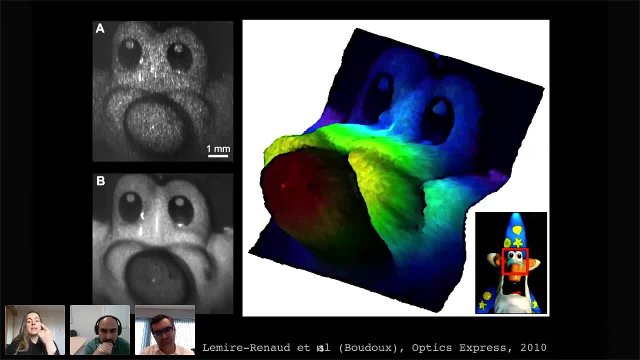 a speckle free image, much more intense, but that is, you can also recover the depth. so, for example, if you were to image an ovary and there was a tumor, you would see a bump showing in the red. you get the, the three, the, the third dimension for free using this, this new technique, of course. 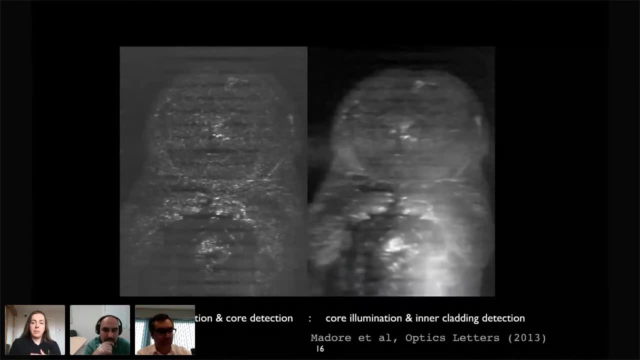 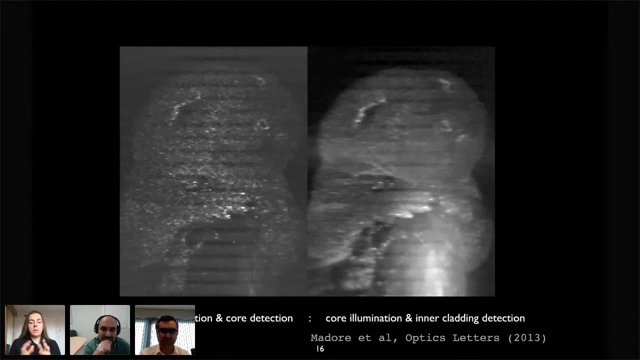 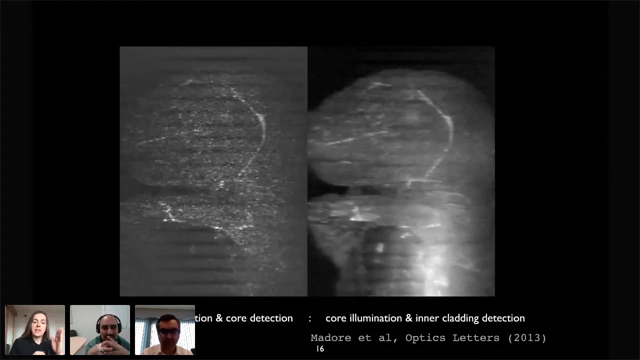 my idea of of translational imaging is not just to image kinder surprise toys, just to know which one there is before you eat the chocolate. the idea was to try it on biological systems and this is where we tried it on the mouse embryo. the image with a single fiber on the left and the image 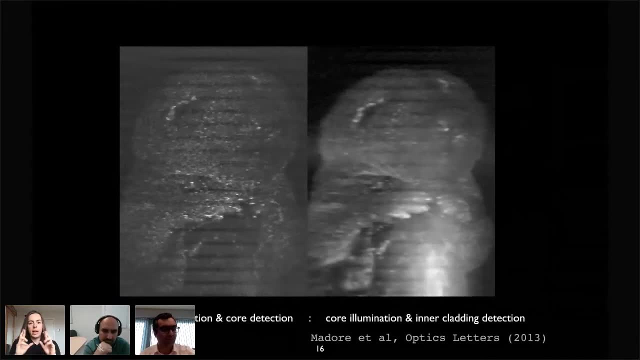 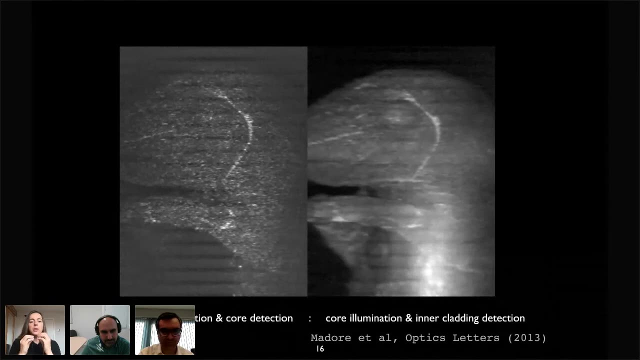 from and i hope this video is showing is showing on my screen, so i have. i have hope that you guys see it as well. but you see how the, the signal to noise is much, it's much deeper. you have an attenuation, a speckle, and you you can see the feature of the animal much better than by just 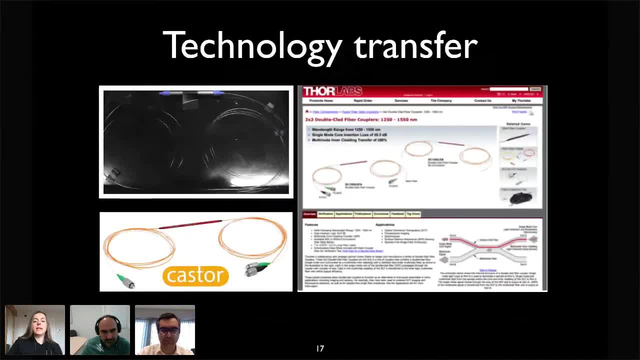 changing the fiber optics. this particular video led to technology transfer. of course we're academics. so we thought: you know the, the produce? uh, the product on the the top left was totally fine. and then our partner thor lab said: you know what, let's refine it a little bit before we put in a. 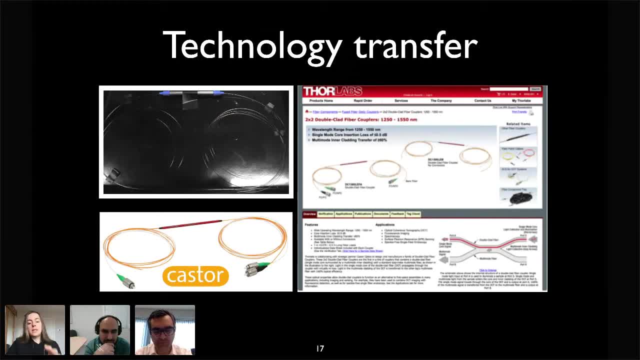 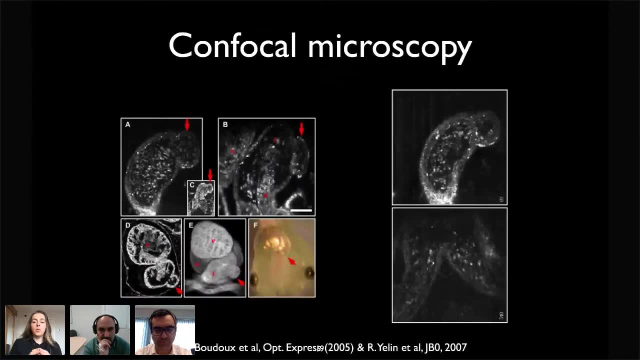 catalog. so now we are, we're producing here in montreal these um, these uh, um, instruments and and, depending on how much time we have, at the end i can tell you about the, the tech transfer as well. so, in terms of applications, um, one, one piece that was of interest, because, again, that's that. 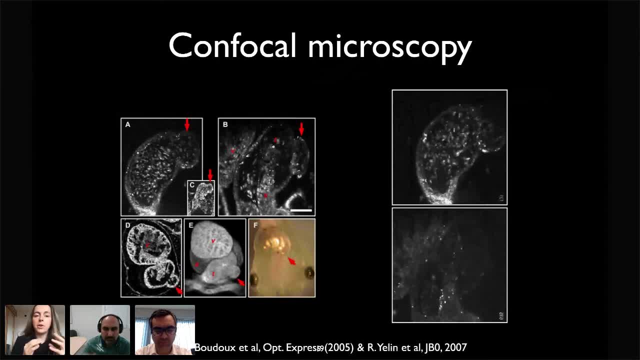 was my phd thesis was confocal microscopy and for for those of you who are not familiar with confocal microscopy, the difference with white field and confocal microscopies is that you can acquire virtual sections. so if you're looking at um a xenop embryo scene in f, 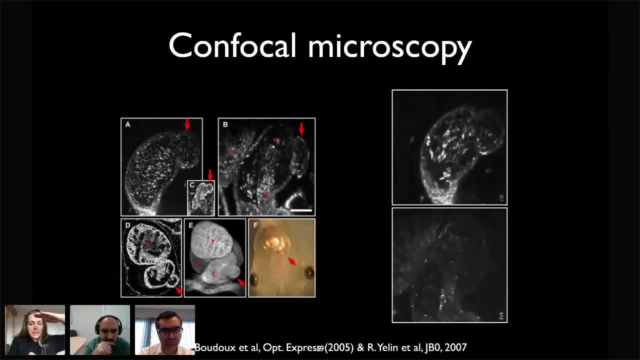 with a white field endoscope, a microscope, what you see is all the layers at once, and so the light scattering doesn't allow discriminate between sections. so an organ that is buried in the middle, even though it's a transparent embryo. the organ that is buried in the middle, the heart. 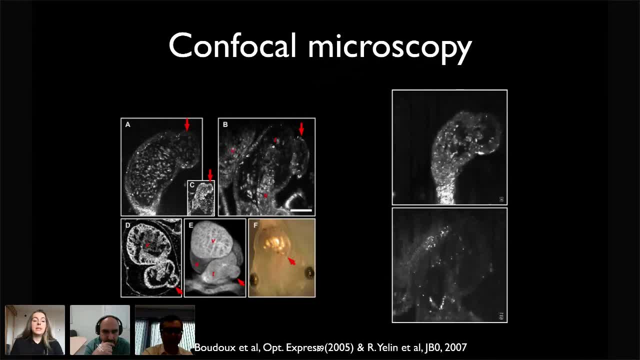 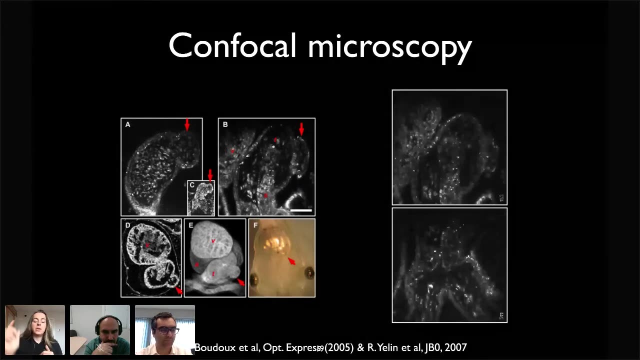 shown by the red arrow as can't be seen, And if you're imaging it with confocal microscopy, you can get virtual slices, And if your focal microscope is fast enough, you can get those videos. So these are actually red blood cells flowing through the artery. 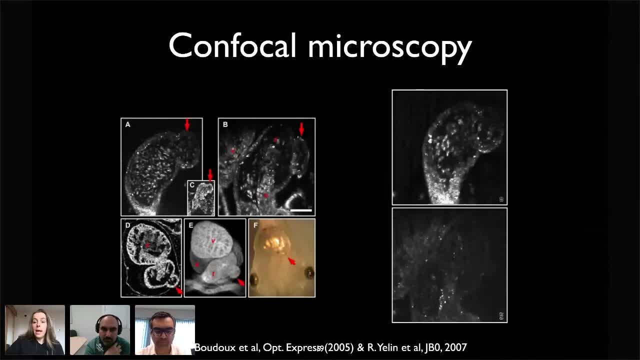 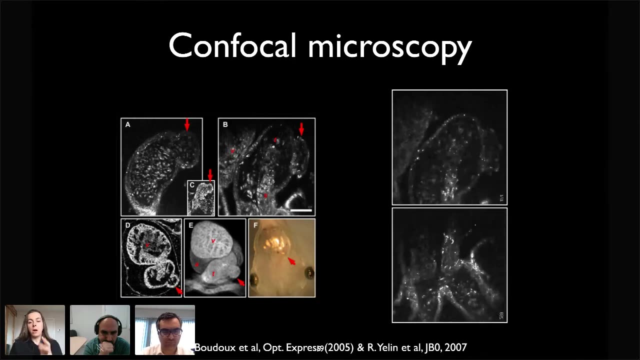 the artery loop near the heart of the embryo. And for those of you who are familiar with the architecture of the artery loop, you see, there's actually an aneurysm that was created in the lab by exposing the embryo and its mother to alcohol. 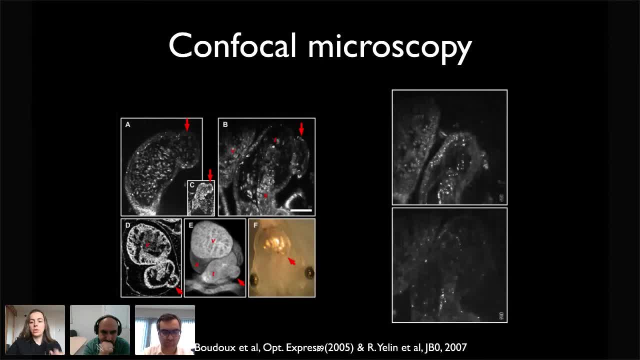 So this is a warning, as if we didn't have enough warning not to drink during pregnancy, So we could actually see the stagnation of the blood vessels within the aneurysm and the flow of blood through the heart. This is being done on a tabletop. 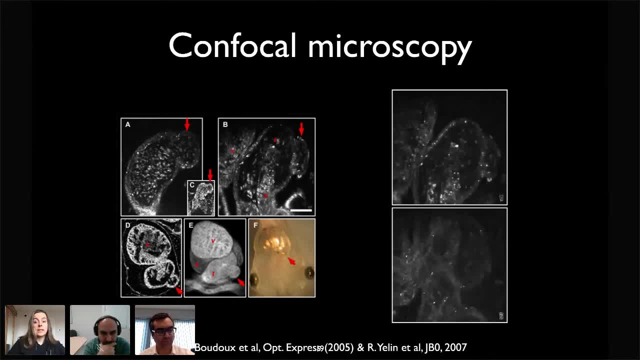 system and the idea is to bring confocal microscopy to the clinics as well, to translate it outside of the lab. And, as opposed to using pinholes in the lab, we're using fiber optics. They act as a pinhole and that's what allow the sectioning to be done. 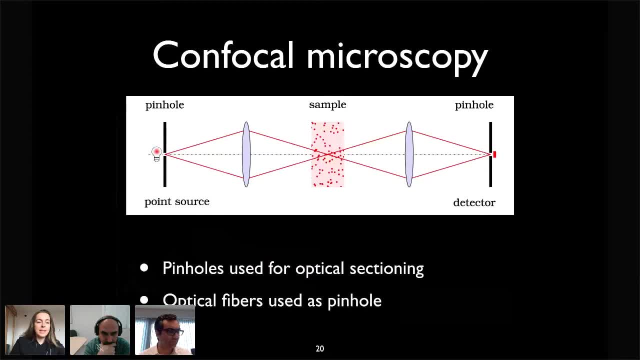 So this is the schematic from Minsky's patent, Of course redrawn for the purpose of my textbook, but the idea here that by using pinholes you can get rid of the scattered events, and you can. you know, you can see the red blood cells. 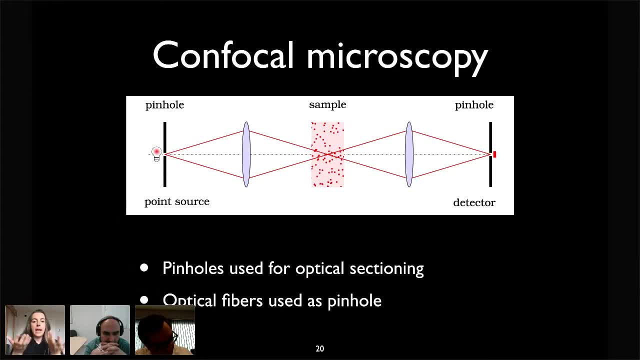 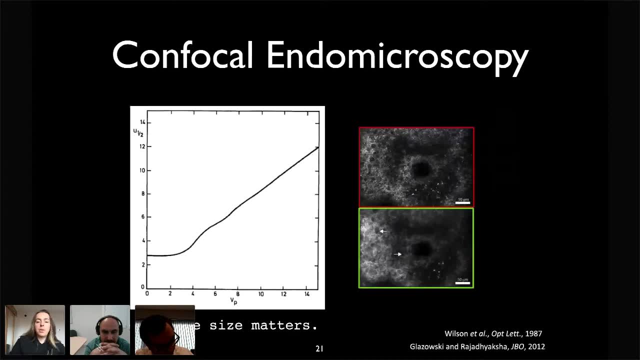 you can reconstruct photons from a plane and essentially make abstraction of everything that was below and after, up to a certain depth, And people had shown that you can improve the size of the pinhole to increase the SNR. So if you're the image that is shown in red, 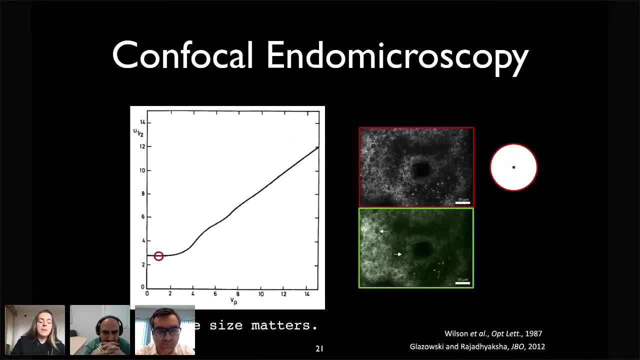 this is image of the skin taken by Milan Rajadakshya. If you have a single mode fiber or very tight pinhole, you get low signal and tons of speckle And you can improve a little bit the smoothness of the image. 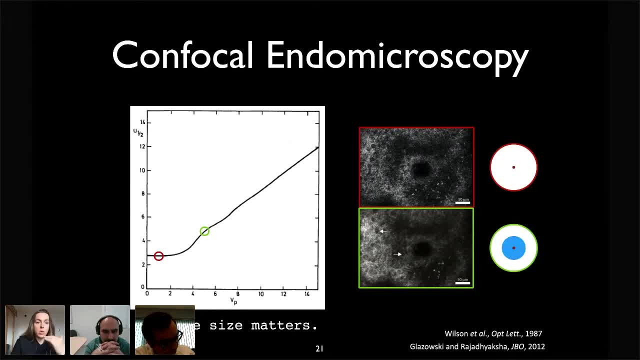 and the signal to noise by opening the pinhole, And in our world that means opening the fiber a little bit. So what you see here, the cross sections on the right, are cross sections of our fiber. So the red dot is the core and the red and blue 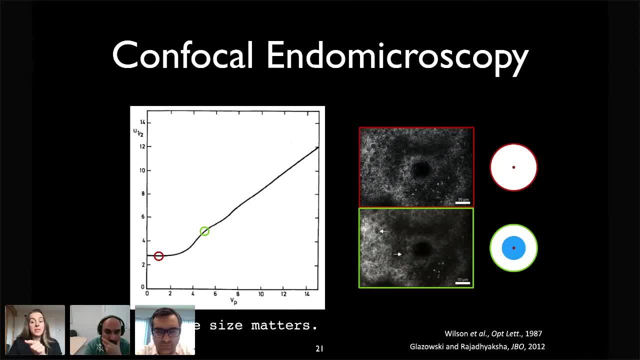 is the dual cloud fiber, But it's very different from the dual, the double cloud fiber that I've shown you earlier. The first double cloud fiber- the dual cloud fibers that we worked with- had a really really wide inner cladding. 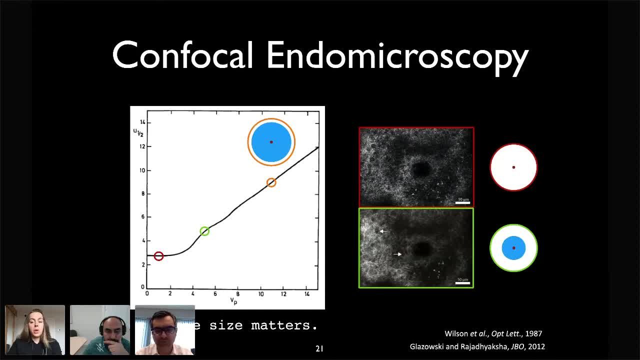 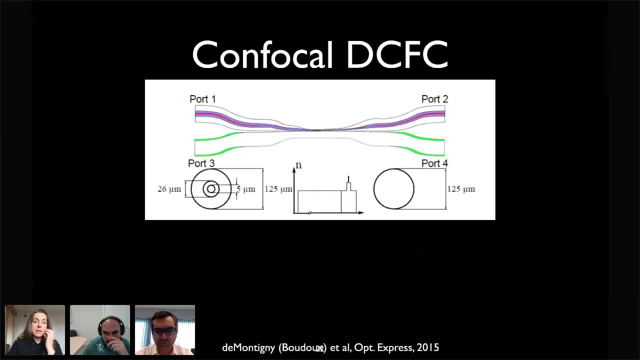 And so we had to go back to the drawing board to be able to make a coupler with this new geometry of fiber, And it looks like such an insignificant difference. but some people had postulated that you couldn't do it because you have such a big barrier of glass to go through. 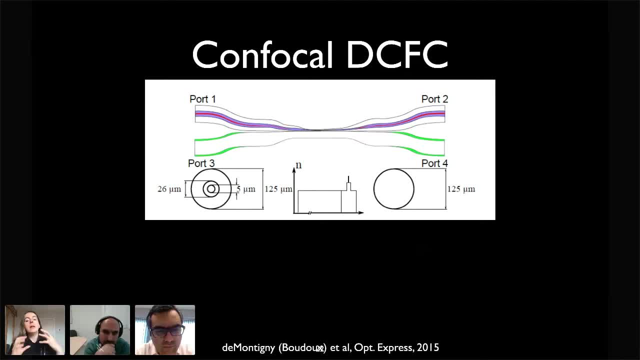 And so one of my students, Etienne de Montigny, thought of a very clever trick with the group to. so he exploited a trick where he pre-tapers the fiber to trap light from the inner cladding and to make a new coupler with this. 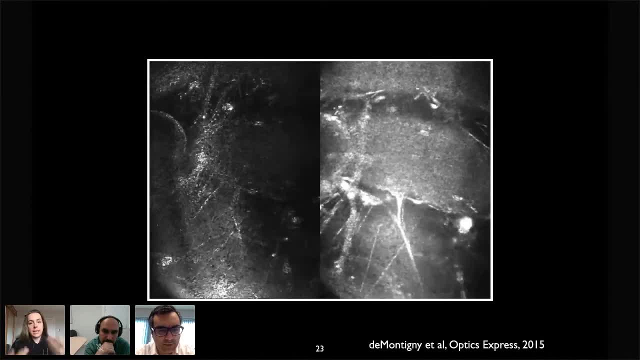 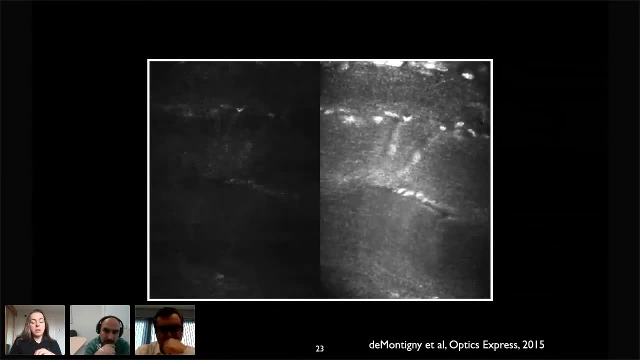 Long story short. we now have a new coupler dedicated to confocal microscopy image. So these are: confocal microscopy of muscle, skeletal muscle. On the left, the image for the single mold fiber. On the right, the image with the double cloud fiber. 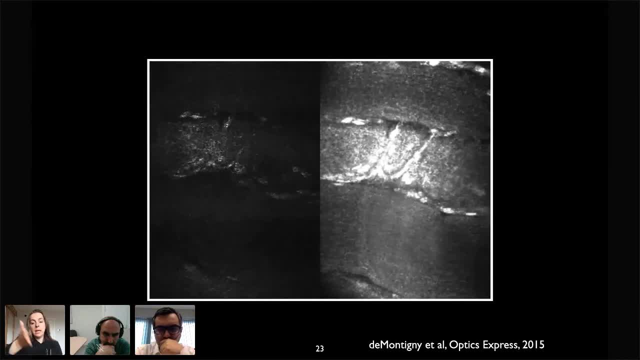 And you can see in the fiber in the bottom. you can see, and you can see in the fiber in the bottom. and you can see in the fiber in the bottom. you can see in the striation of the multi-mold fiber. 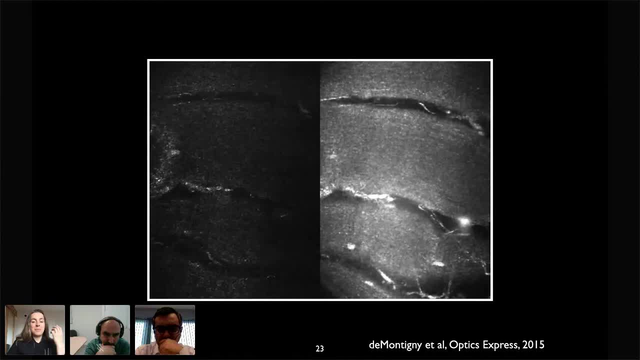 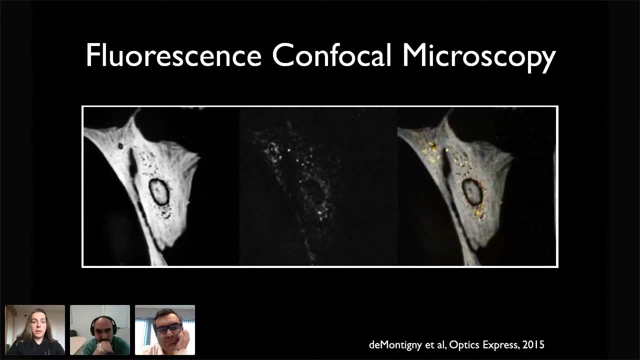 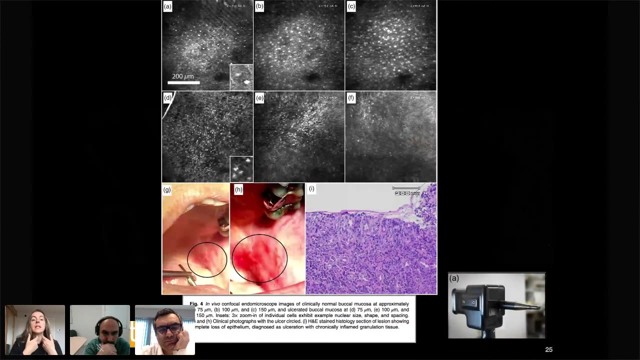 So we don't lose the resolution and we also increase the signal to noise just by designing a new fiber specifically for confocal microscopy. We also showed that we can collect fluorescence through the inner cladding, and some collaborators of us have used it to make a confocal microscope. 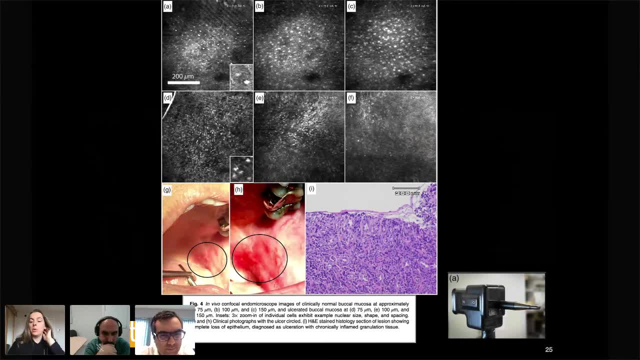 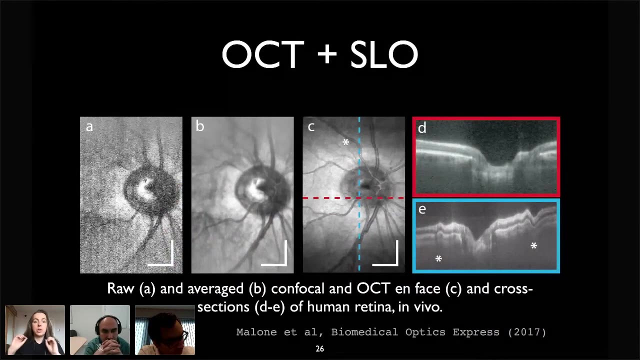 to identify lesion in the oral mucosa, Again using this new fiber dedicated to improving the signal for confocal images, And another group. so we work with collaborators around the world through the lab and also through the company, and it allows us to spread the technology. 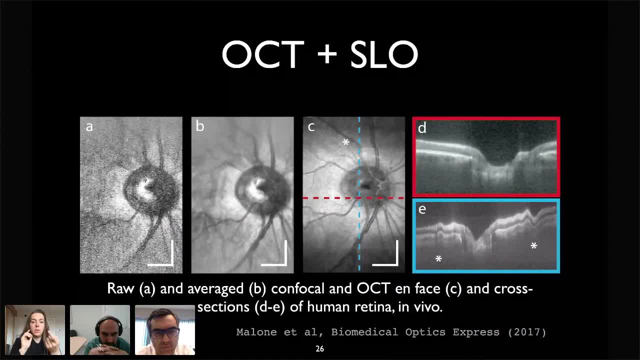 to different applications. This is an image of the fundus, and if you do it with our fiber, you can get both the fundus and the cross section, which is the OCT image. So let's talk about OCT for a moment, because I've been mentioning it a few times. 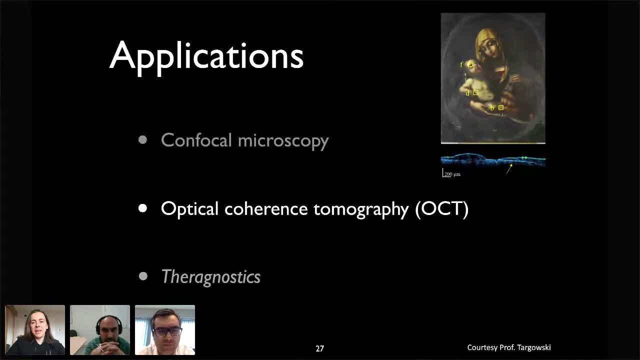 So let's talk about OCT for a moment, because I've been mentioning it a few times. So let's talk about OCT for a moment, because I've been mentioning it a few times. I'm playing with this In my book. I show a piece of art for every chapter. 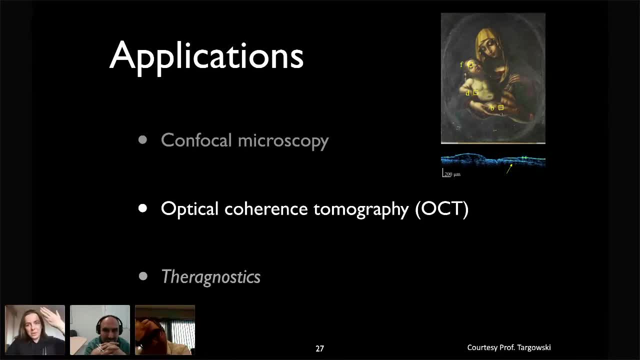 and this one for OCT. OCT is used to acquire non-invasively cross-sectional images, And so here it's used in art restoration to see where varnish's layers need to be restored on paintings. It was done on a minor painting. 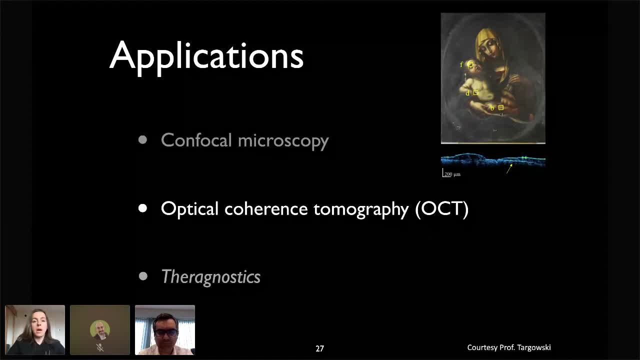 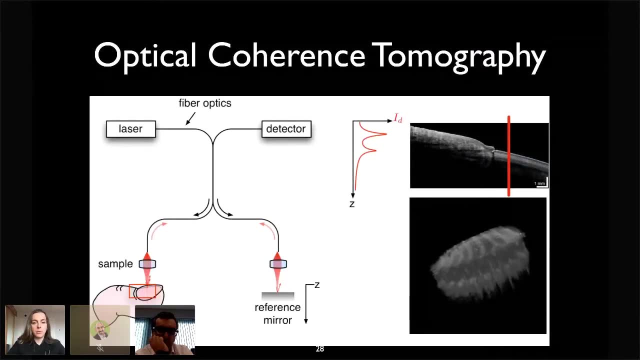 but now OCT is being done at the Heis Museum on Rembrandt and on Vermeer. So how does OCT work? Essentially, it's a new name for a Michelson interferometer, So as opposed to have the standard Michelson interferometer, 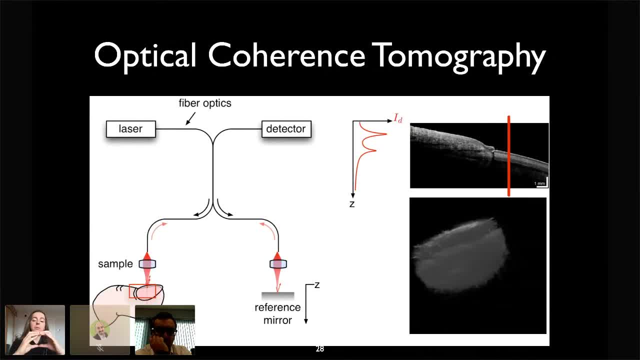 that you've seen in CEGEP or in college. as opposed to use a free space beam splitter to send your beam into a reference and a sample arm and a reference arm, we're actually going to use a fiber optics beam splitter working exactly the same way. 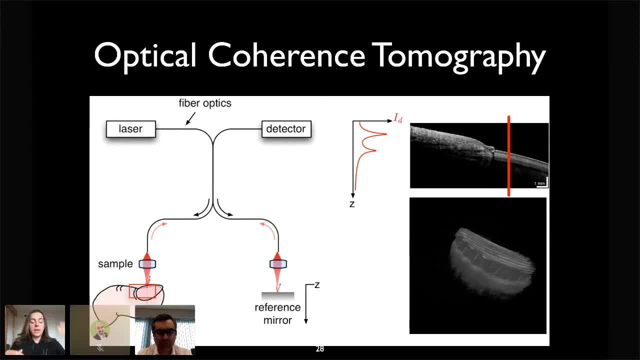 So from the laser you split your signal in two: One that goes to a sample- let's say my finger for now- and one goes to a reference mirror. And by comparing lights going inside your finger and on the mirror, you can get interference. 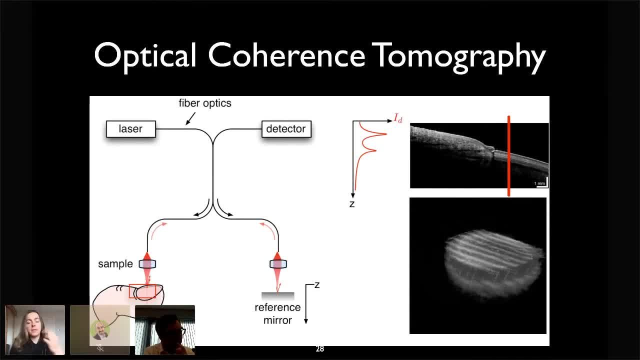 and have sectioning, virtual sectioning of, especially if it's my finger. I'm going to insist that it's virtual sectioning of my finger, And so the images that you get are essentially different cell layers in depth, up to one. So if I were to turn my finger around, 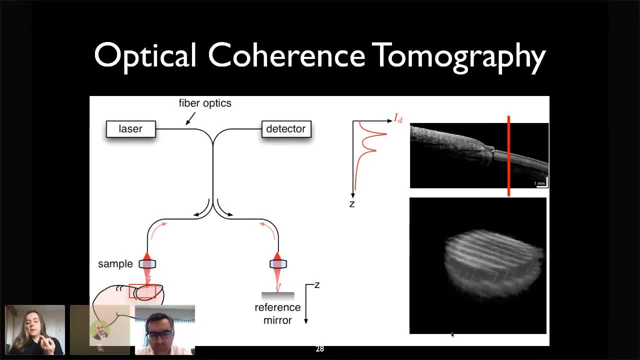 I would. ideally a movie would be playing. there we go. So you actually see the ridges of my fingerprint and the little corkscrew structures are sweat glands going from the dermis through the epidermis and eventually out into the open. 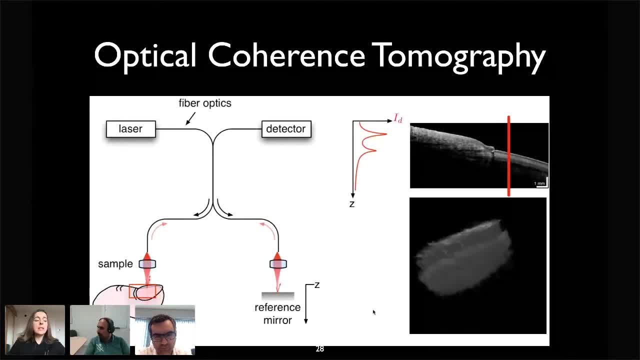 So this is OCT And because we're working with the face, OCT must be in the same phase as the face. So if you're in the same phase as the face, OCT must be used with a single-mode fiber. But the problem is that very few photons contribute to the OCT signal. 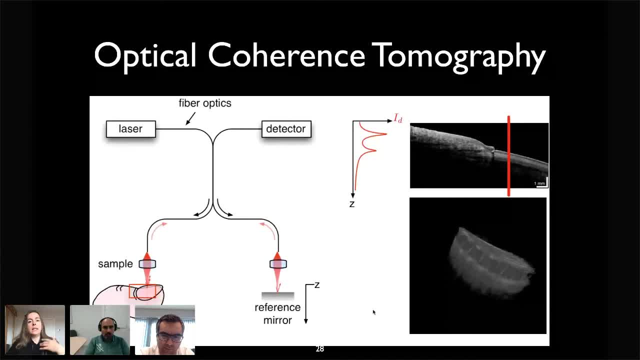 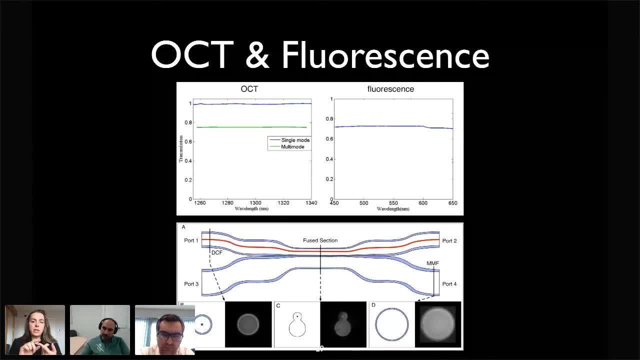 Everything else is lost by this gating or this sectioning, And those photons do carry information. You can use these photons to reconstruct some autofluorescence or even spectroscopy signal, And this is where our coupler again comes into play. 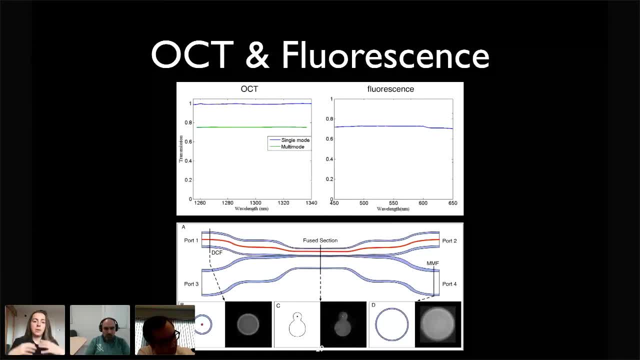 And again we're redesigning the coupler for every application. So in this coupler, we're redesigning the coupler for every application. So in this coupler, we're redesigning the coupler for every application. The red line, the core, is used for OCT. 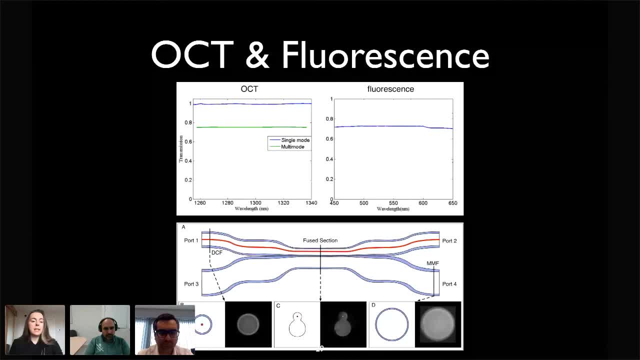 So OCT from 1 to 2 and 2 to 1 losslessly. that's the line that shows like 100% OCT signal in blue. But we can also now gather autofluorescence from the inner cladding at port 2 and collect it at port 3.. 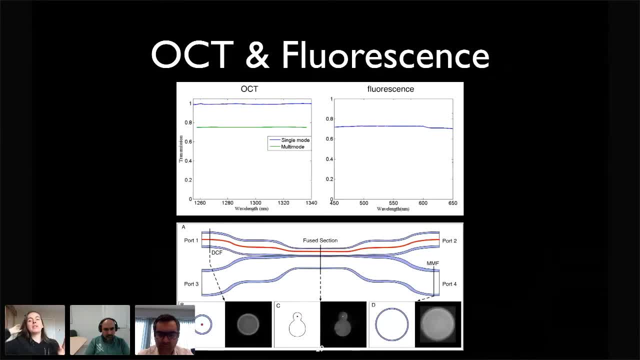 And we used to be very excited to have like 75% transmission, but now we're more around 80-85, so we can collect a whole bunch of photons And because the area is much greater, you get up to 100 times more signal in fluorescence. so this is what it allows you to. 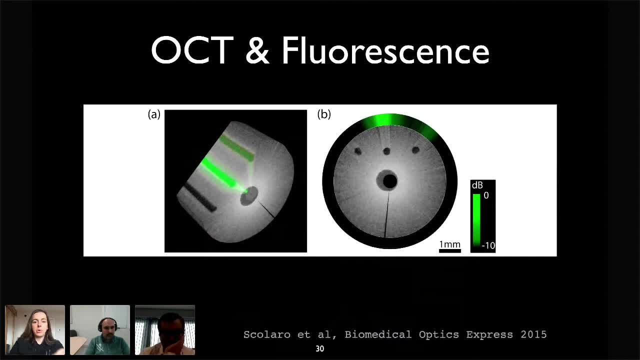 do you get an oct image? so this was done in collaboration with the group of david samson and robert mclaughlin, then in perth in australia. so that was a good way to test whether or not we can ship our couplers and they would work through shipping and i- actually we- we did two things. i. 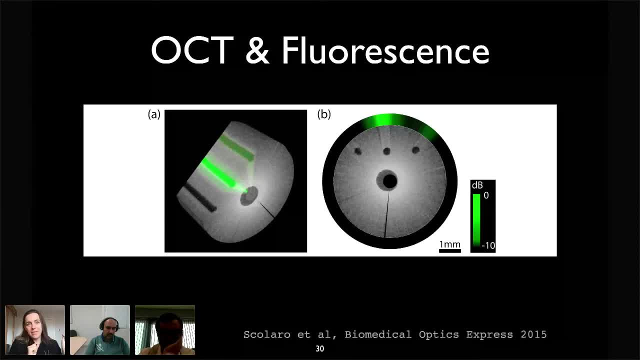 shipped a coupler and i took one in my luggage. so we we tried having the couplers shipped through regular um delivery and also myself bringing a coupler um. so their group is doing oct through a needle, so they essentially make a cylindrical phantom and then they poke a hole inside the 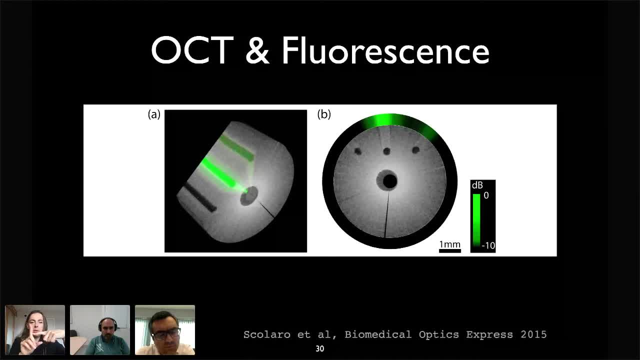 phantom and their, their needle acquires oct images at 90 degrees and as you turn the needle you can get cylindrical information also oct was great to tell you that there were three channels in this phantom and then with our fiber, we can tell that there's, in addition, some in the channels: autofluorescence- uh, a channel was just 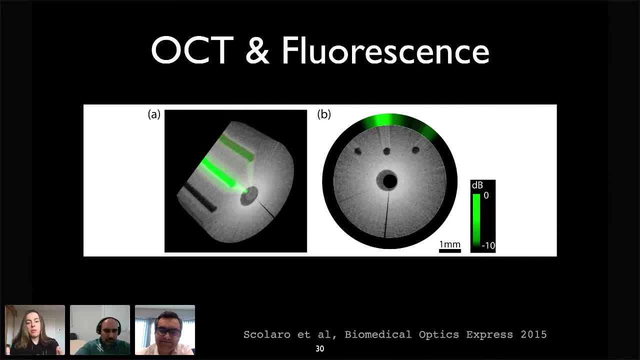 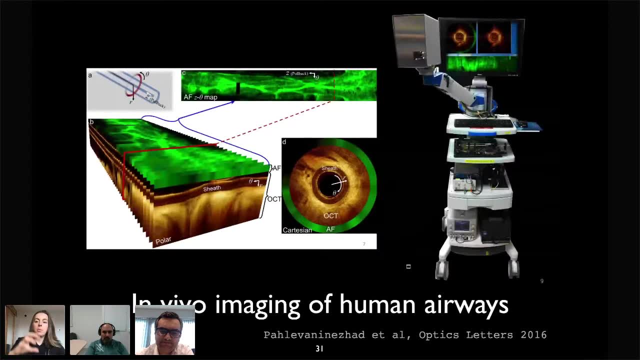 with water. one with high concentration, low concentration. proof of principle: in 2015- 2016, a group in bc cancer agency worked with us to integrate our coupler to their oct system within an uh an in vivo probe that was sent to um the human airways. 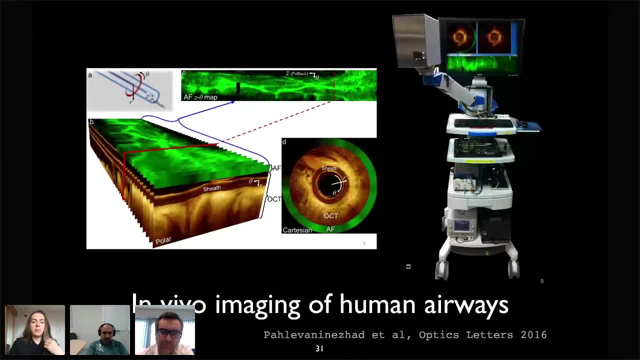 in vivo imaging showing the autofluorescence from the extracellular matrix. and so essentially we can, once we acquire the oct signal and we unfold and make a map. we can make a map of the blood vessels following um that are, that are adjacent essentially to the airways and what this group is. 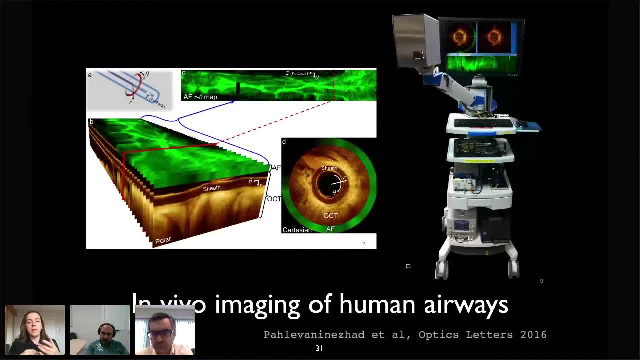 also showing is a destruction of the extracellular matrix from neoplasias and dysplasias, and so this could become a natural. this is a natural system for a group to be able to make a map of their cell. This is autofluorescence. 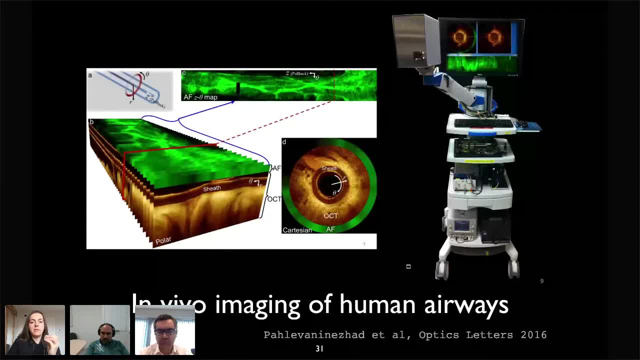 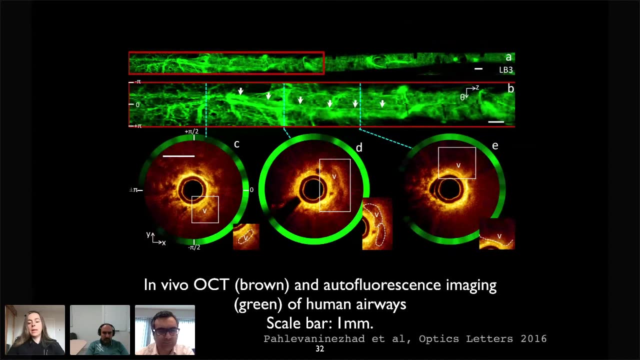 There's nothing injected to the patient. The patient is also not genetically modified to fluoresce. It's pure autofluorescence intrinsic to the human body And that could potentially become a marker for cancerous lesions, And this is what this group has shown here. 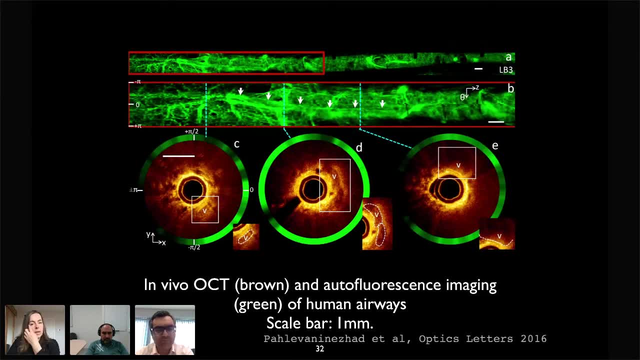 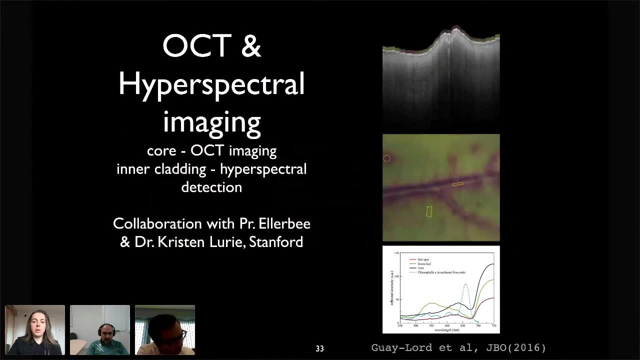 And I encourage you to go read their papers. It's really excellent research. Back in Montreal, we're also showing new applications for this coupler- Again OCT- but this time where we ask ourselves: can we, in addition to have the depth information with OCT? 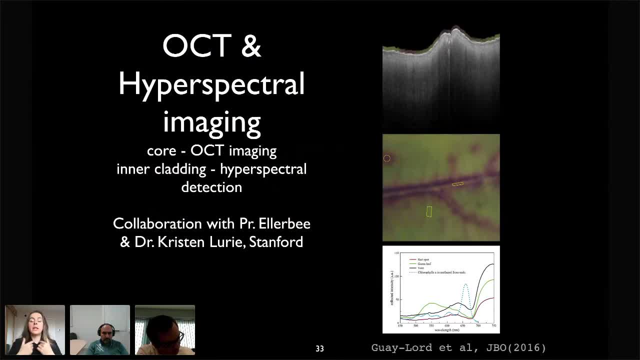 show the color, Because most clinicians have been trained with the color an entire life, right? So with the different shades of red, they can tell inflammation. different shades of yellow and green, they can tell infection. So we started with a plant in my office. 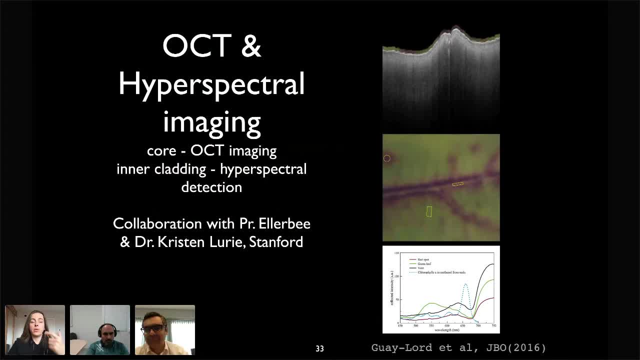 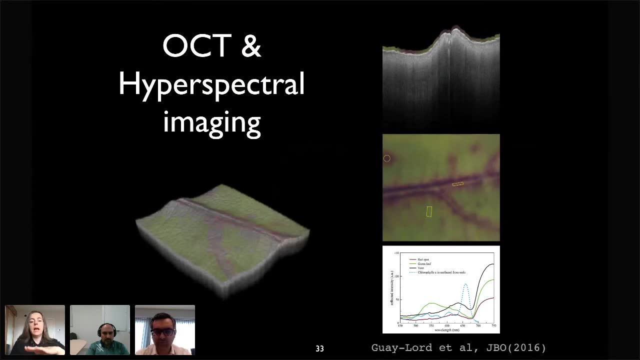 The plant is now dead because we kept trying with different leaves. But essentially we're doing OCT through the core and hyperspectral imaging that we can reconstruct whichever way we want. We decide to reconstruct it with color And by combining the two you get the high resolution, depth information from OCT. 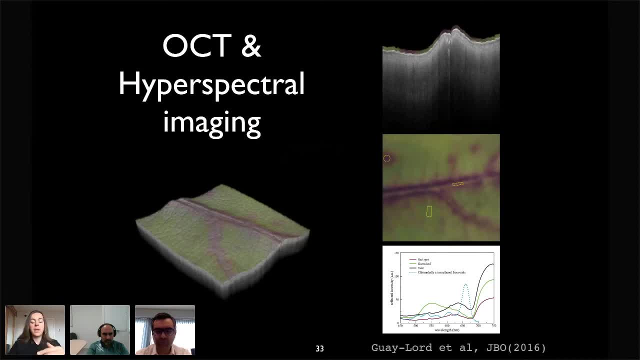 and you get the color information from the inner padding And we can reconstruct it with RGB. so true color, but we can reconstruct, once we have the hyperspectral cube, whichever way we want. So for skin imaging, for example, we can look for inflammation just by the color. 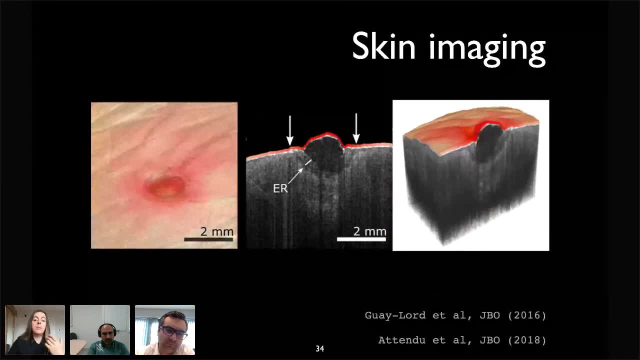 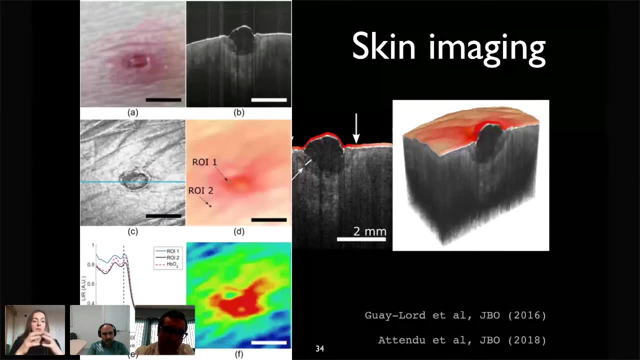 the white color that the surgeon is used to seeing, and also use the spectrum from oxygenated versus deoxygenated data and then provide a map that tells the oxygenation or tells if there's other markers, So by the hyperspectral imaging. 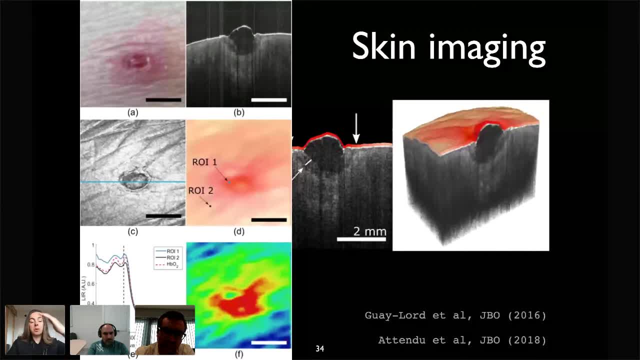 we can reconstruct the image whichever way we want and superimpose this spectroscopic information to the OCT depth imaging, showing here very simple example where you see the epithelium being regenerated under the scab. but it can show anything really. And the very last segment that I would like to address: 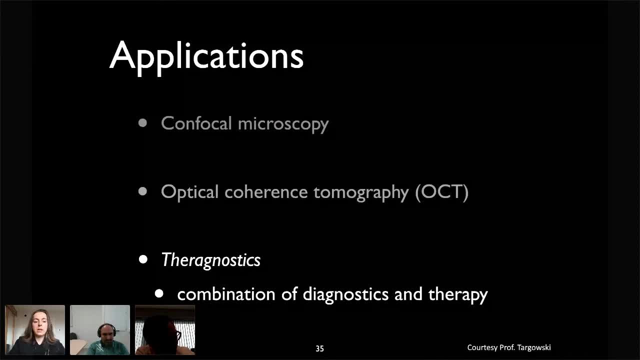 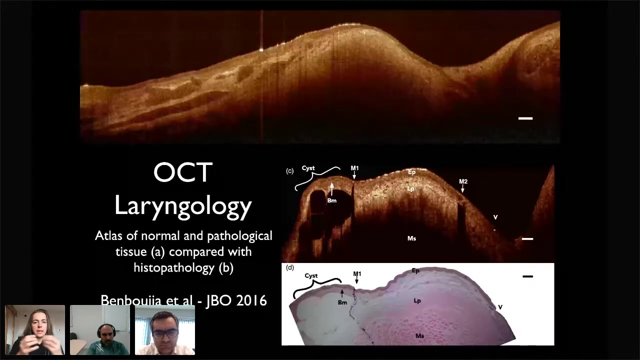 I still have about 15 minutes, so this is good- is not only doing diagnostics or imaging, but also see can we do new devices to help the therapy during, while doing this in the diagnostics. So this is again inspired by our clinical translation. 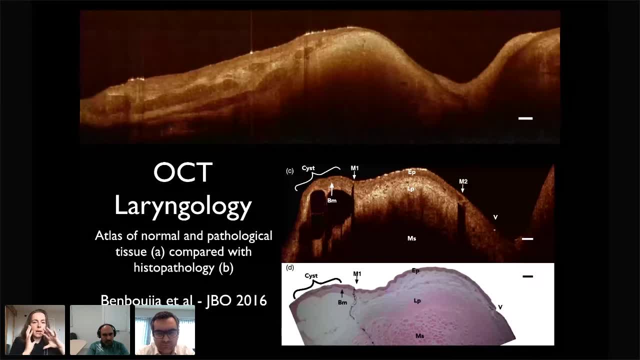 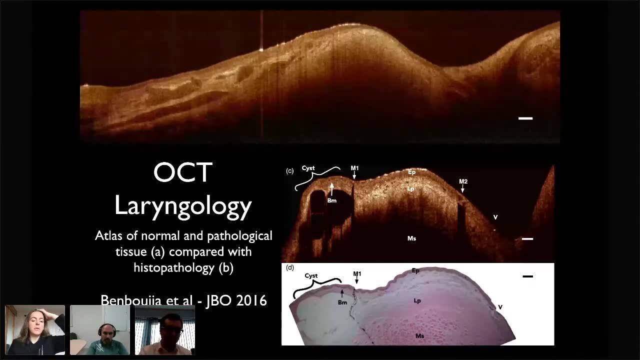 So one of the great aspects of our lab is going to the clinics with OCT and learning from that, And this is the work of my first student, Fouzi Benbouja, who's now instructor at Harvard. So we're doing this in collaboration. 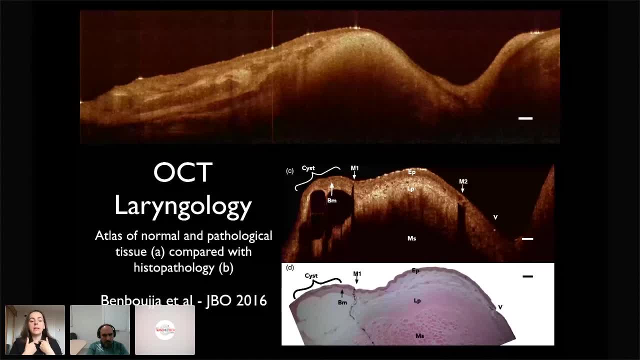 with the Massachusetts Eye and Ear where he's using OCT in laryngology to look at normal and pathological vocal folds. On the top you have a normal vocal fold with the layered structure, the glandular appearance, the normal and false vocal fold. 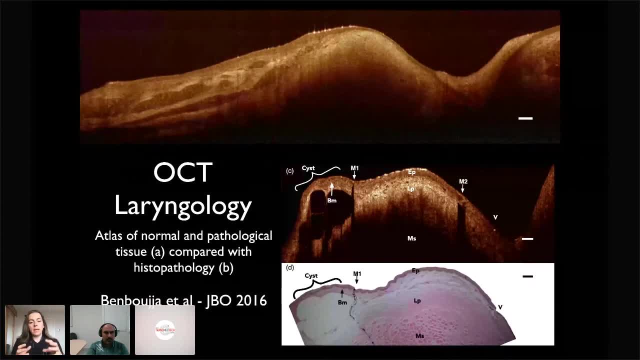 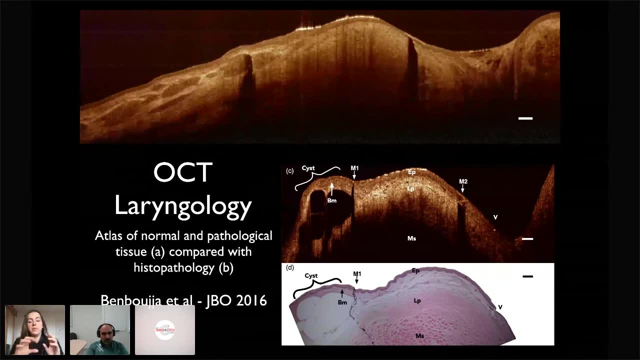 And in the bottom you have a cyst. And this is truly important here, because OCT is the first technology to show you the cross-section of the cyst non-invasively. Here it was a really rare case that the cyst was also biopsied. 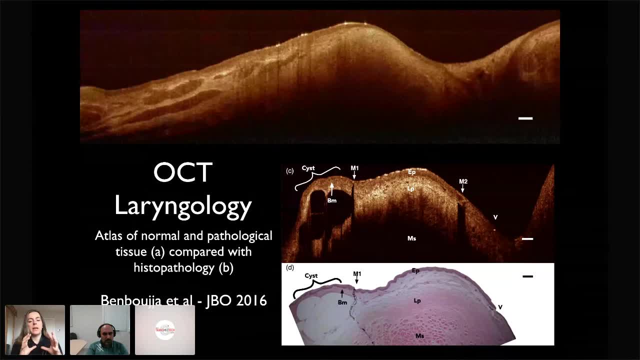 Typically you don't biopsy the vocal folds except in really rare cases. But here the cyst was biopsied and it allows us to show that OCT and histology have a really, really great correlation. You see the different structure. 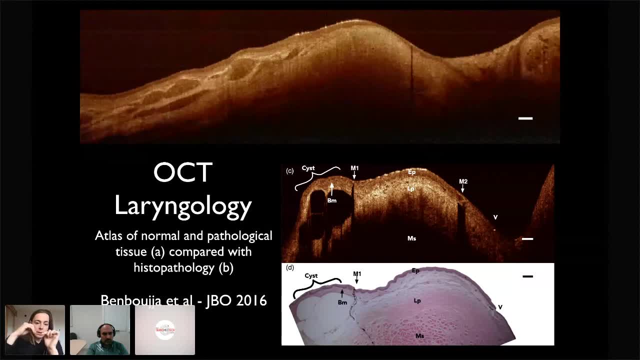 You even see the membranes between the different cyst structures. So it's not to the level of confocal microscopy but it gives you a layered structure and have a very good idea. The differentiation between normal and pathological is great. Of course, bringing color to that is one avenue. 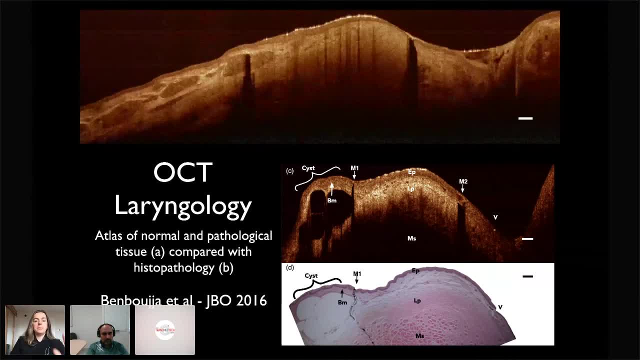 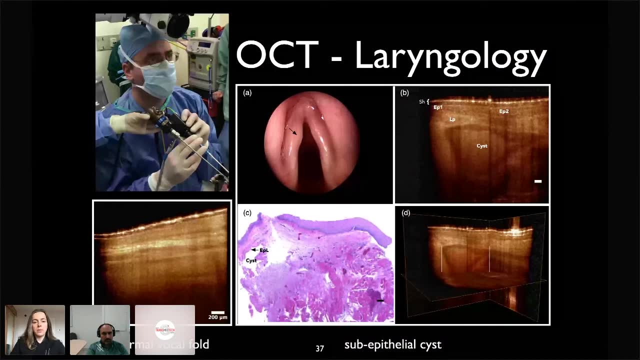 But another avenue is: what do you do once you diagnose a pathology? And again I want to stress the importance of OCT. In A you have the endoscopic vision of the vocal folds and the arrow points at a bump, And the current way to diagnose is essentially: 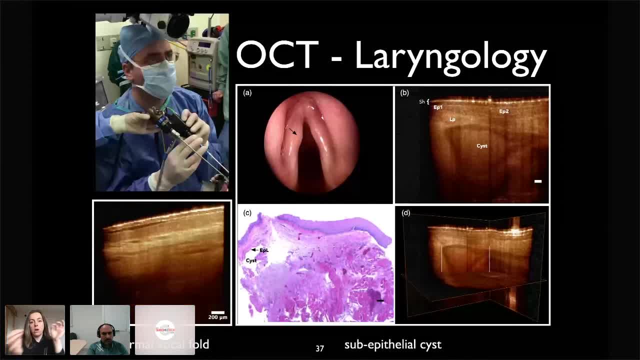 to sort of touch it with a long device and try through mechanical properties, trying to assess: is this as stiff as it is? Right, Yeah, Yeah, It's not as stiff as a nodule or a cyst And you have no idea what kind of cyst or nodule or even tumor. 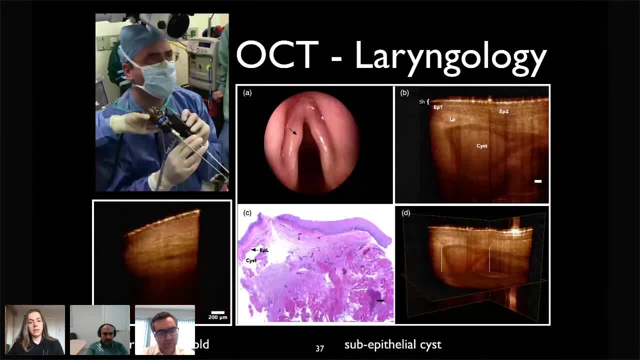 it is, And I'll show you some pathologies- I have a much more gross appearance- that are pretty obvious. But for a simple cyst like this, is this a nodule? Is this a cyst? How deep is it? It's very hard to tell just by touching it. 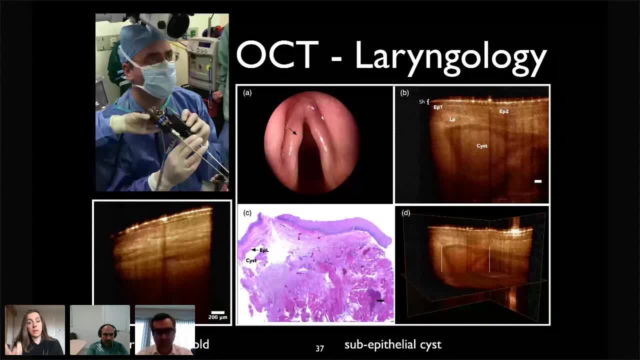 OCT shows you the type of cyst. Is it full? What is it filled with, Especially if we bring the spectroscopic data? And also, how deep is it? How much of the lamina propria can you preserve? In other words, how much of the voice? 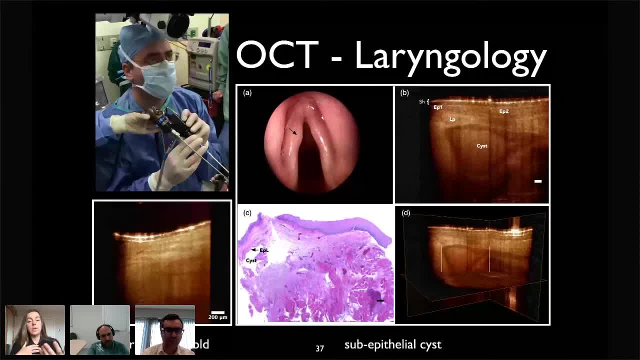 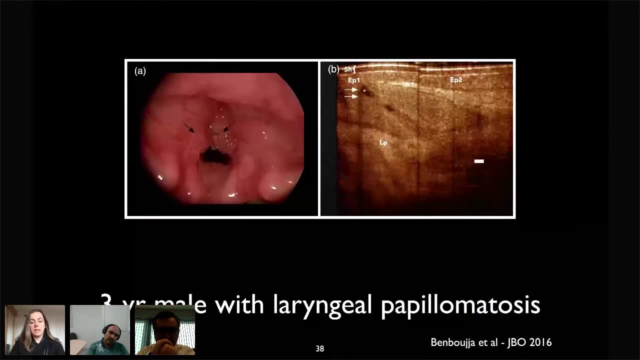 can you preserve by operating on it, So it can give you a prognosis for the therapy. But more than that, there are other lesions that are even more aggressive than a cyst, And this is the papillomatosis. It's the result of a viral infection on the vocal folds. 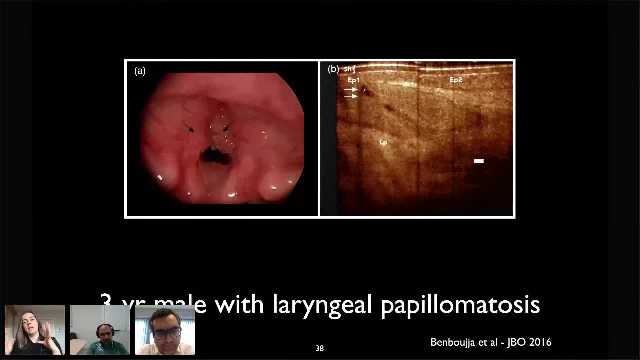 It's essentially a wart. So in my very uneducated engineering point of view, this is like a wart growing in the vocal folds very rapidly And what happens is that it increases, increases, increases the thickness of the vocal folds, closing the lumen. 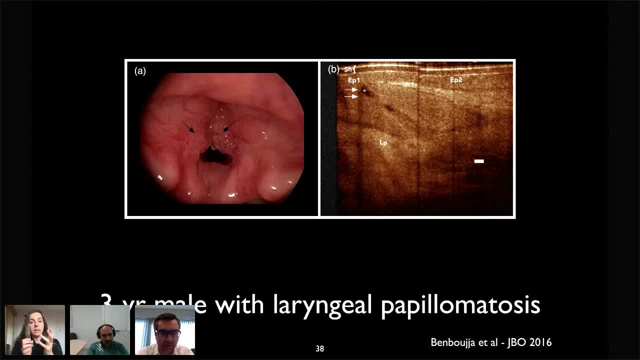 Unfortunately, the lumen here is the airways, So if you let it grow, grow, grow, grow, grow, you don't have any room to breathe, And this is, as I know as an engineer at least, very incompatible with life. 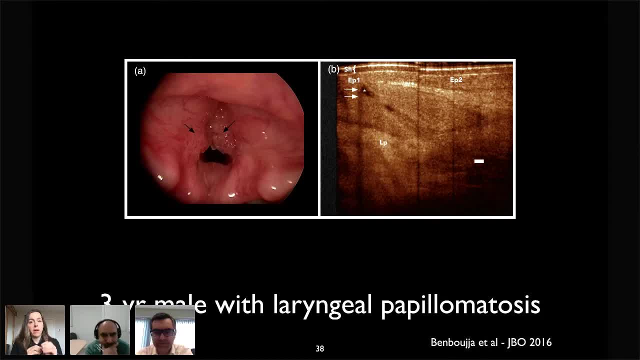 So if you suffer from this terrible, terrible viral infection, you have recurring warts on your vocal folds, closing your airways, And every several months you have to go to get a surgery, get it removed so you can breathe again And eventually we're also trying to preserve your voice. 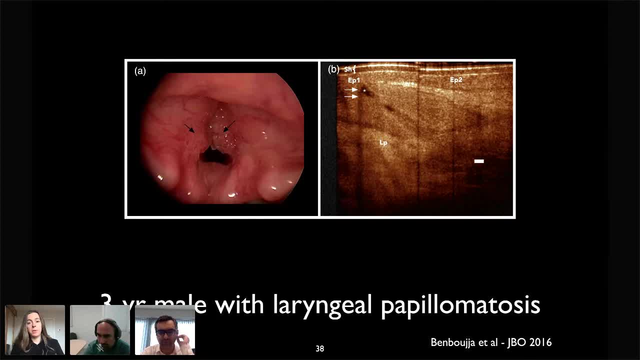 But in terms of the Maslow pyramid of, you know of human functions- breathing and then the voice- So we're trying to do both. So what my student Fousey is doing with Dr Hartnig is trying to look at OCT to, of course, 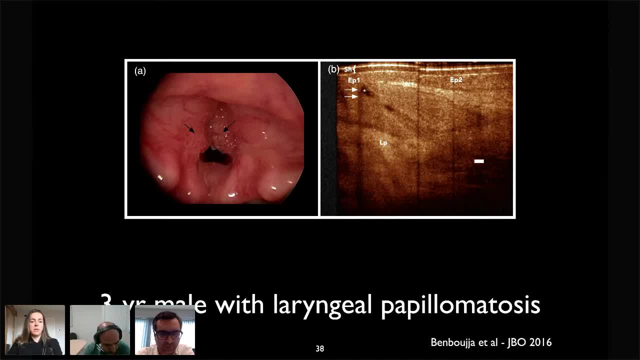 you don't need OCT to diagnose the papillomatosis. I think everyone notices that there's something wrong here, So that's good. But at least how deep is it? And can we use OCT during the treatment to assess the depth of the treatment? 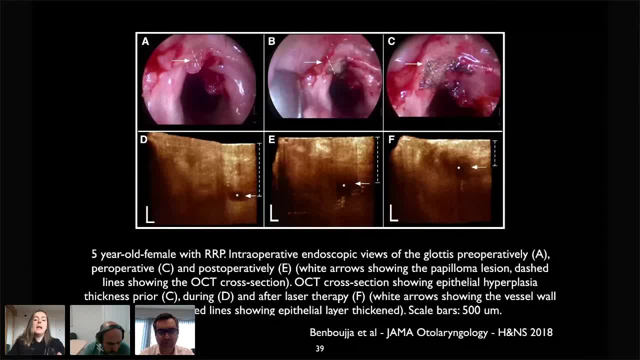 and to stop the treatment once we reach critical areas. And this is a great first step, right? So you go with your laser probe, you remove it, and then you go with your OCT probe and you try to image the same area, because the field of view is very small. 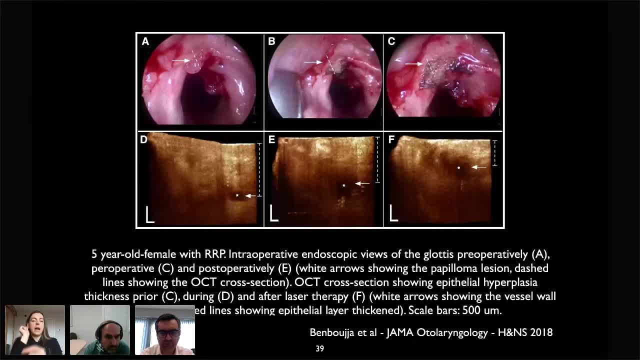 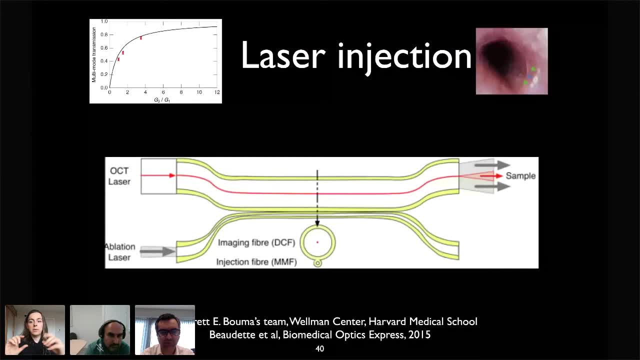 And then you remove it and you do laser again, And so this is not the ideal way to do it. And so you guys see where I'm going with this. We've flipped our coupler around As opposed to extract light to have more imaging. 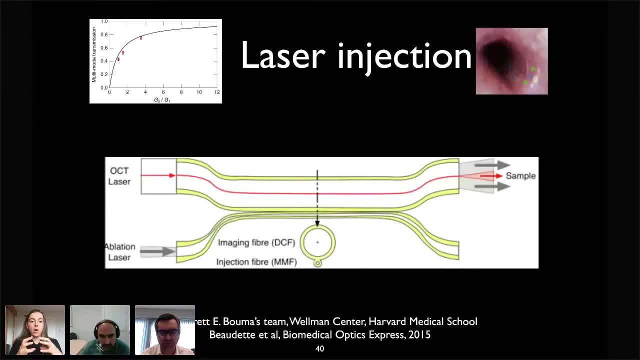 we want to send light in, to be able to have OCT-monitored laser ablation, And this cannot be done in a snap. This is not just wishful thinking, though. We're working on it, but we're working step by step. 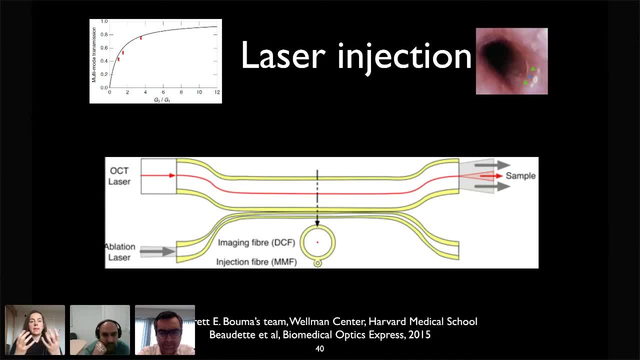 And if you look at the laser interaction with skin, think of the egg. Like when you put an egg in the pan, first you have it heats, then you have coagulation right. Your egg white turns white. right, It was transparent, then it coagulates and turns white. 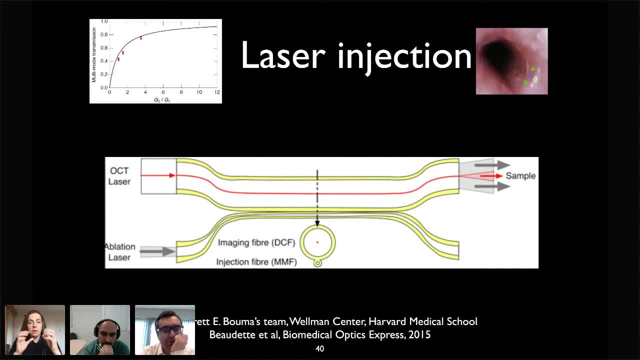 And eventually, if you leave it there for too much, you get all the vapor out. So you have vaporization, And if you do it very quickly, you have carbonization. This turns black. So you have all these steps and we're trying to gauge this. 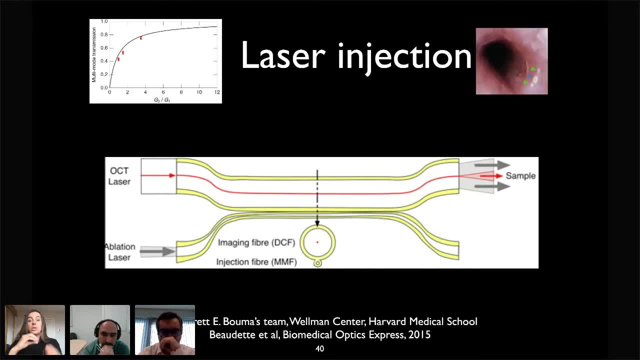 And we're also doing that- not, of course, carbonizing the coupler. So we need to come up with new fibers, new geometries, such that we can reach exactly the right level of ablation without carbonizing and without going too deep. 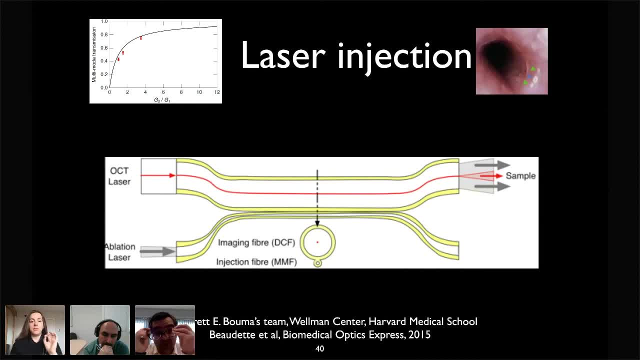 and without also breaking the coupler. So our first step that I gave to a second PhD student, Cathy Beaudet, was to ask her: can you reach coagulation? Nothing else, just coagulation. So she did the math. 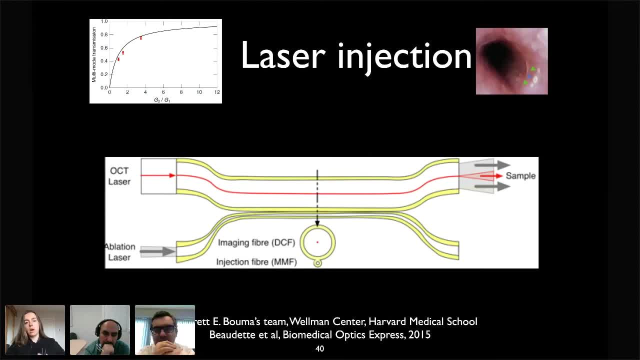 the modeling. She had a dynamic Monte Carlo because, as it turns out, as you're doing your laser treatment, you're also changing the optical properties. So it's a simulation that dynamically changes in time as you apply the treatment. But she managed to show. 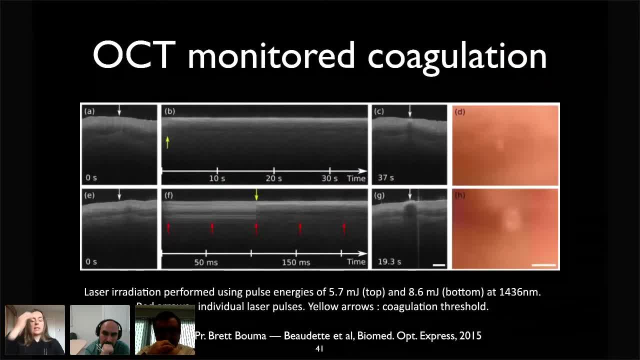 and to predict when she can reach coagulation. So she's done imaging here on the. So she first created the coupler that did not exist a priori and used on, showed it on excised porcine esophagus. So in A you have the OCT image. 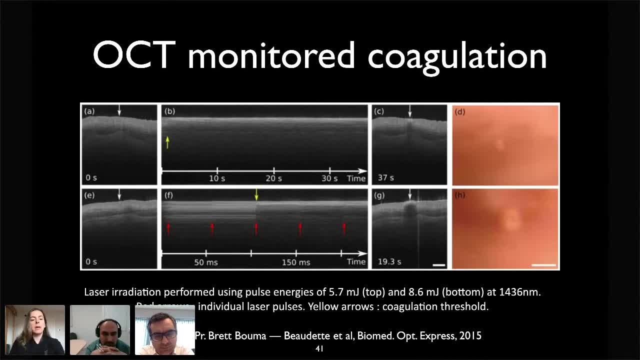 and then the, the parenchyma of the esophagus, And then, at the white arrow, she stops her image so that it becomes an M mode and she's pulsing her laser to see when coagulation occurs, Depending on the energy of her laser. 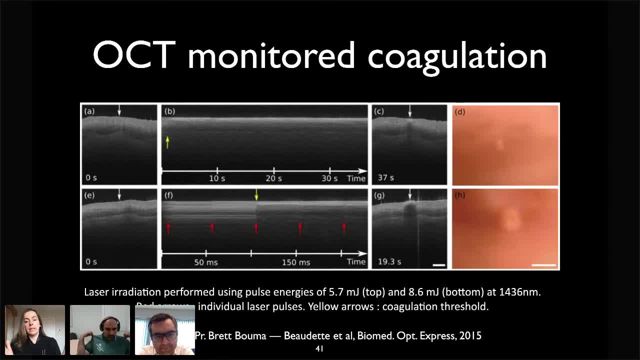 coagulation takes 30 seconds or can happen in as fast as 16 milliseconds, And coagulation is actually seen in OCT because as the tissue coagulates it increases massively. so you see the white arrow where the coagulation spots occurred in the OCT image. 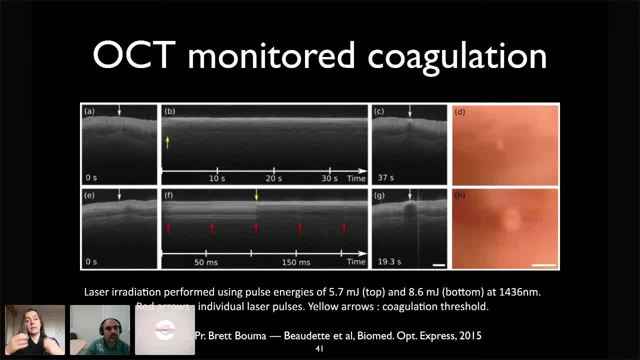 and in D you also see the coagulated spot turning white in the visual, And so now she refined the coupler to be able to have single pulse coagulation. This is what you see here. So again, porcine esophagus on the left. 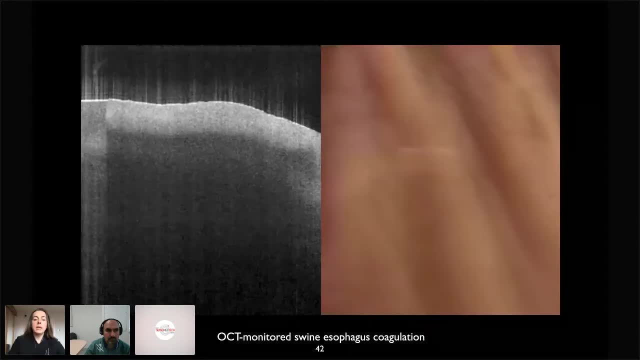 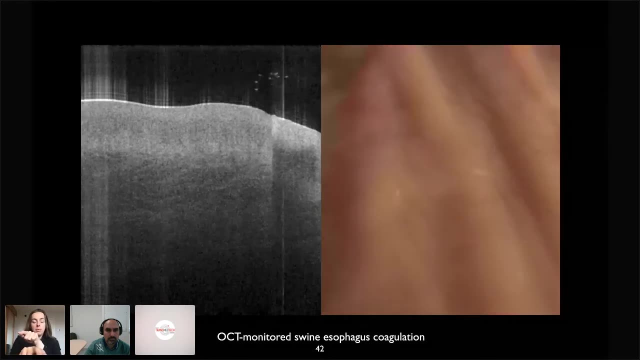 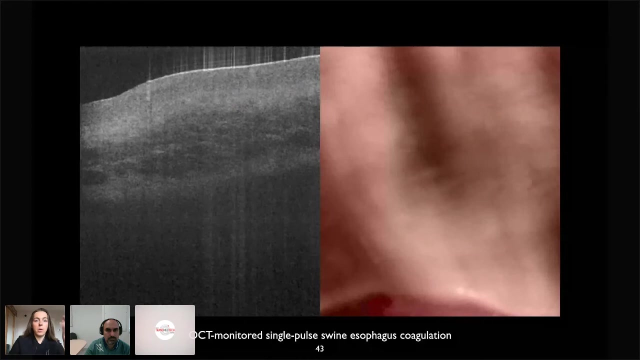 and the visual aspects of the endoscopy on the right And you see that she's essentially we're following the laser trace on the OCT image that produces the coagulation. She also managed to have a dotted line to show that she can do single pulse coagulation. 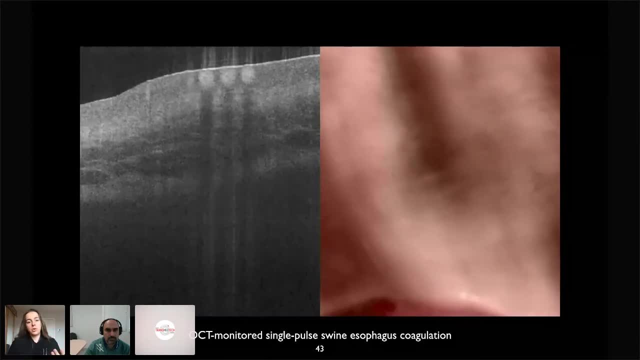 And with other students in my lab. what we're trying to do is have new types of fibers made of new materials, to be able to up the energy, the single pulse energy, to be able to achieve vaporization. But you actually see little water drops here. 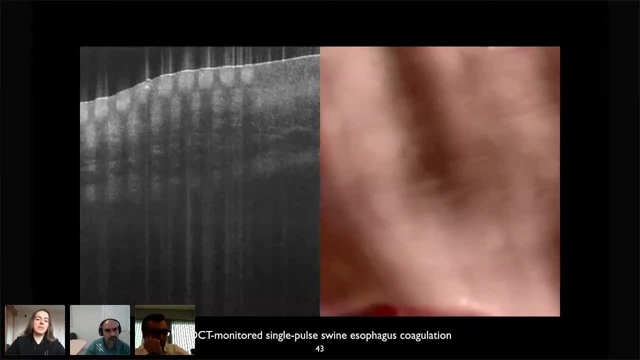 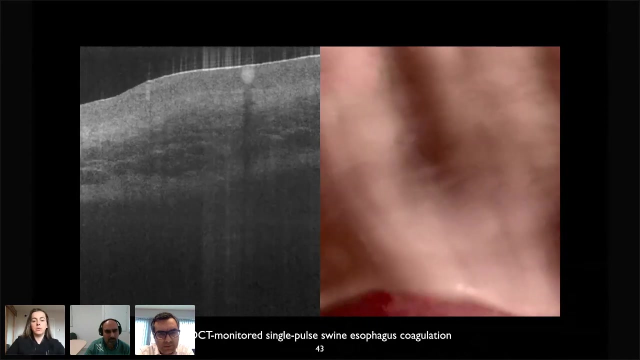 You see the plume. there's a little bit of evaporation that's being done, So we're right at the cusp of being able to do that. This is through new fibers and we have a project supported by Transmedtech supporting who's working on these fibers here. 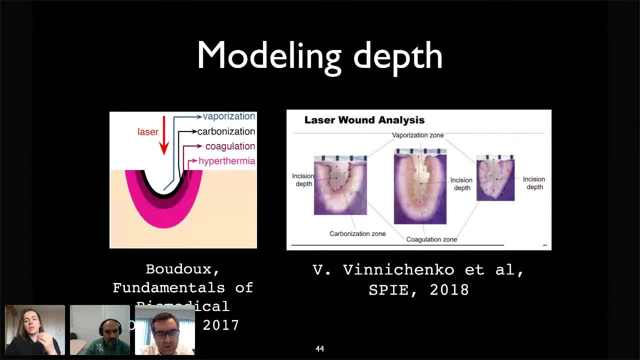 So we're modeling the depth. We're trying to not just go blindly and shoot at stuff with a laser, but to be able to have an absolutely controlled wound depth of wound without carbonization and just being able to ablate very cleanly. And this time we use speckle. 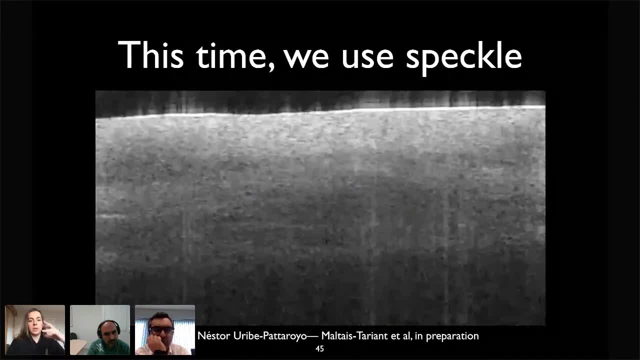 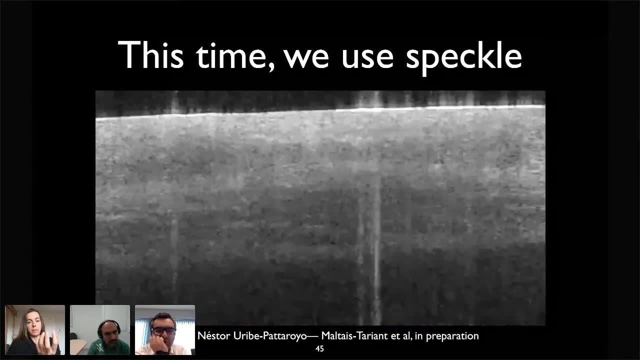 It turns out that the speckle is an indicator of the heat wave, So at first as heat. so the laser heats the tissue. it creates a Brownian motion that will make the speckle move in your image, But eventually as the tissue. 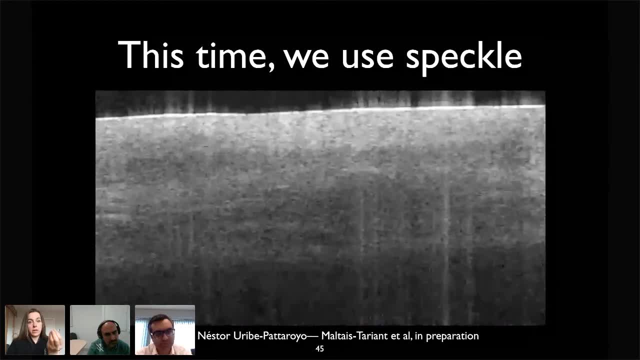 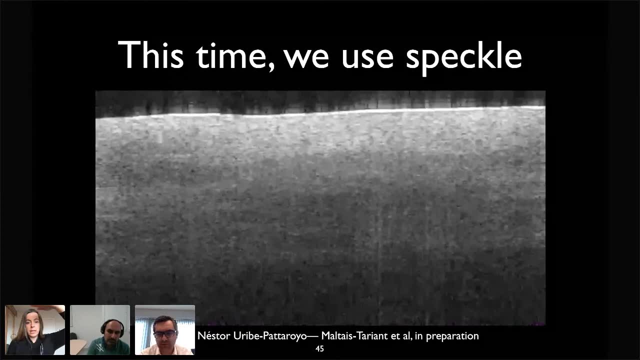 coagulates, the scatterers become fixed, they're stuck in time, and so the speckle doesn't move anymore. And so, if you look at this video, what you see is actually the speckle, So the heat wave propagating down, speckle moving. 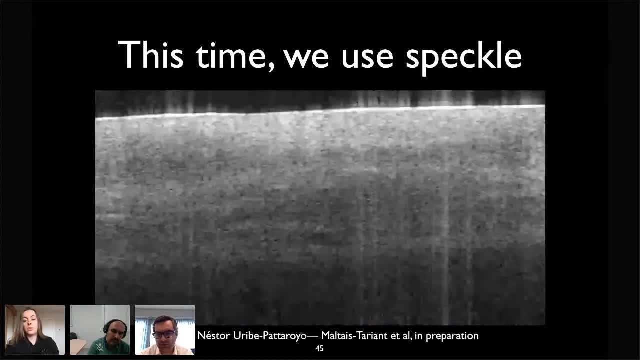 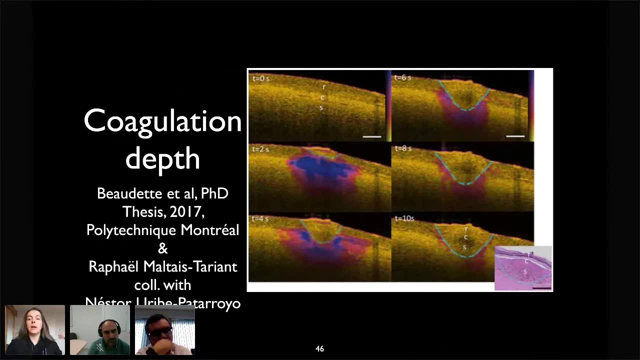 and eventually it stops moving, and this is the depth at which you've reached coagulation. Raphael and Cathy are working on this. Cathy is done now She's actually managing Castor, and Raphael finished his Masters in collaboration with Professor Uribe Pataroyo. 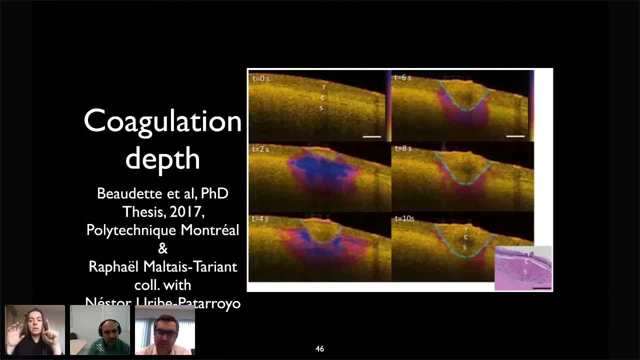 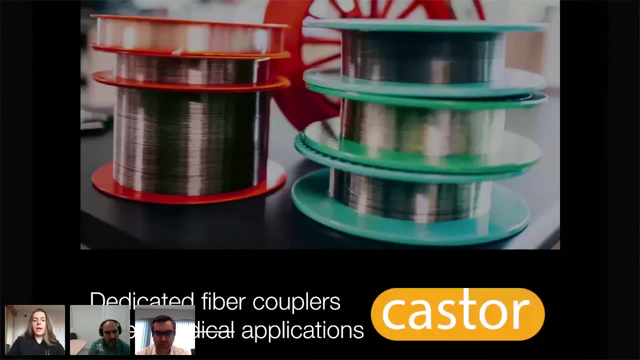 at Harvard Med. But the idea was to show that until the depth, we can essentially predict the depth and have the computer, through the speckle analysis, stop at the appropriate depth. I have three minutes going and I thought I would give you a flavor of entrepreneurship. 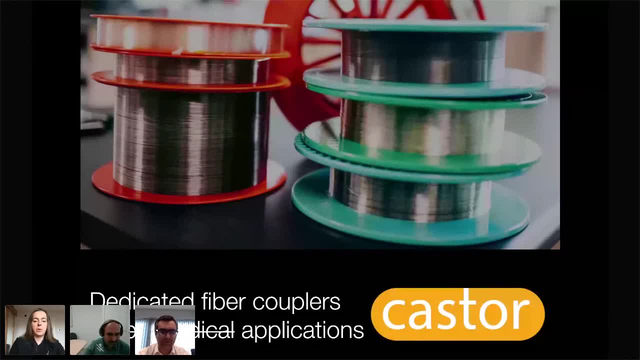 if you allow me to do it in the last three minutes. So in 2013,, I'm an academic through and through. I've never had a job other than being a university or a hospital, So I was always in the lab, never had any entrepreneurship. 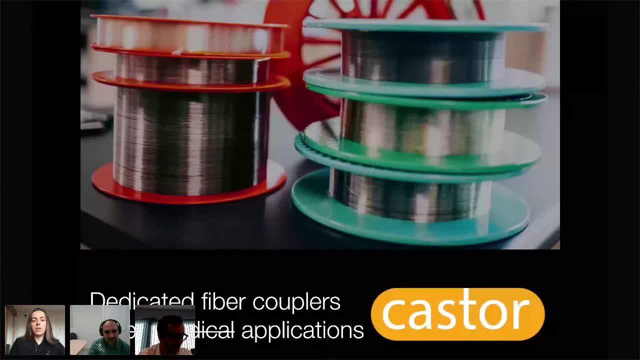 desires or ambitions, But in this case, the technology. once you have something that improves the signal to noise by a factor of 100, you have a moral obligation to send it out, And our goal was to say: let this technology be available to as many groups as possible. 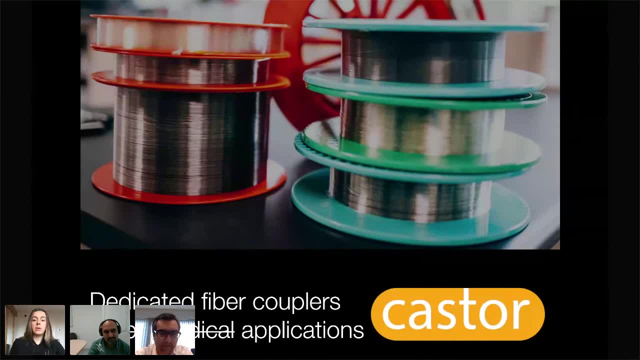 And we spent a year with Univalor, now Excelis, trying to figure out the technology to have the product to the market as fast as possible. We wanted to license or, And eventually it turned out that the market was still to be explored. 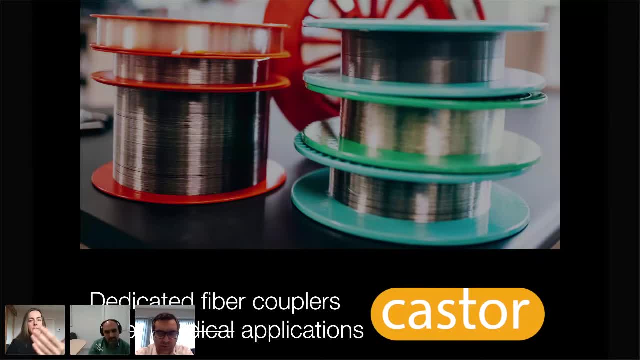 And the companies who had the know-how. very few companies know how to make these products And for them, because they were used to telecom numbers and volumes, the product was a little too niche for them And so inspired by great, great entrepreneurs. 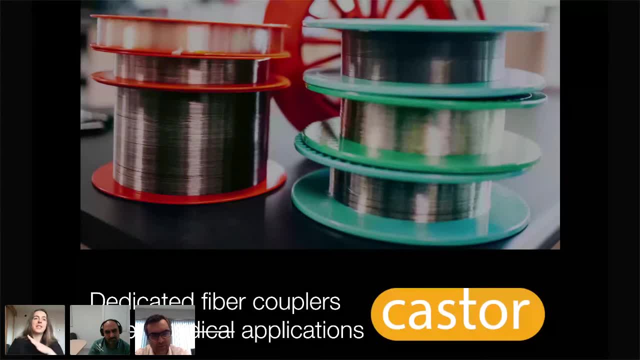 who decided to have money. following their speech, a great entrepreneur said: we'll start this company with you. And it started as a company dedicated fiber optics couplers for biomedical applications. And for once, as opposed to just talk, talk, talk- we also took a moment to listen. 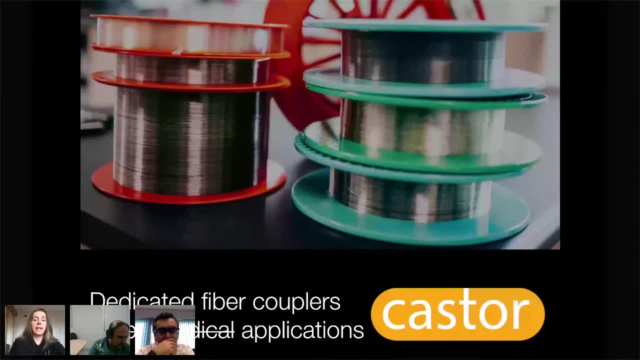 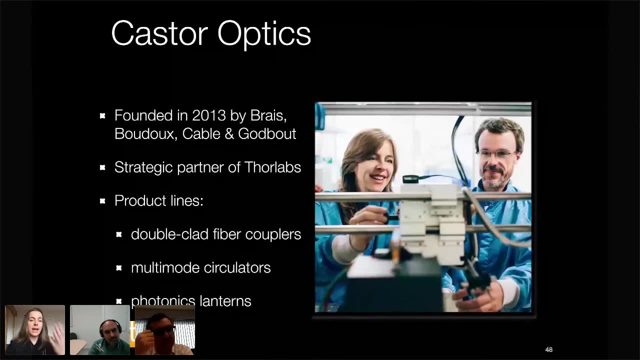 And the market tells us: wow, this coupler can be used for biomed, yes, but also for lidar, also for agronomy, also for all sorts of markets. And this is how Castor was funded, but also Castor evolved. 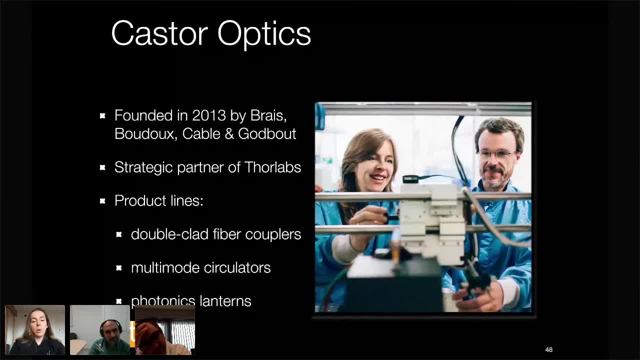 over the last eight years. Founded by Normand Bré. founded and funded by Normand Bré, a serial entrepreneur in Montreal, and Alex Cable, the founder and sole owner of Thorlabs, and founded with my colleague Nicolas Godbout and myself. 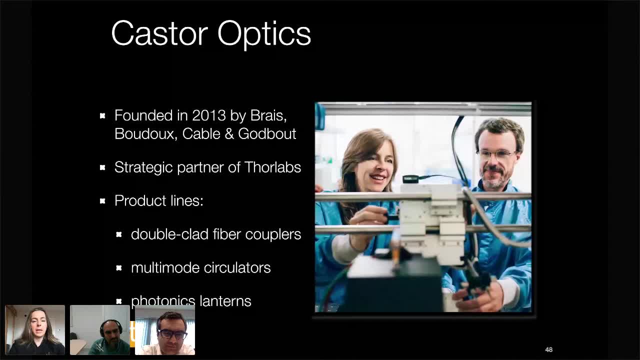 and also Univalleur, so Polytechnique has essentially equity in this company. We're strategic partners of Thorlabs and they were babysat us through the early stages. We can focus, could focus on the technology and they would take care of. 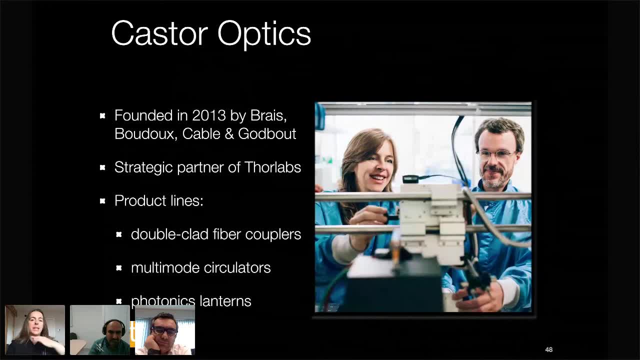 distribution, invoicing, packaging, sending shipping. so it allowed us to just focus on technology and also both of us. we kept our job as a faculty and still have a research group at École Polytechnique, So now we make double cloud fiber couplers. 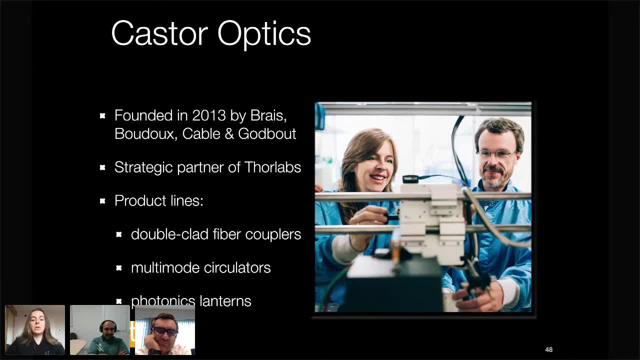 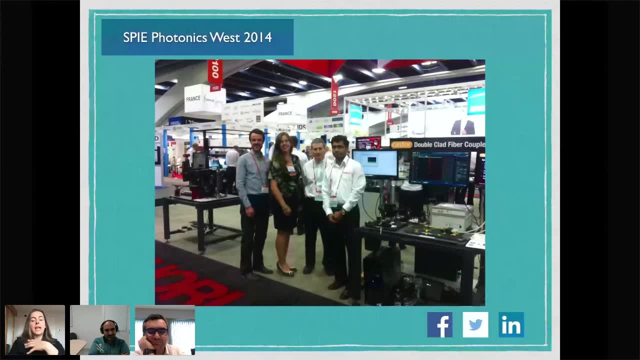 multimode circulators, photonics lanterns, and we're branched out based on the market. So we launched at Photonics West 2014,. we didn't have a product, we had a demo and we were just saying, hey guys, we have this new technology. 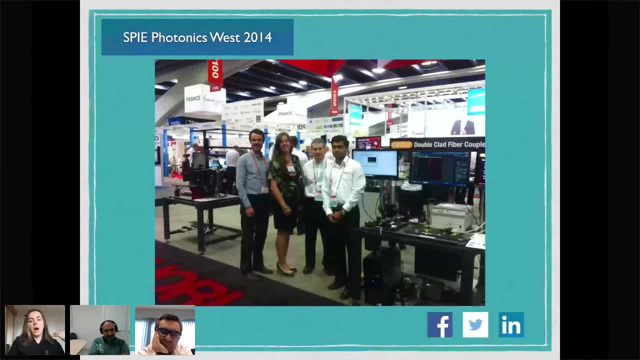 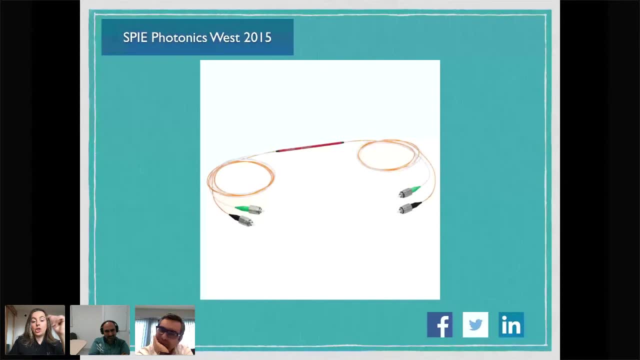 tell us what it's good for. and the next year we launched a product so it looked very good. it went through all the approval of Thorlabs, it was on their catalog and if you look at the date- less than a year later. 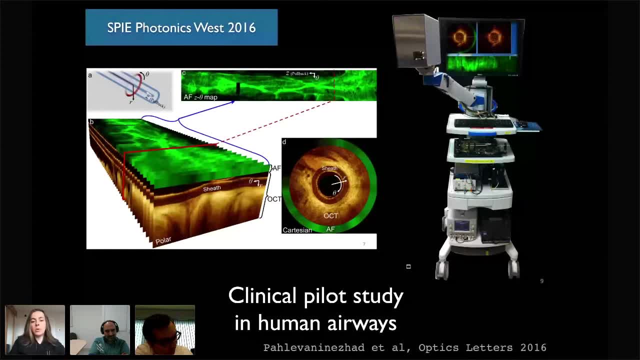 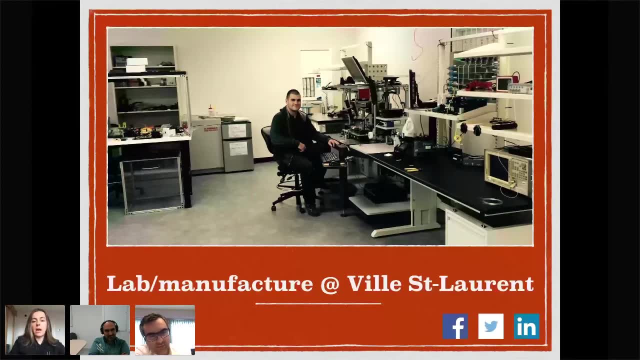 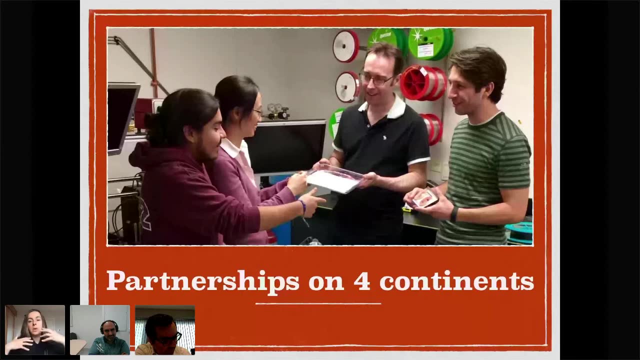 it's detecting a pathology. A few years later, we moved from the incubator at Polytechnique to a lab manufacturer at Ville Saint-Laurent. this is our first employee, now director of operations. We kept partnerships with different labs, different companies to help. 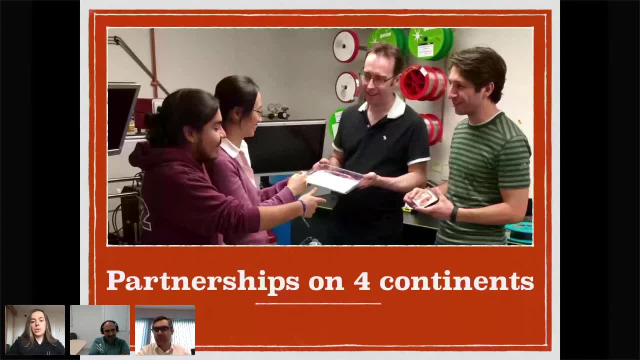 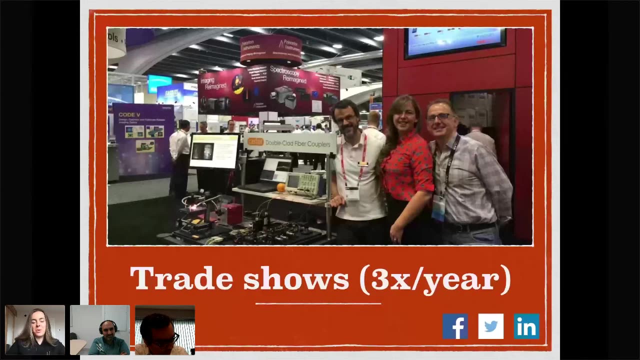 them integrate our products into their solutions and their imaging technologies. Before COVID, we kept going to trade shows. this is Nicolas, myself and Alex Cable, one of the two entrepreneurs who are mentoring us, and we have new products. so we're building it the Russian doll way. 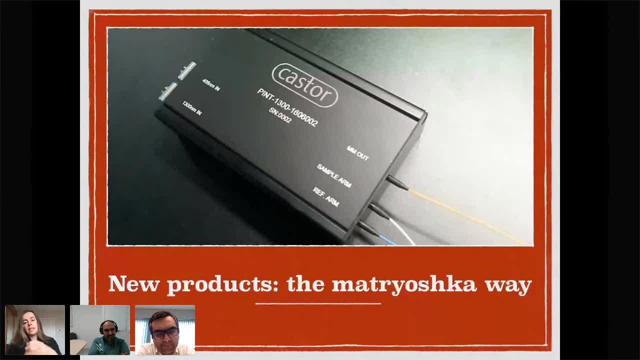 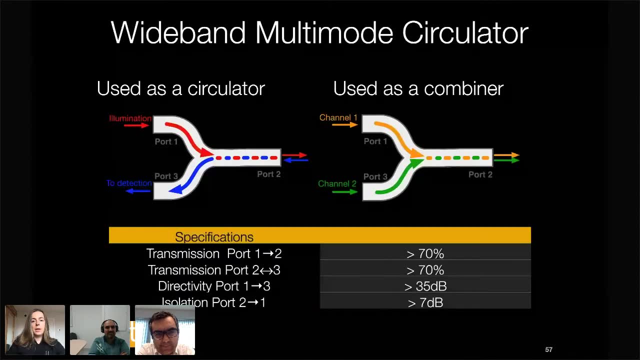 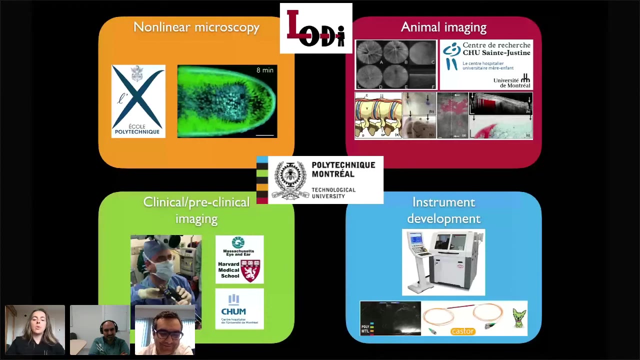 where we have a coupler, we're putting it in the subsystem and then we kept growing the company adding layers on top of the couplers. So, yes, this is an overview of what we do in the lab, what we do at Castor. 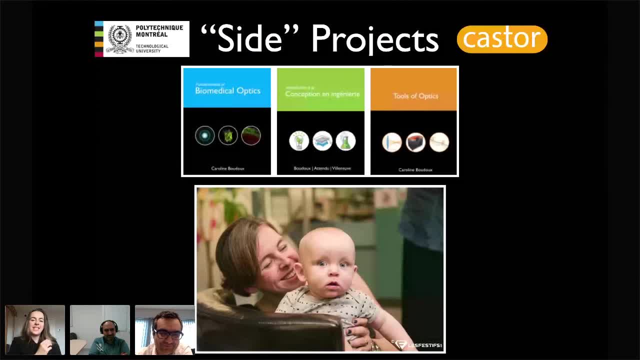 and with that I'd like to end this project with these side projects, the textbooks and my son, who's been very quiet, so I think he needs a hand of applause. I'd like to thank you very much for your attention and for this very kind invitation. 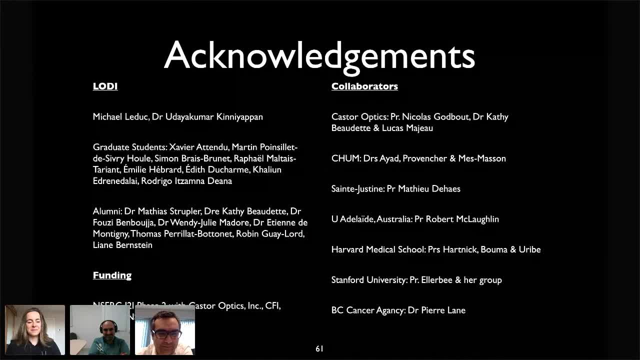 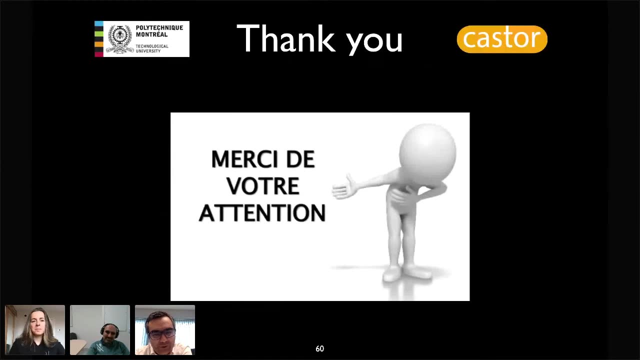 to this e-seminar series. Well, thank you very much, Professor Boudou, for your very nice and very interesting presentation. It took me back to some of the work that we used to do at Harvard Medical School on whispering gallery mode biosensors. 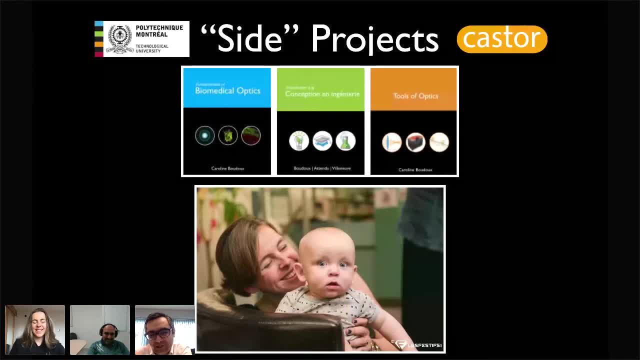 It was a long time ago and I was learning back then how these couplers work and to be honest, I have to confess, it's very difficult. The physics behind it for me is beyond my knowledge and capability, but anyways, it's very, very interesting. 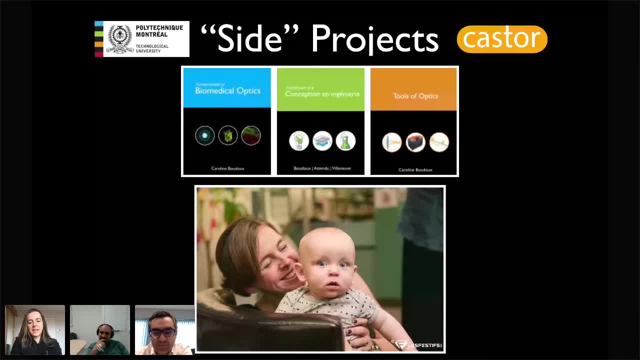 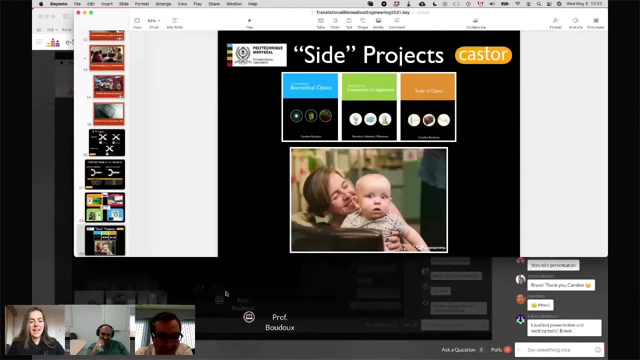 I think the audience are very, very interested in your talk, So we have a couple of questions from the audience. Can I stop sharing my screen so I can see you? Sure, you can, Although I would love to see your son's face. 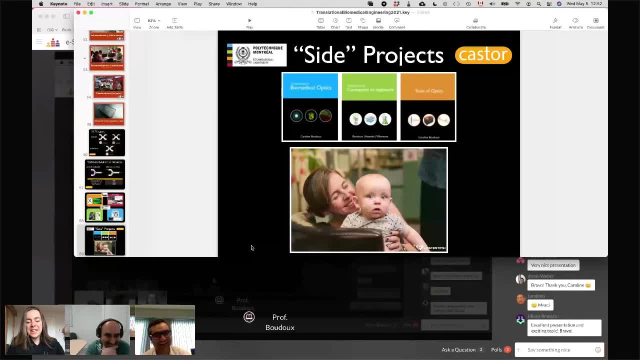 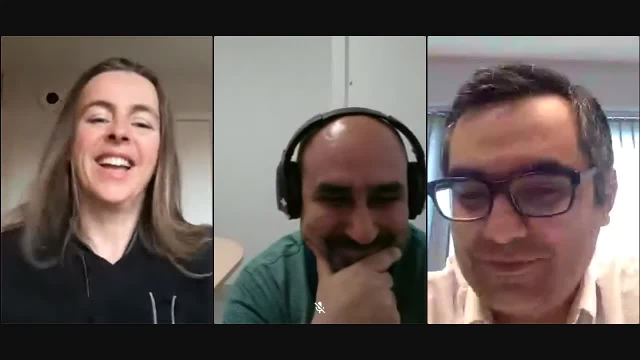 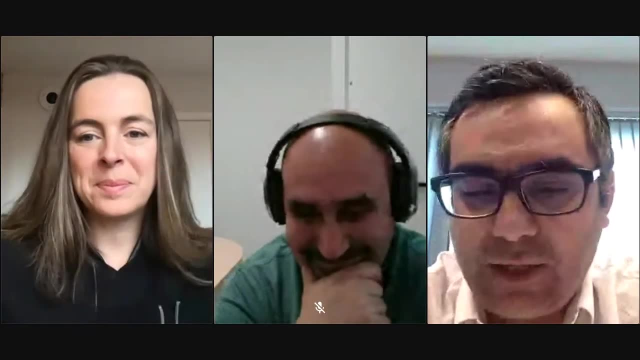 He's very cute. He will come. If I unlock the door he will zoom back in, I know. I know I can give a talk, so I usually hide in one of the rooms. So we have a few questions from the audience. 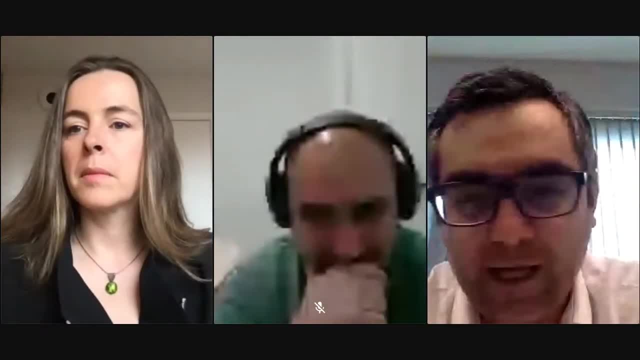 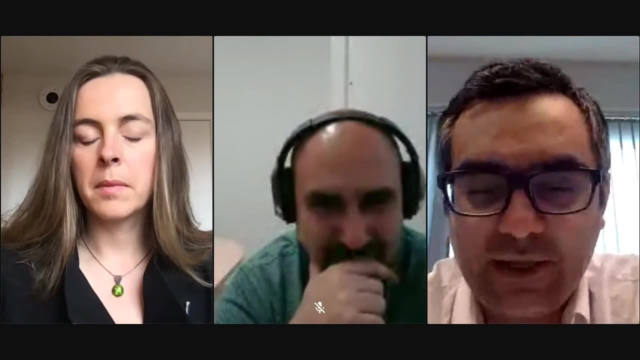 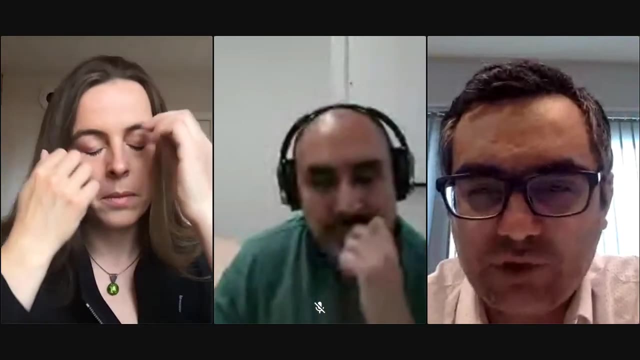 I have a number of questions as well, if time allows, But we'll start with Mike Callas from the University of Calgary. He is asking about the field of view at the end of the fibers. He's also interested in the time it takes to acquire. 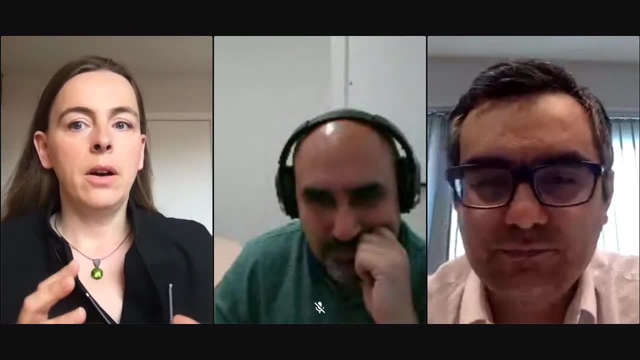 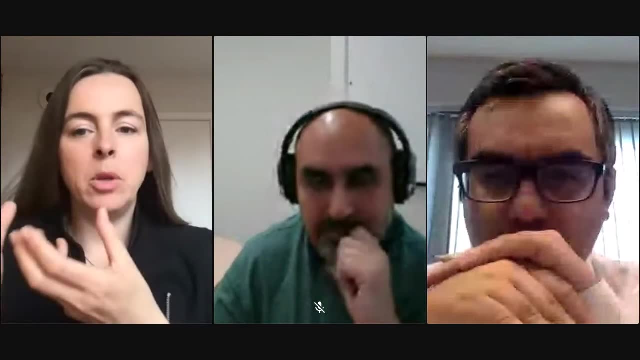 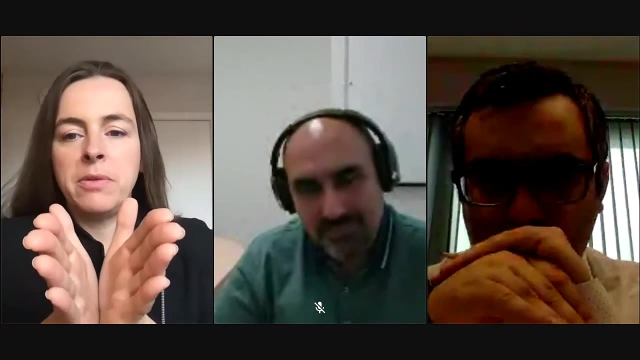 data. Thankfully, the field of view is not to do with fiber but the scanning mechanism you employ. Typically if you're doing confocal microscopy, half a millimeter field of view is feasible. That's great for confocal microscopy and that's doable. 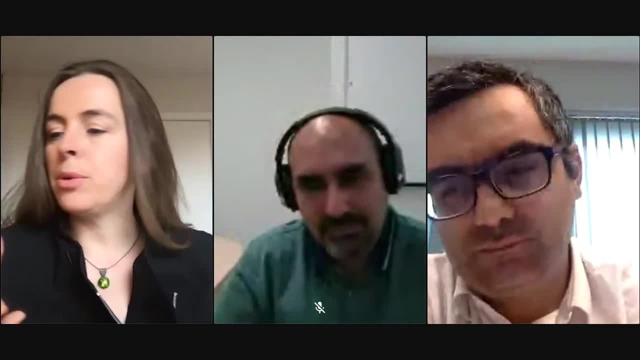 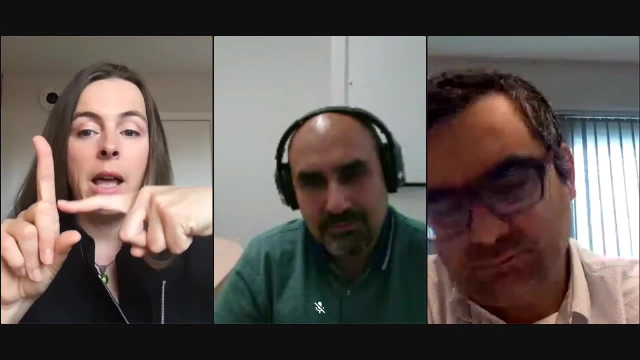 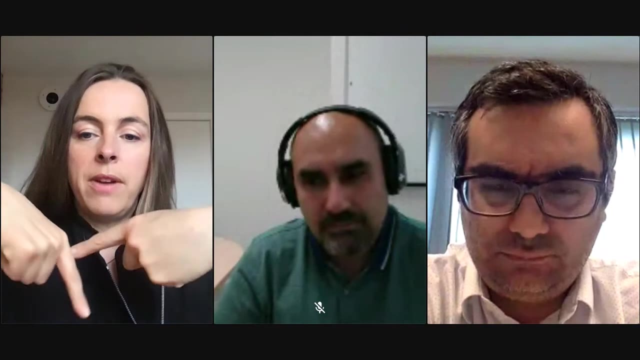 with spectrally encoded endoscopy. For OCT, the problem is different. You have your fiber optics and then you have your interference line, called the A-line, 90 degrees with respect to your fiber. As you rotate your fiber, you acquire full circle. 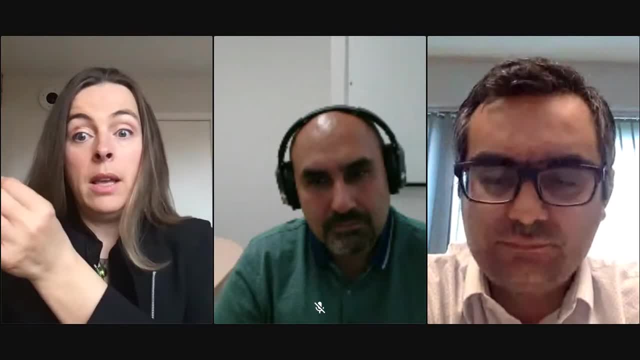 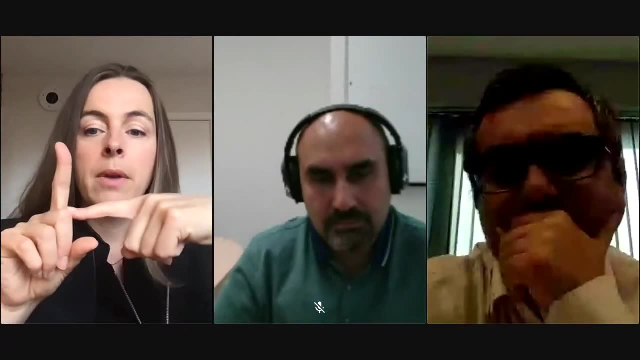 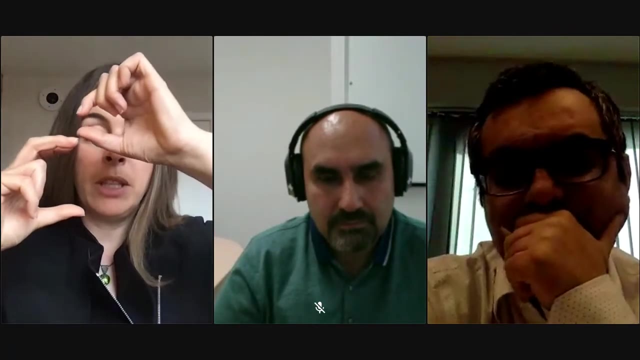 and as you pull your fiber, you get your 3D. The only dimension that is limited by physics is the depth. You can have the working distance being like three centimeters away and only imaging, but the physics tells you you won't be able to image more than 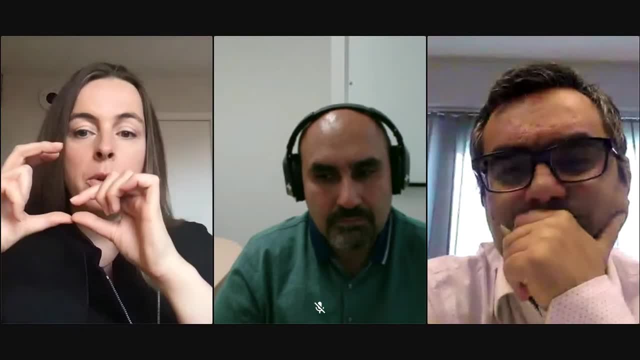 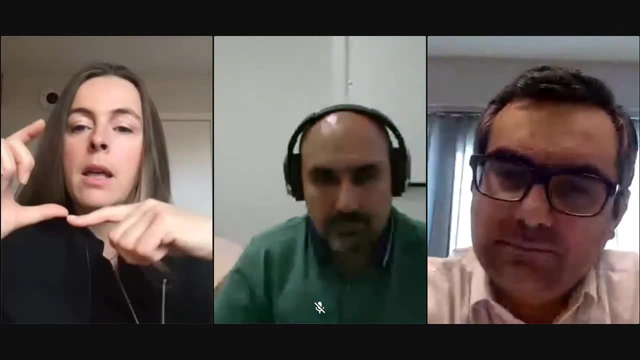 one to two millimeters. That's essentially your field of view, but you can have your field of view close to the axis or far away from the axis, depending on how you design your working distance. You can have that and you can decide to pull for 30 centimeters. 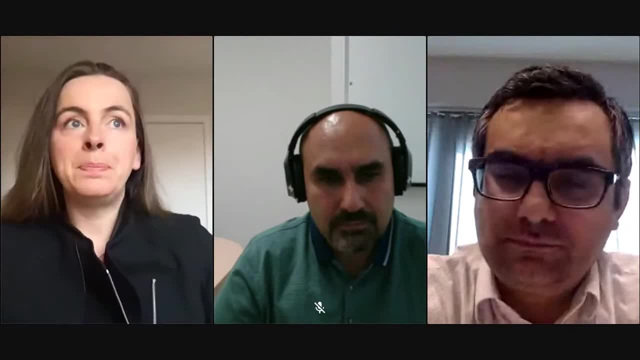 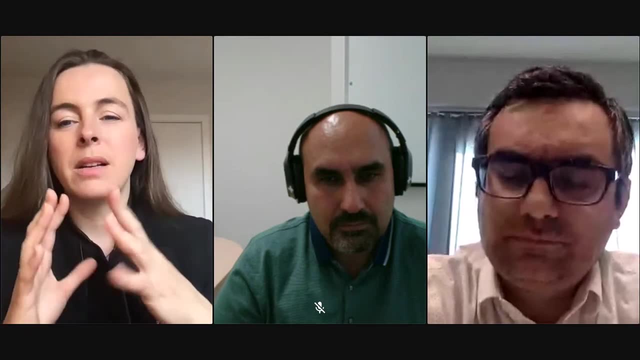 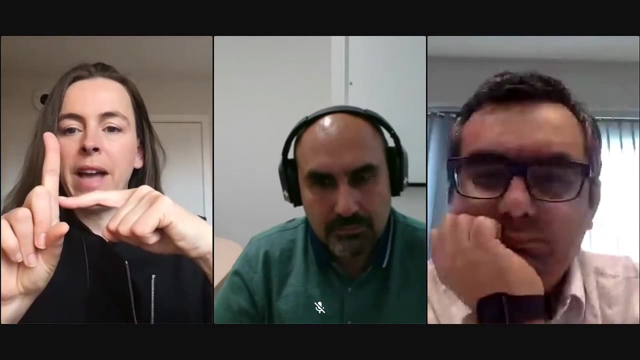 and do the entire esophagus in a matter of minutes. What's the speed of acquisition? Confocal microscopy, depending on your SNR? let's say 30 frames per second. That's good For OCT, it's a matter of how many. 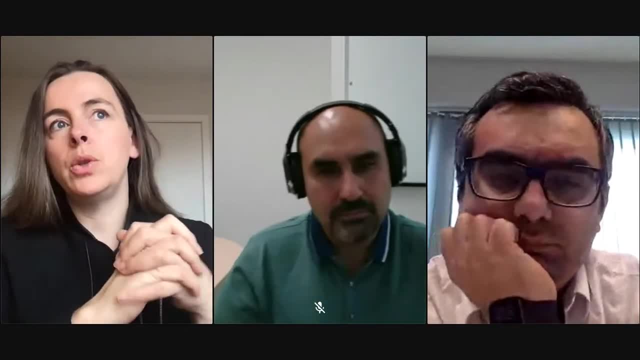 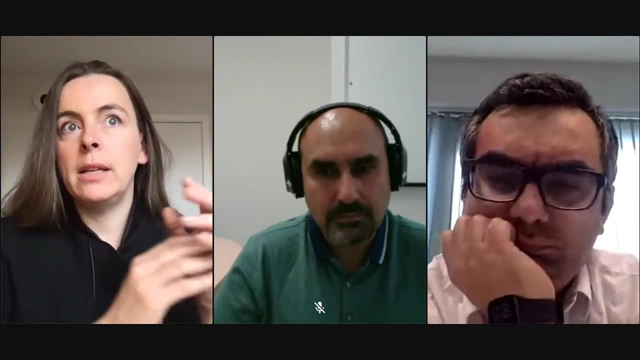 A-lines you get per second. I was mentioning that with our laser we do 100,000 A-lines per second. but there are groups pushing, especially in Austria, groups pushing this repetition rate- and it's not commercial yet, but to a million. 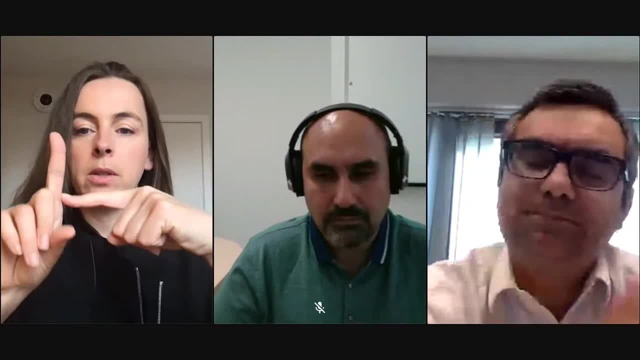 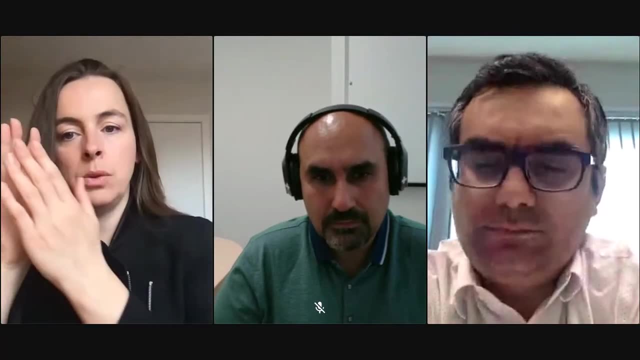 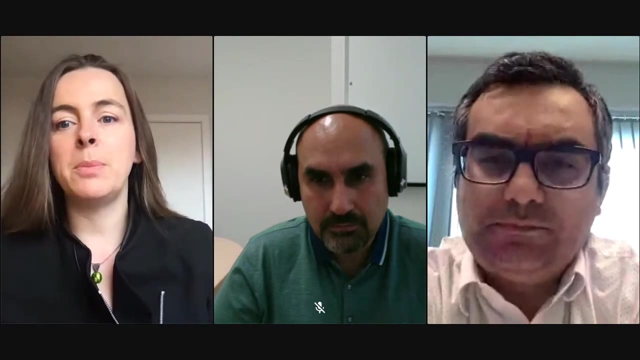 A-lines per second. Now it's a question of Nyquist: Depending on your diameter, how many A-lines you need to put next to one another to fulfill the Nyquist criterion and then pulling back With a million A-lines per second. 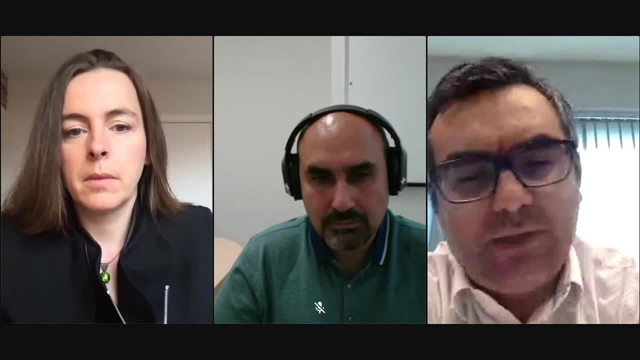 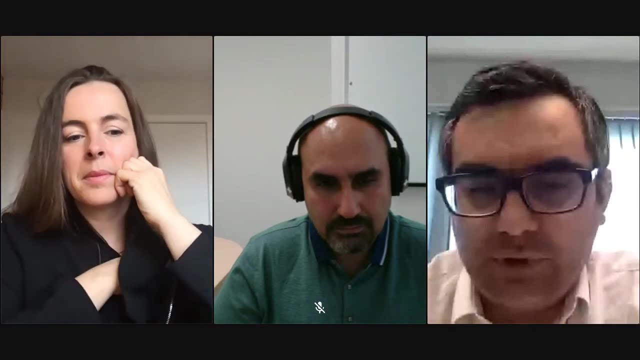 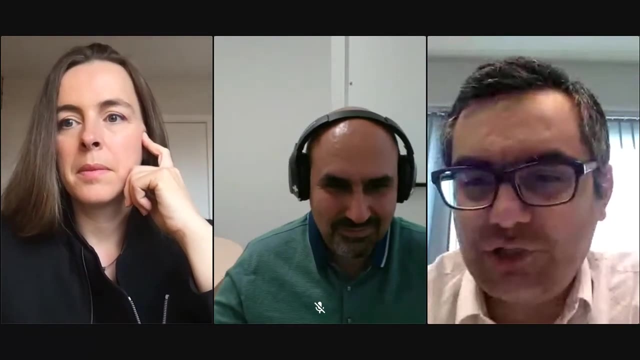 you can go pretty fast. I see, Mike. I hope you received the answer you wanted, but I think, Mike, if you are still there, I was thinking about using this technology for imaging the spheroids or the organoids that you're making. 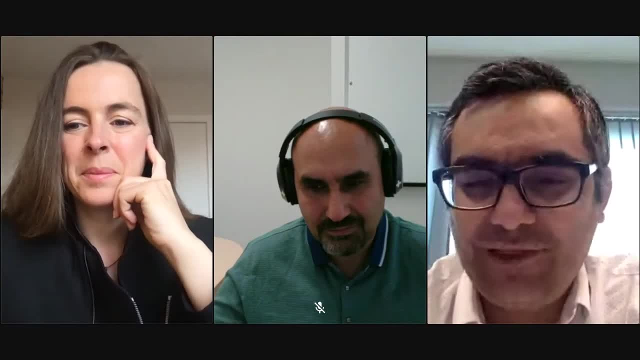 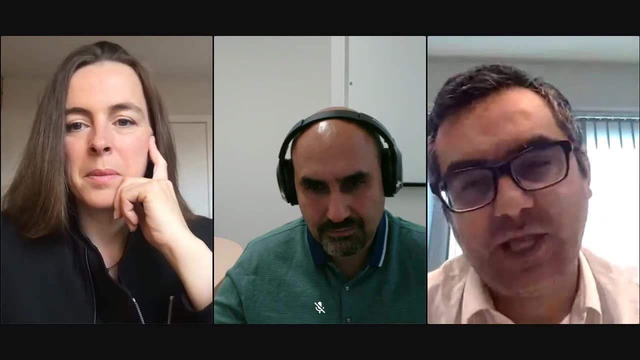 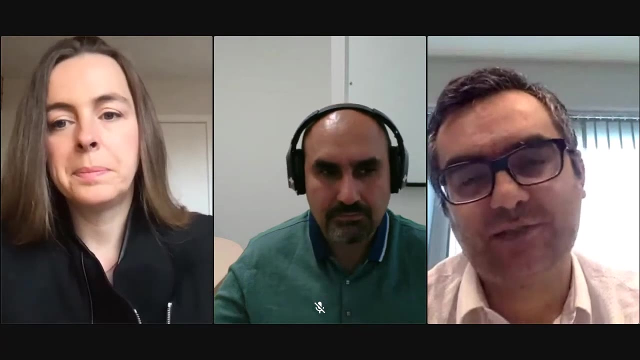 So that's a follow-up question that I had actually is that: can this technology be integrated in existing live imaging technologies for imaging maybe spheroids, tumor spheroids or stem cell organoids and things like this, In terms of monitoring? 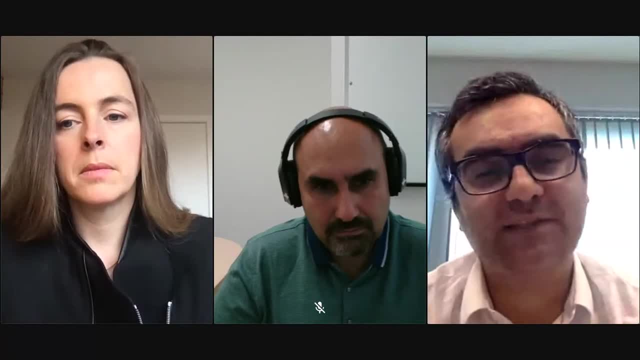 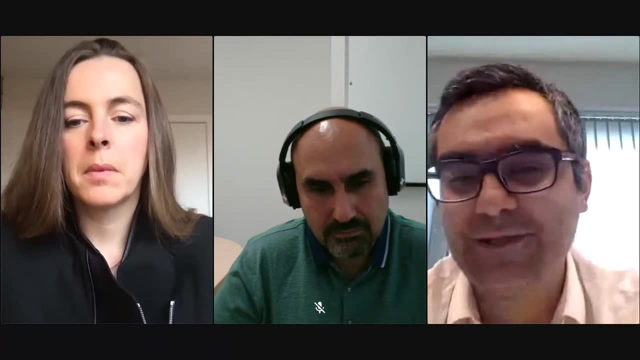 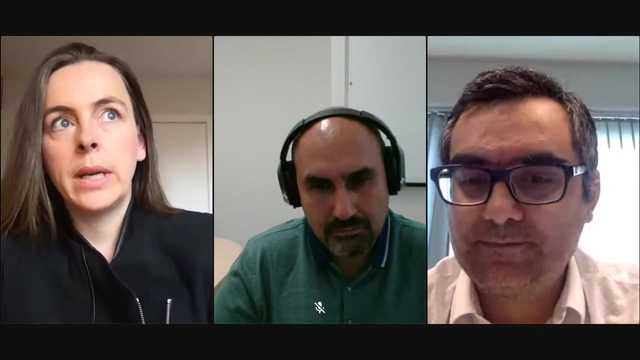 their growth or, you know, investigating the effect of drugs on these tumor spheroids, cancerous spheroids or stem cells in situ and then maybe use them for drug discovery and drug screening. That would be fantastic to do it. 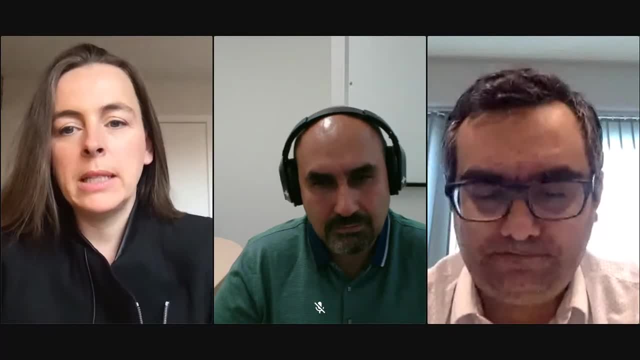 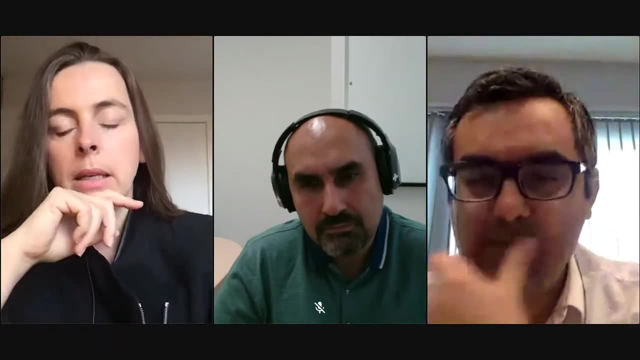 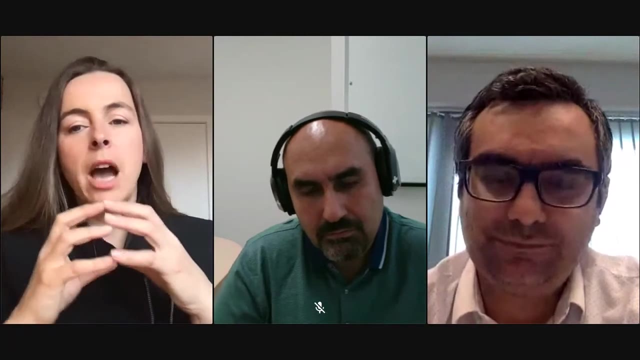 especially now that we have the spectroscopic capability. Again, if your spheroid is less than two millimeters, I think you would see through. so that would be great. But the imaging head, the system is expensive, but the imaging head is not. 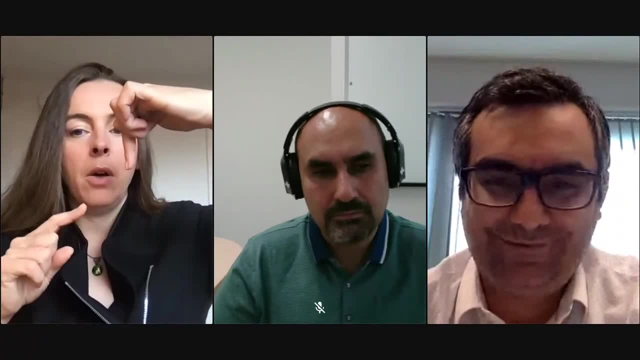 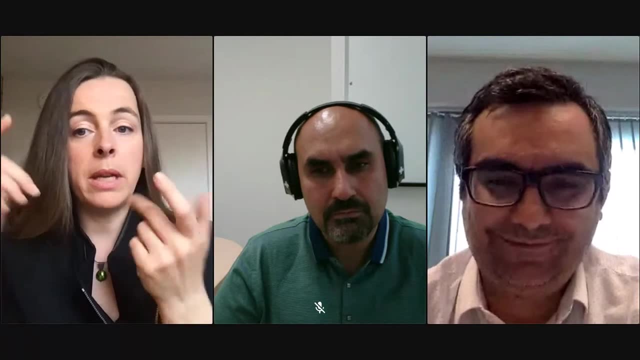 So let's think of a system that has, for example, OCT going this way, OCT going this way, and let's have a third axis. And now, as opposed to have three different OCT, you make an optical switch between the two and you say A-line, A-line, A-line. 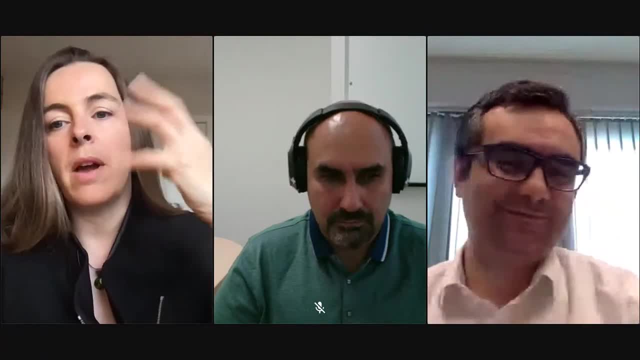 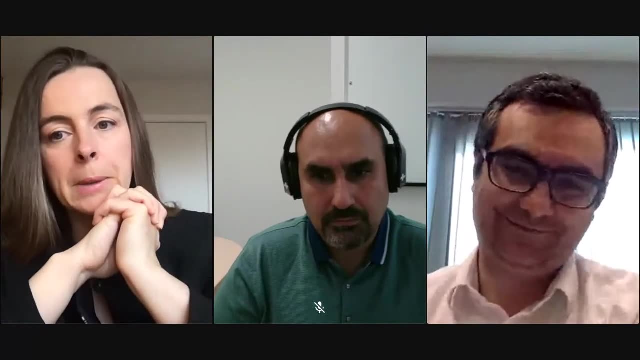 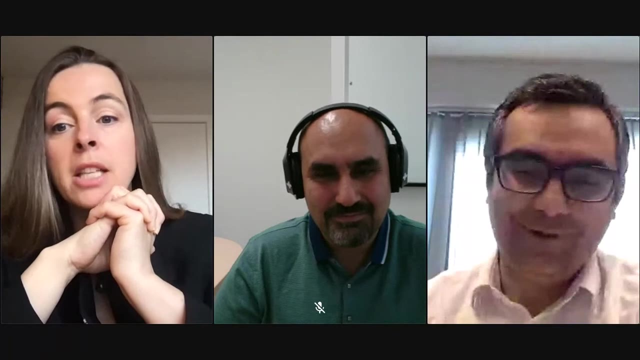 A-line, A-line, A-line and you get your system. So you can make a tomographic system. But I would say that this is a beautiful, beautiful PhD in engineering. It's a great topic for a PhD student through TransmedTech. 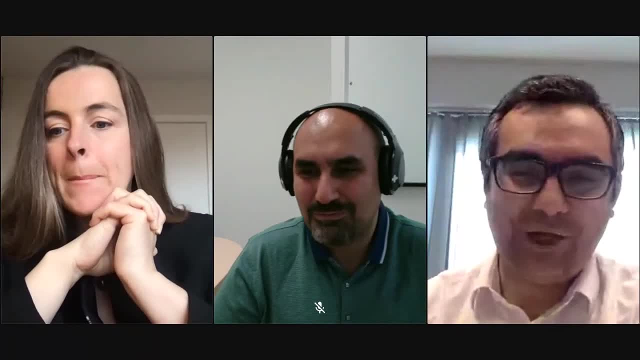 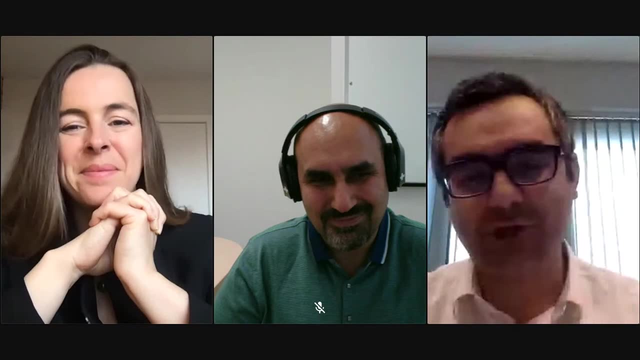 or other means Mike is even thinking about having an array on a dish. So Mike is doing a lot of work. and then he was one of our previous speakers, and then he gave a talk on stem cell manufacturing And I think he will be very interested. 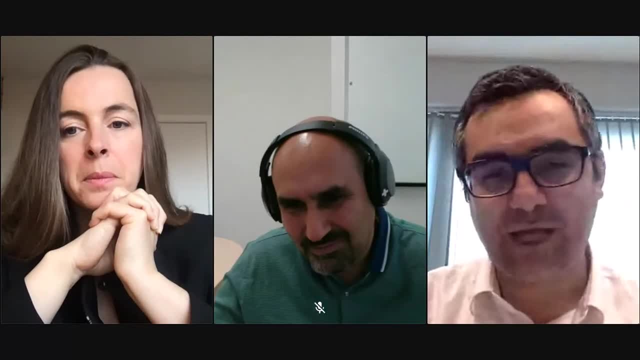 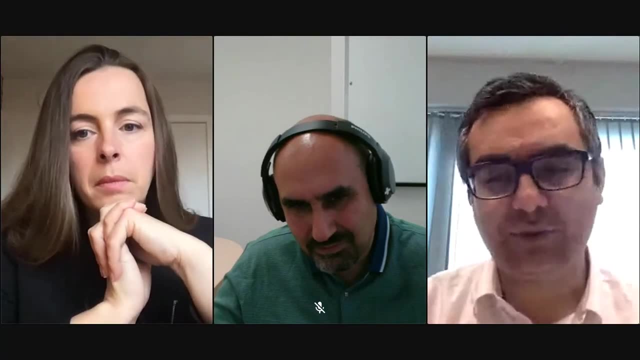 in using this technology, especially in the form of an array to analyze their spheroids- aggregates they call them- And then we are also working on tumor spheroids, And then there is a lot of potential here. I can see that. 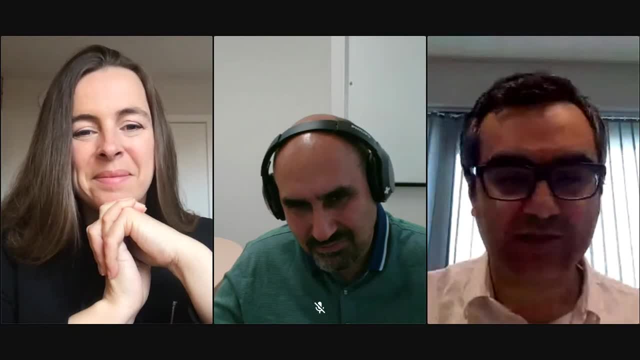 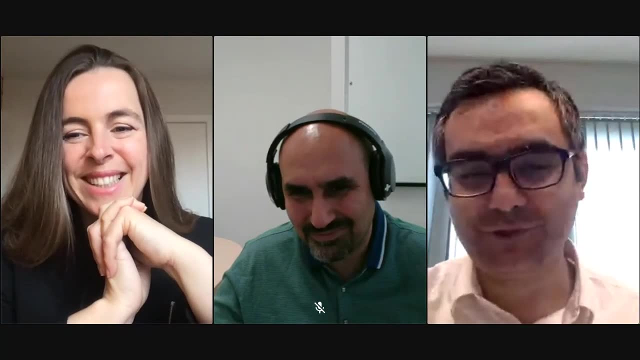 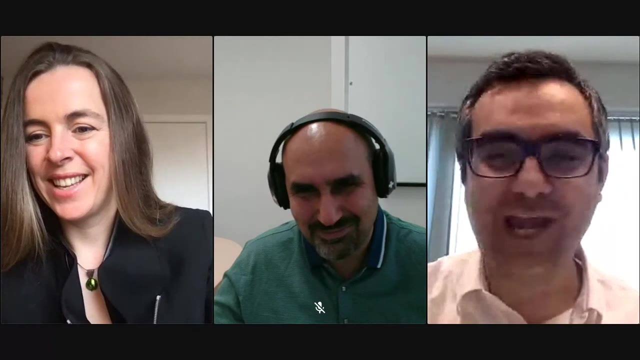 this technology can be used for tumor spheroids analysis for drug screening. Yeah, sure, I mean, Mike wants to talk to you, Me too. Fantastic, Yeah, Maybe Huma and Mike myself we can chat separately offline and then come up with a very nice. 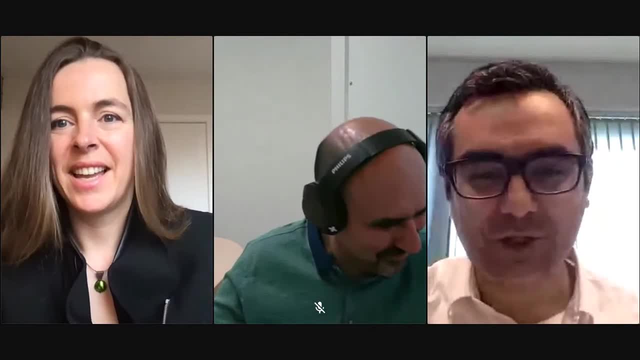 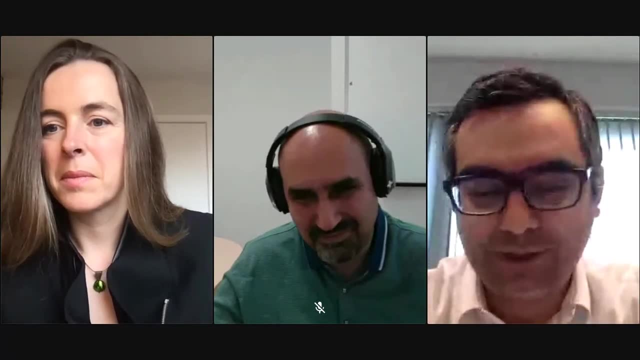 and interesting project. I'm very interested in this technology. So the next question is from Chris Flores from our university. So, Chris, he is very good in MEMS. I know him in person. He is our industrial liaison, So he is thank you. 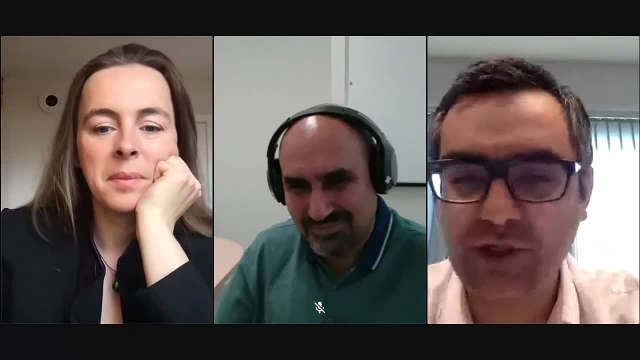 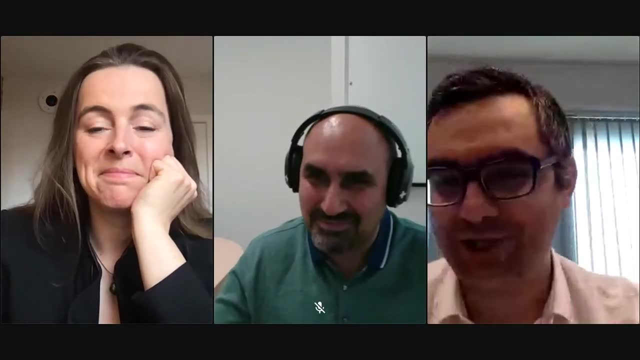 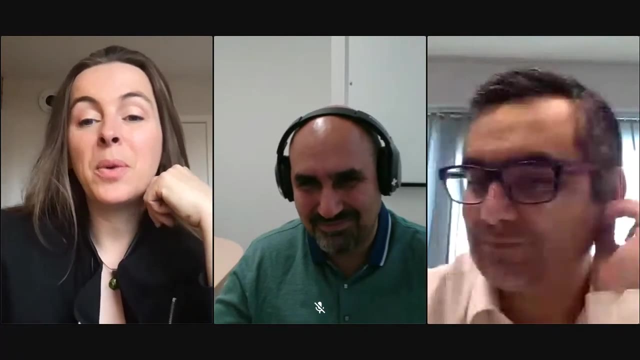 for the excellent presentation. He was wondering if you can also comment on the application of these couplers in gas detection, And I know why he is asking that, for applications in maybe CO2 capturing, CO2 sensing and then other applications. So yes, 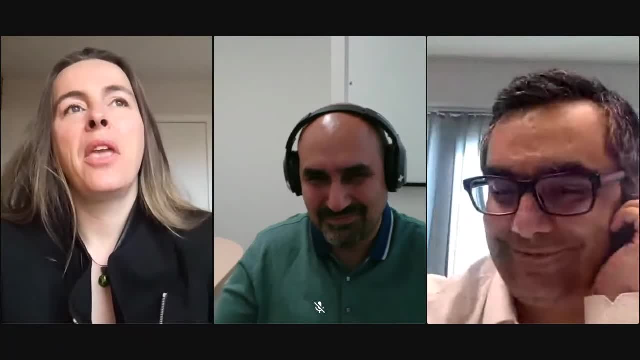 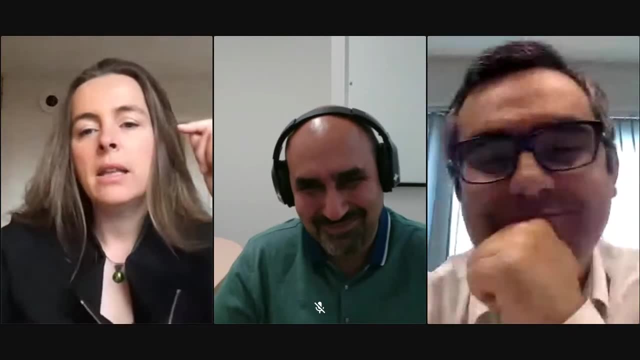 Yes and yes, I don't know if it's a secret- in our lab, but I think through TransmedTech, because it's a funded project. you guys would know that. So currently our couplers are limited at 1700 nanometers. 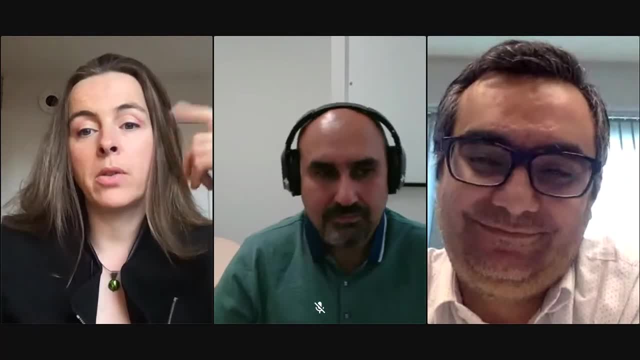 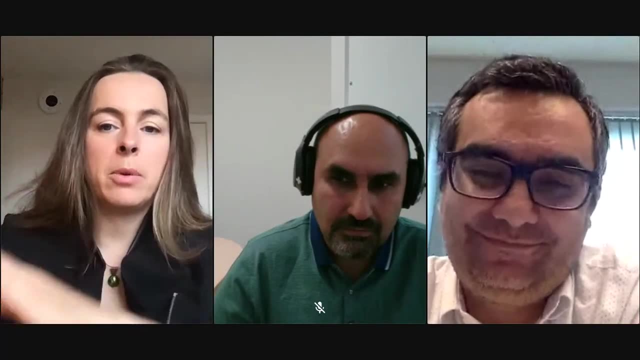 Our whole drill in terms of therapy is to bring it to 2 microns and 3 microns. That requires rethinking. It's not even redrawing the fiber. It's a new type of fiber material and it's a new type of fiber optics. 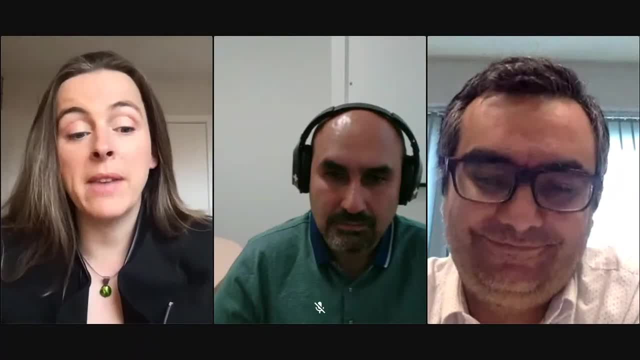 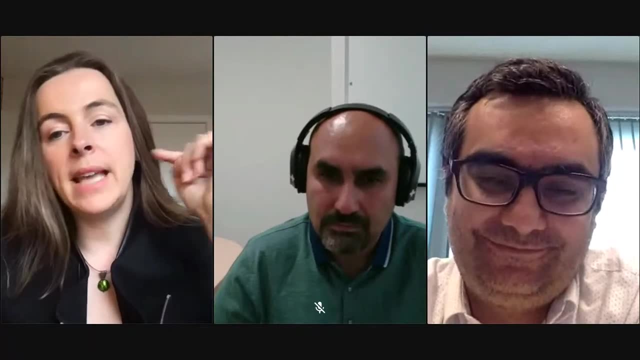 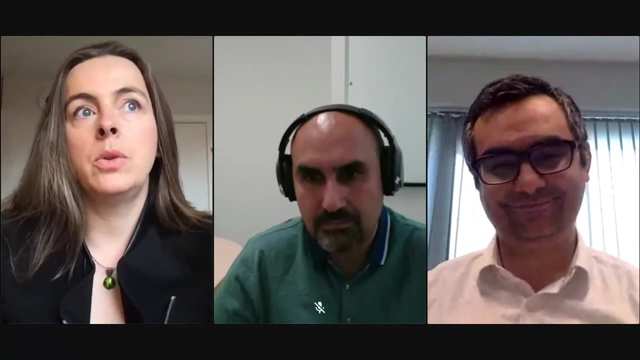 It's a new school of design and that's what we're working right now with. We have a student funded through TransmedTech who's doing beautifully, beautiful results. So I'm saying yes to CO2, but at longer wavelength. So very soon. 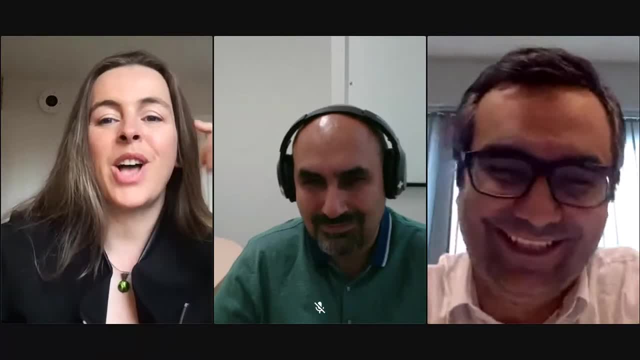 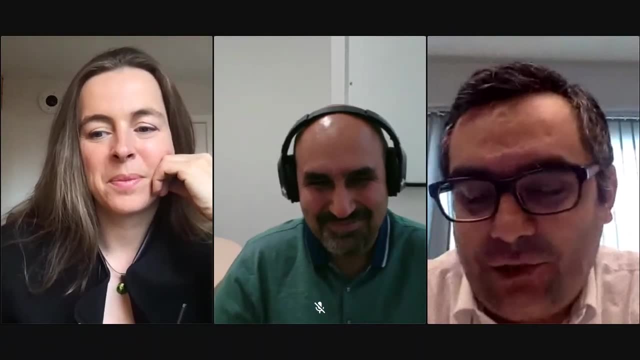 if you invited me next year, I would have great results on bringing this to 2 microns and 3 microns. But I have to put you, Chris, I think that's why you asked this. I don't know if I was correct. 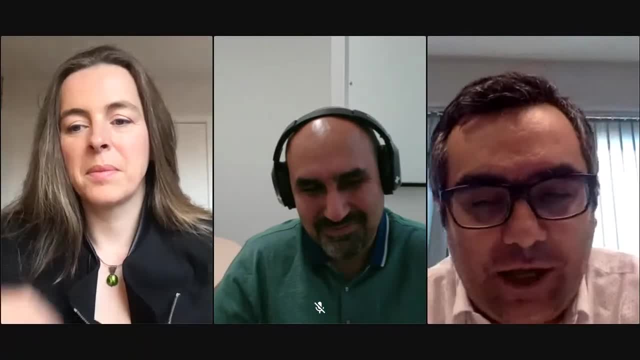 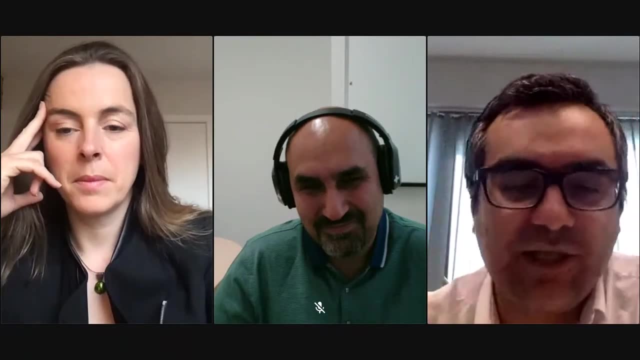 and, if I'm wrong, if you're still on the call, But I think I should put you in touch with some of my colleagues here who are doing CO2 capturing and CO2 sensing for carbon management and then these kinds of applications for energy applications. 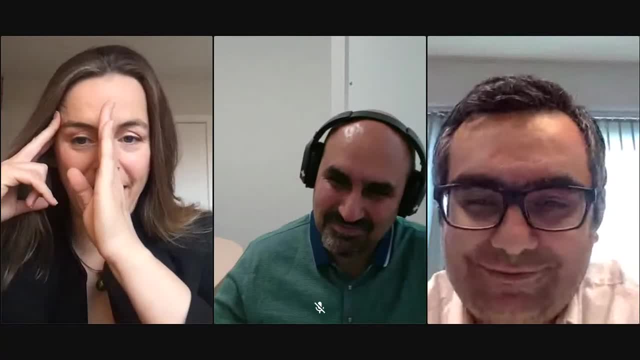 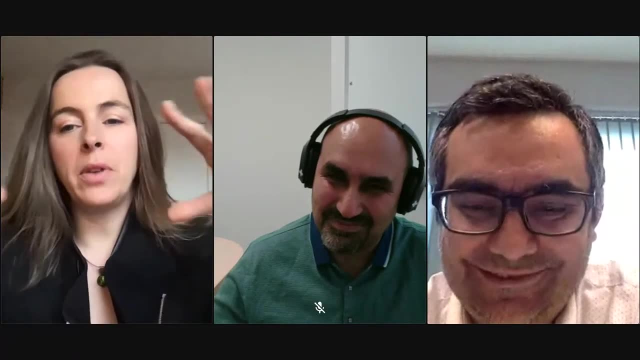 So this is very interesting. So this is where I have to separate my brain. I'm giving an academic talk today, and so the great relationship with Castor is that we're not just a startup. you know, in Montreal We have access to the world. 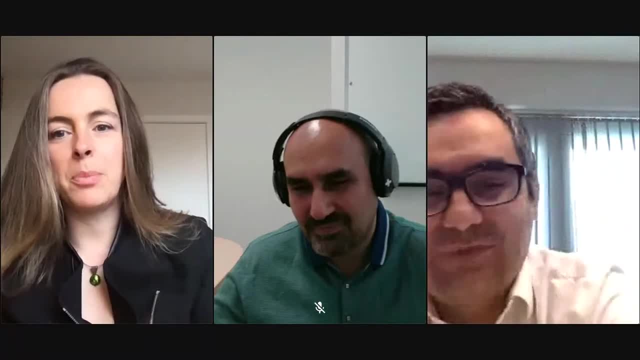 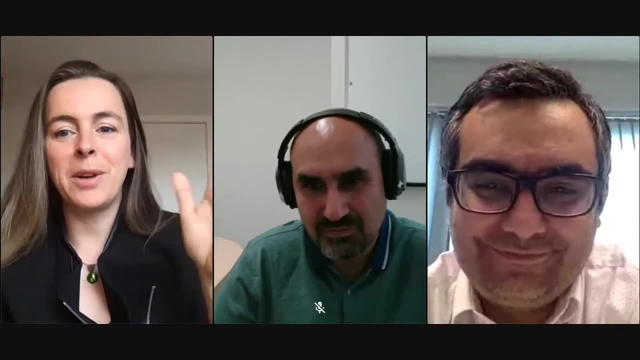 because we're in Thorlabs catalog. I don't know if you guys know Thorlabs, but it's a pretty big deal, right It is, And thanks to them we have, you know, those famous customer inspired products We have. 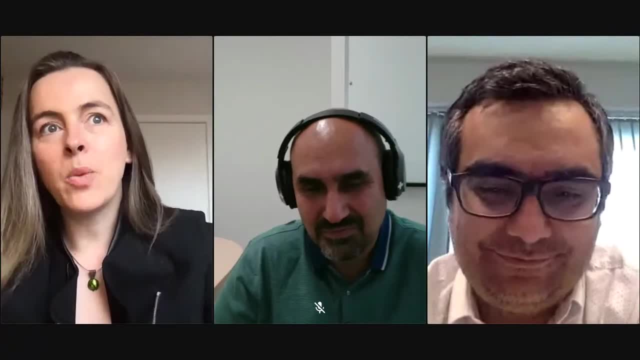 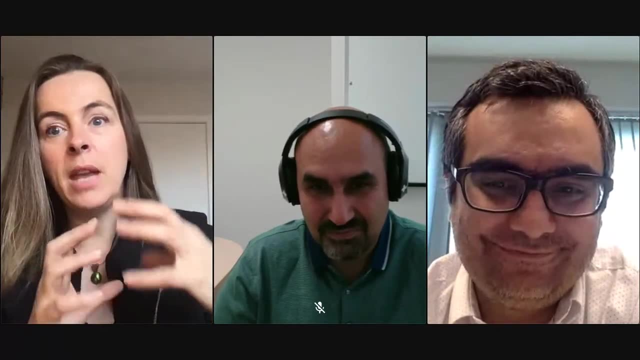 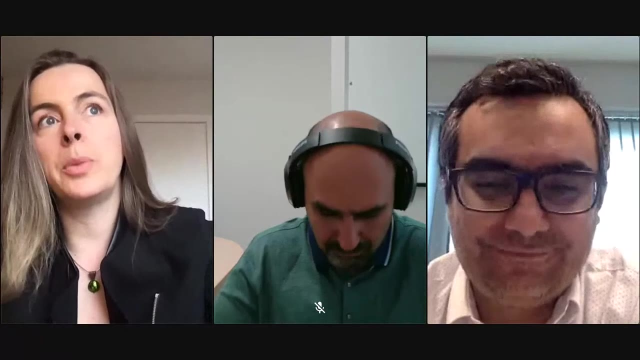 so I have to watch out, because that's why I had to scratch biomedical applications when I talked about Castor, because day one the biomed was our primary market, but in three years it's not going to be. It's super exciting too, And also from a personal. 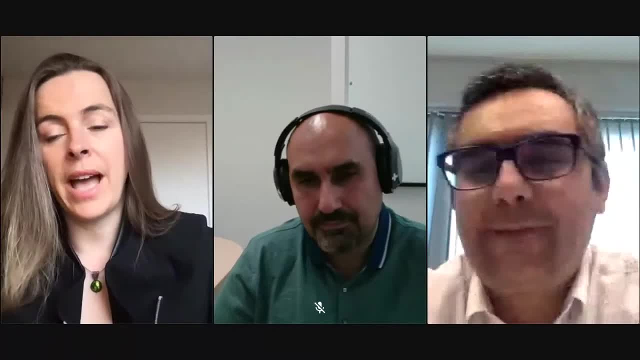 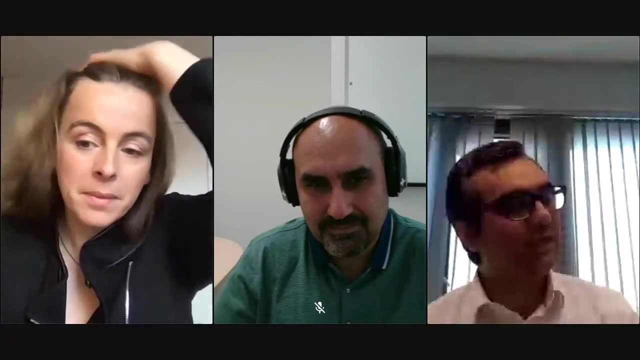 point of view, having an impact through biomed is fun. Having an impact through biomed and environmental science, that's awesome. Yeah, yeah, it is, it is Indeed. And then, in terms of biomed, I have a follow-up question. 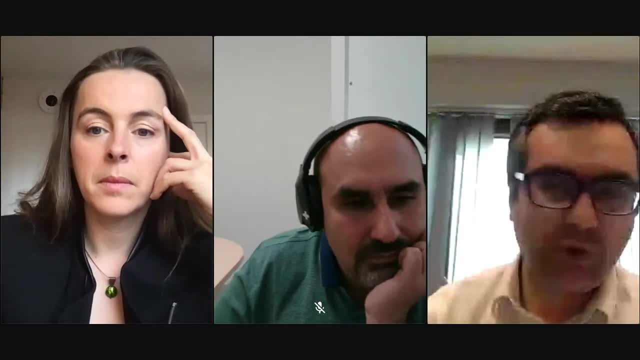 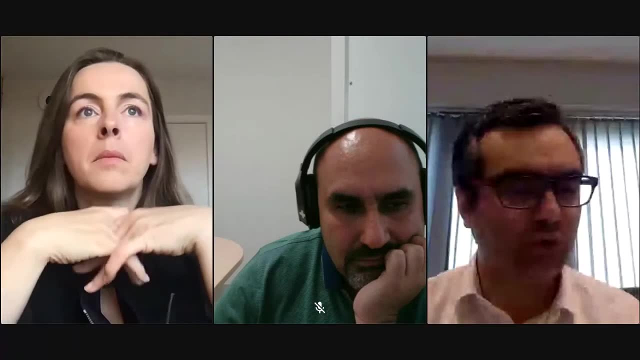 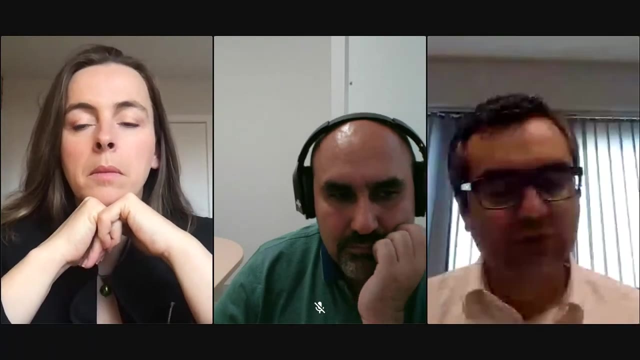 for you And that's about the. so when you enter into the biomedical engineering field- and then clinical applications of these kinds of technologies, you always think about the safety issues and the risks associated with these kinds of technologies. So let's say that you want to obtain. 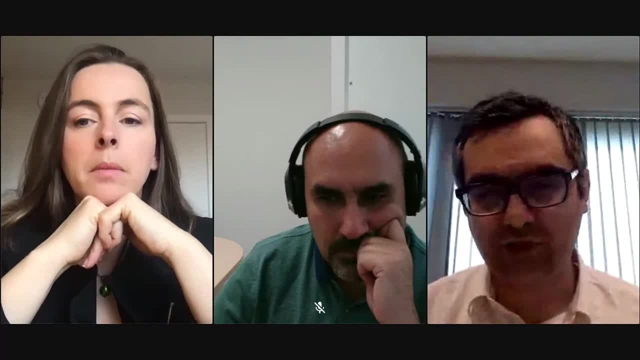 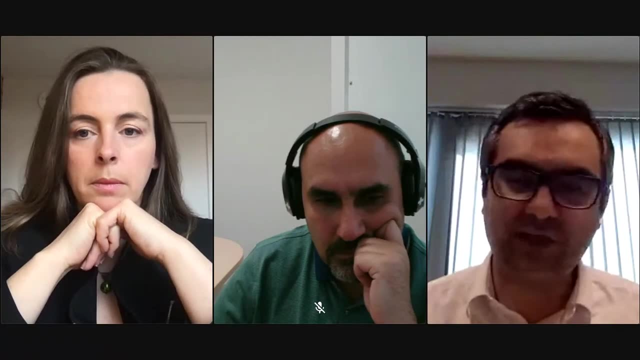 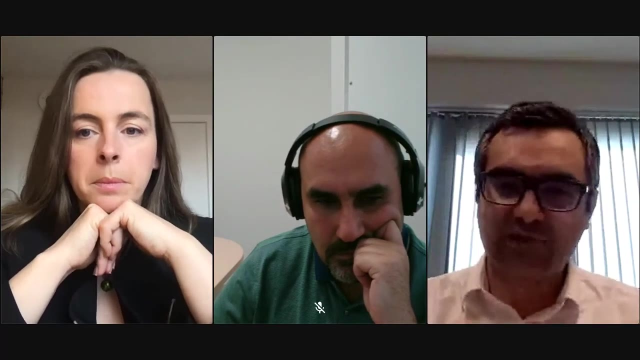 FDA or Health Canada approval for this technology right Eventually, what I envision is that these sensors or these imaging devices are going to be not implanted, but they're going to be inserted into the body to image tissues and organs in the body. 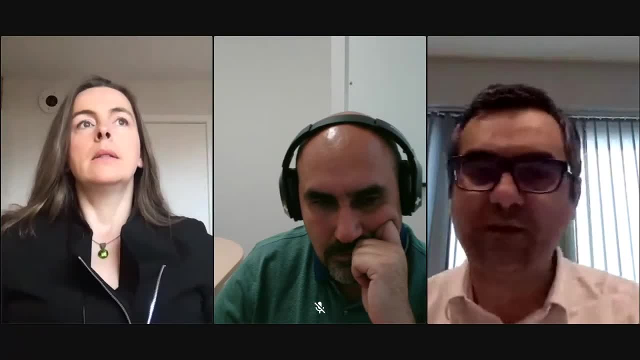 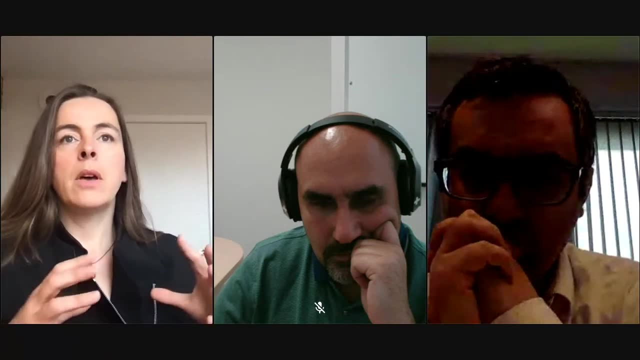 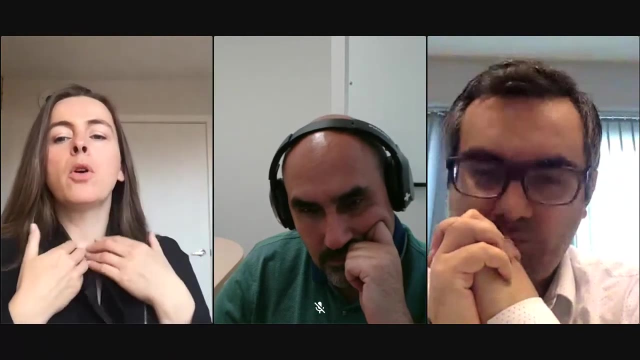 So what are the challenges that you see in terms of safety of these technologies? So I sort of cheat the system a little bit, because the vocal folds is not quite endoscopic. It's, you know, the vocal folds. I wouldn't call it an external organ, but it's. 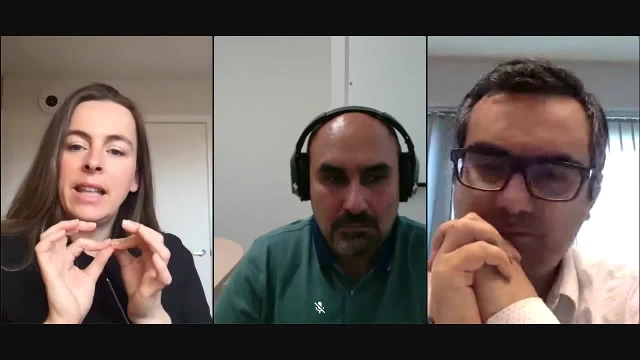 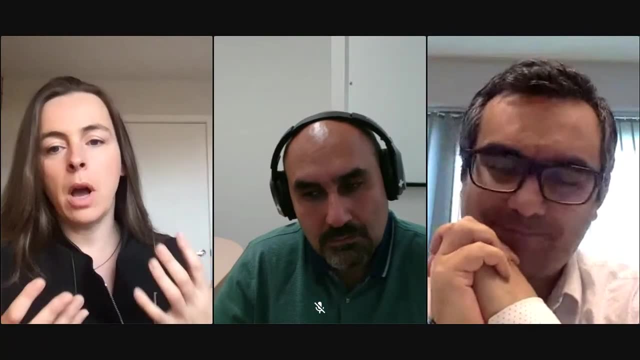 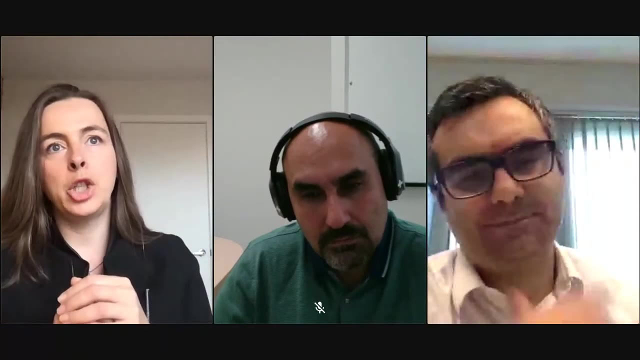 as close as you get And I can encapsulate my fiber in thick enough of a material such that I know nothing will break. but you always have to make this demonstration of the failure modes. what happens if and? so We can glue essentially everything in epoxy and 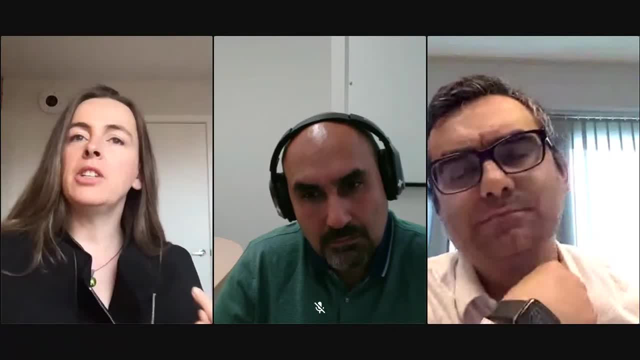 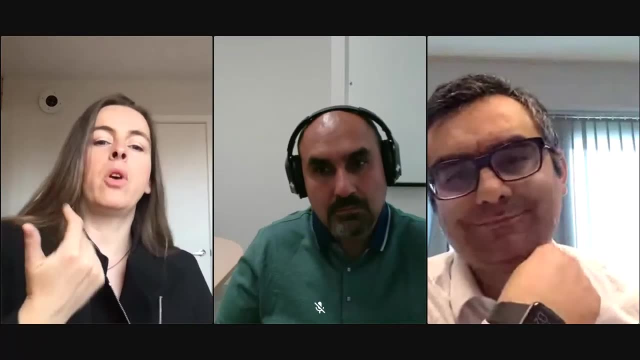 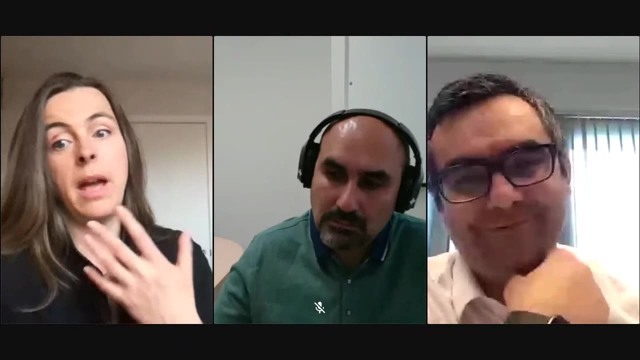 have this demonstration that nothing bad can happen. but I think the challenge is much harder when you go, for example, to do coronary artery through the femorals and you navigate through the blood And I think it's really important to get there And a technique that was used by early OCT scientists. 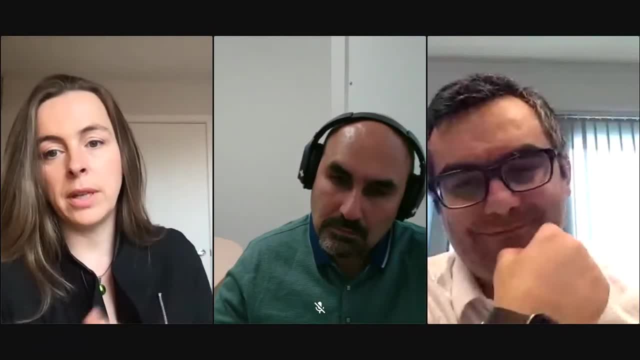 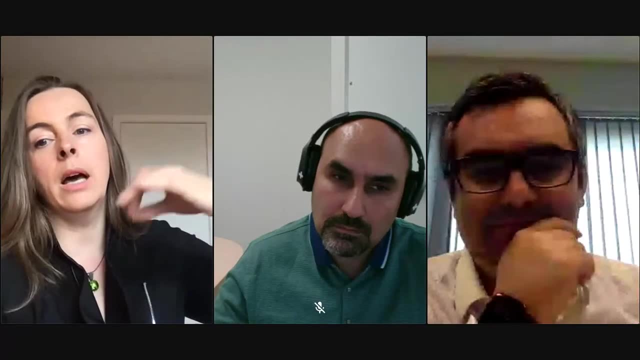 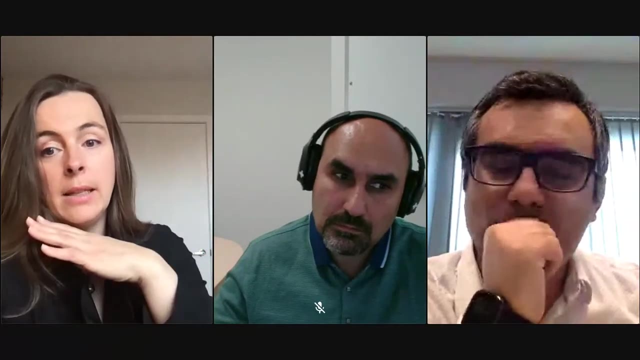 that I thought was beautiful is to take an existing system, an IVUS, for example, so intravenous ultrasound system that's already going through the artery system to get to the coronary artery, And what they did is that they took an IVUS and they stripped it out of its piezos. 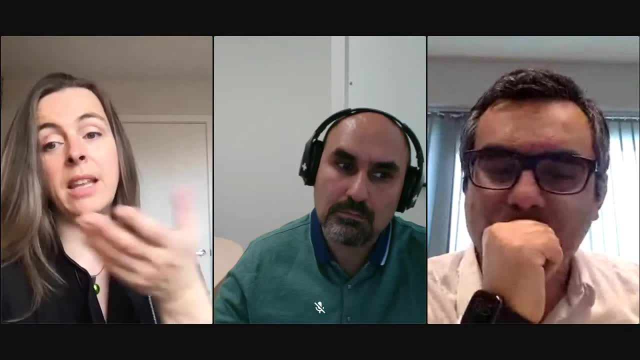 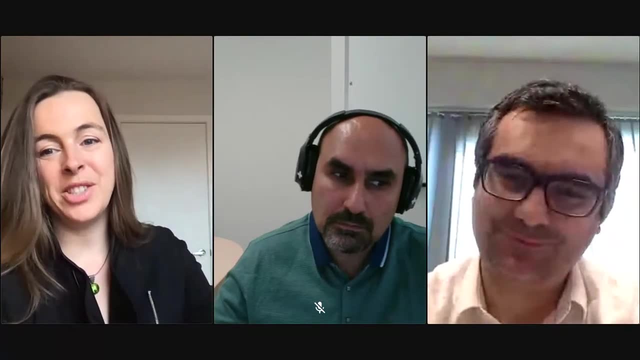 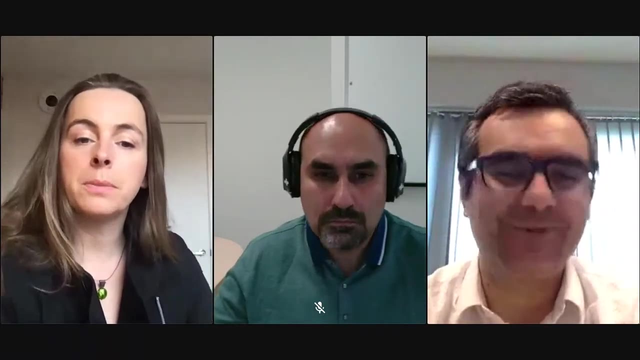 and ultrasound system and the fiber optics is so small that then they put the OCT system in it, So you leverage from people who've done it before you, essentially, And so that shows that's your first entry to this world. Yeah, that was actually. 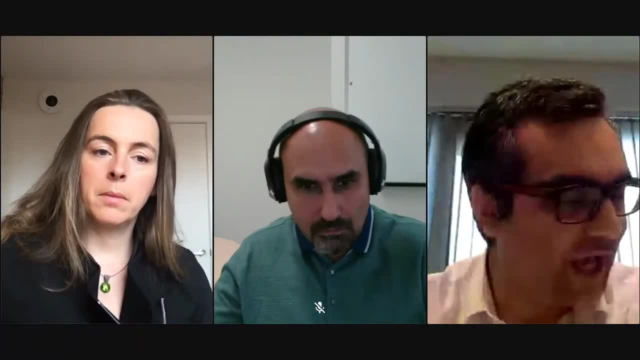 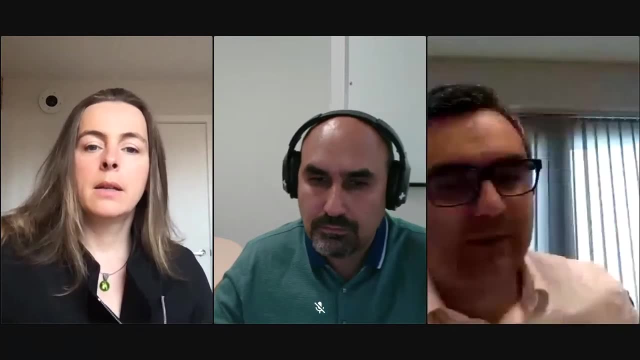 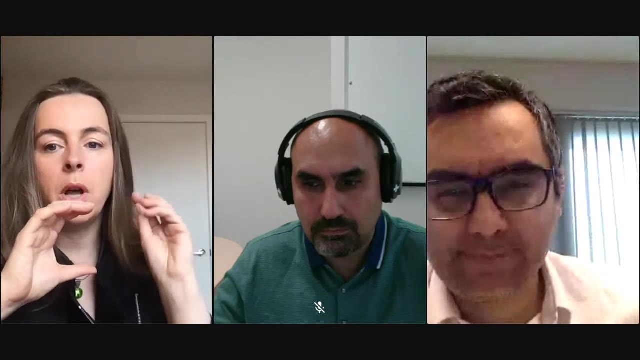 you answered my next question partially- is that whether this technology can be integrated into existing catheter systems technologies. So typically, what we do also is to so for a big industry. you have an endoscope, you have an instrument port. I lose the word. 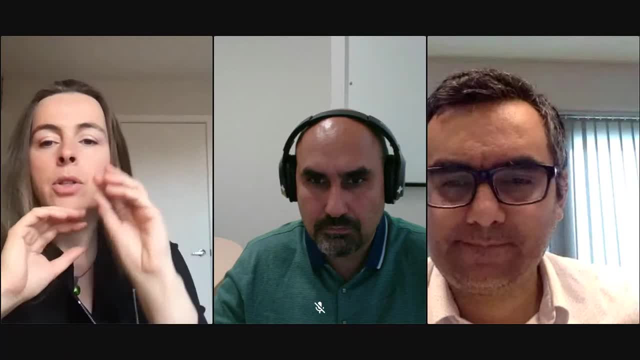 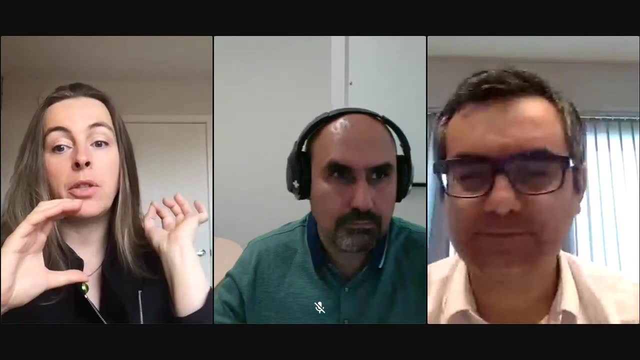 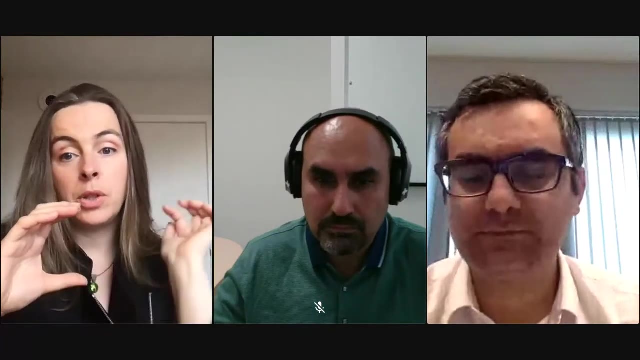 in English, to go grab it, to do a biopsy, essentially. So you have an instrument port with your endoscope. when you find an area that is suspicious, then through the instrument port you bring some forceps and grab a piece of tissue And so you can use the instrument port. 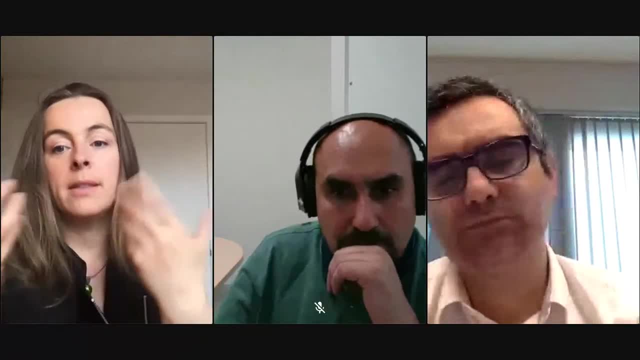 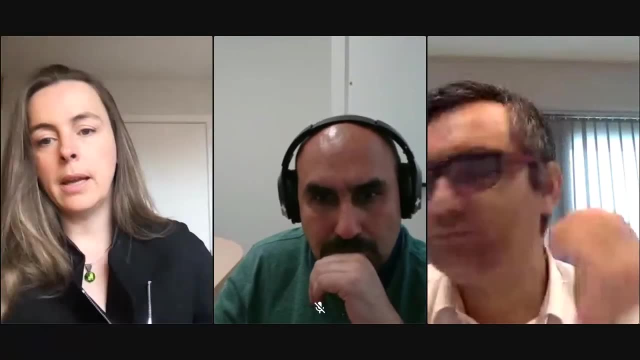 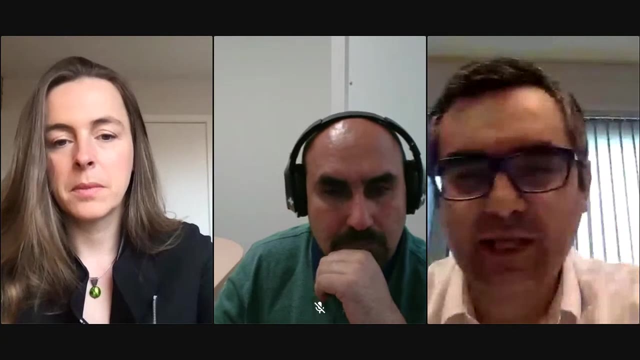 to slide your OCT slash, confocal endoscope, and this is how you again leverage the mechanical, the navigation from those existing systems. Yeah, that's very smart actually. I mean you don't want to reinvent the wheel, and then it makes your life. 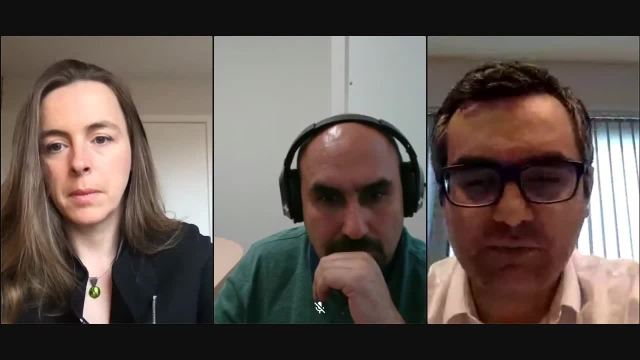 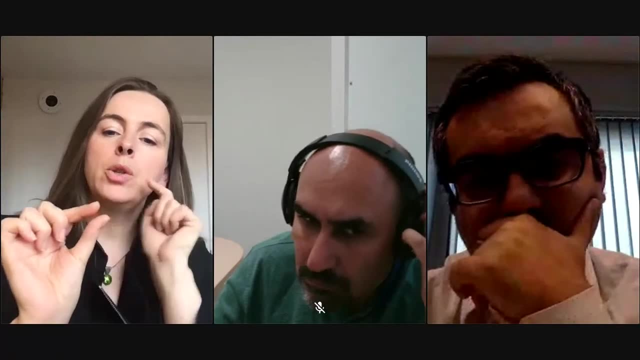 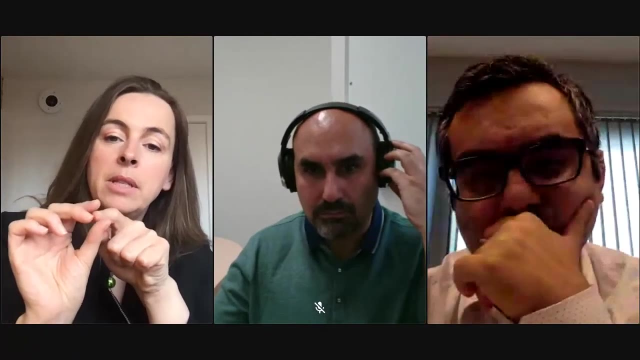 much easier in terms of obtaining the approval from the FDA or Health Canada because you rely- And some people have hacked those, so sometimes the instrument port is too small to slide it in and out, so they essentially build their. so the confocal system is a little. 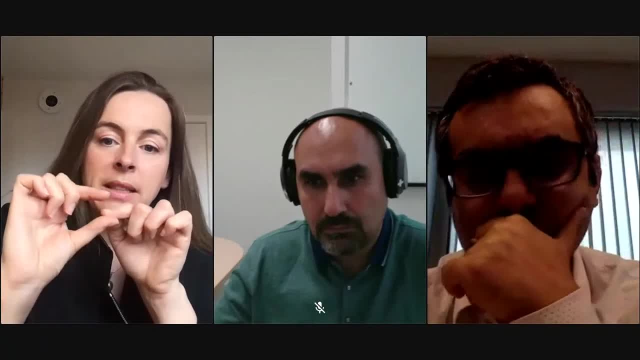 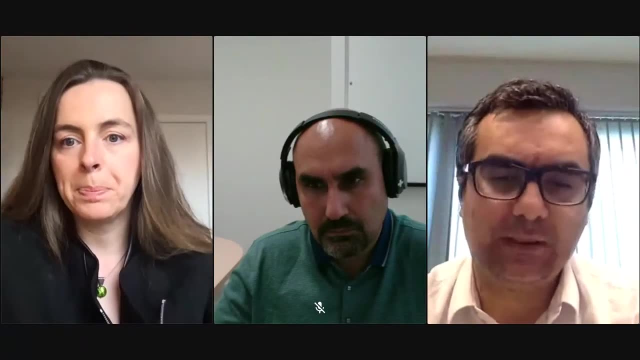 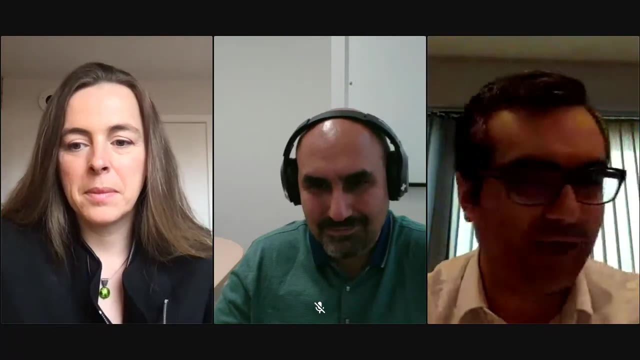 too protruding, just by a few millimeters, but the lens needs to be a bigger diameter. so they hacked it and they permanently exploited the instrument port. Yeah, No, that's very interesting. and then again, I had another question before about the ability of using. 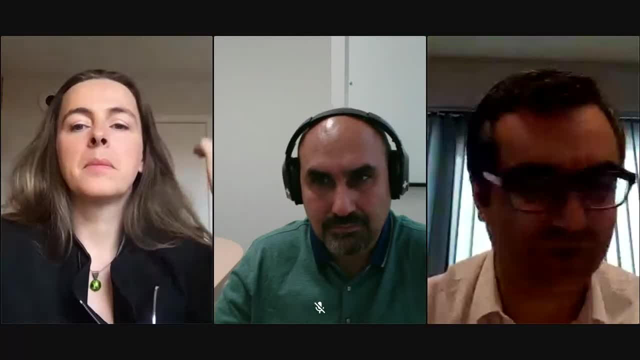 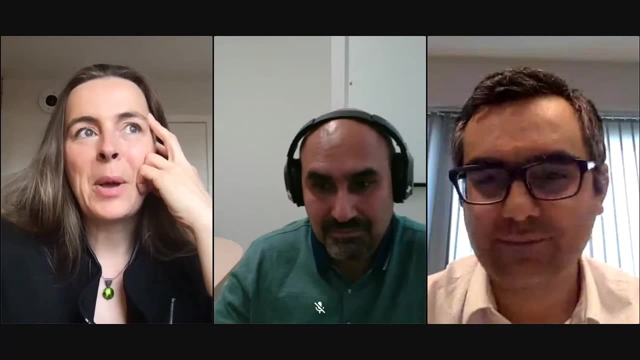 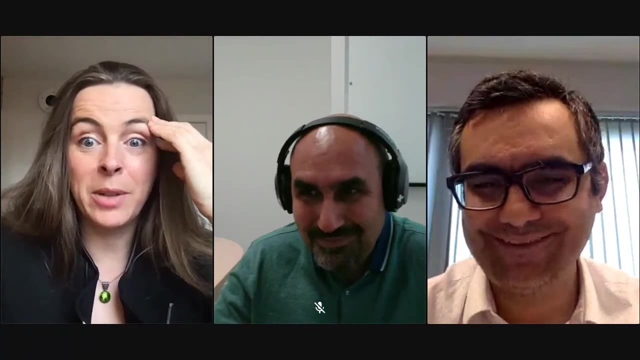 this technology for treating patients, but you already answered that question as well. nicely, with the laser ablation. basically That was my. I wrote my faculty application almost overnight because I saw it by chance and that line was the next day and I'm like. so I wrote it overnight. 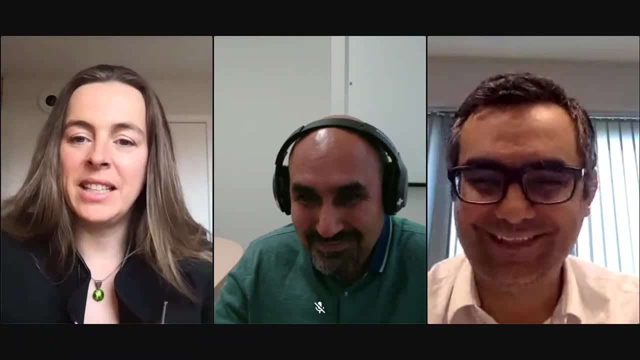 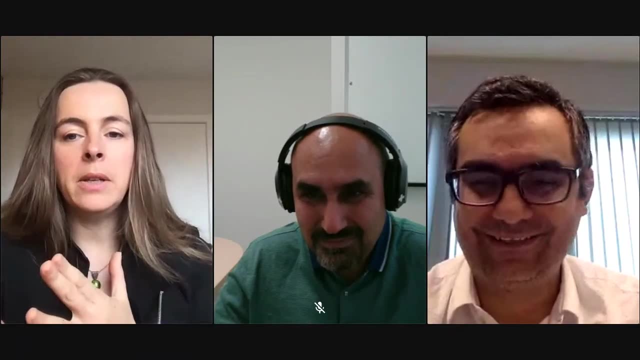 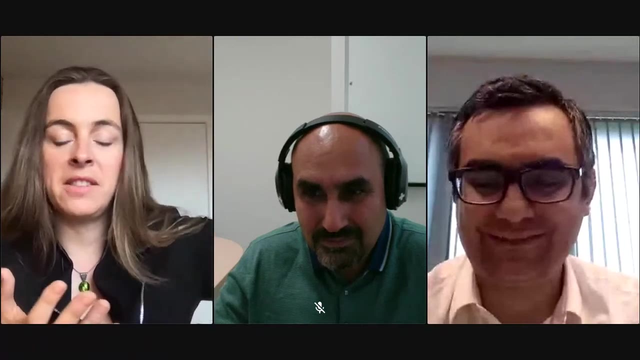 and as I was writing it I wrote this line that I said I wish one day you can. you know, after first visits, after your endoscopy, you can tell your patient you had cancer, not you're having cancer, and then you know we're going to make a course of action in six months. 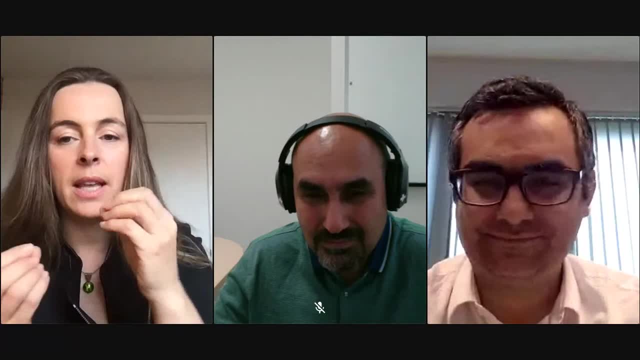 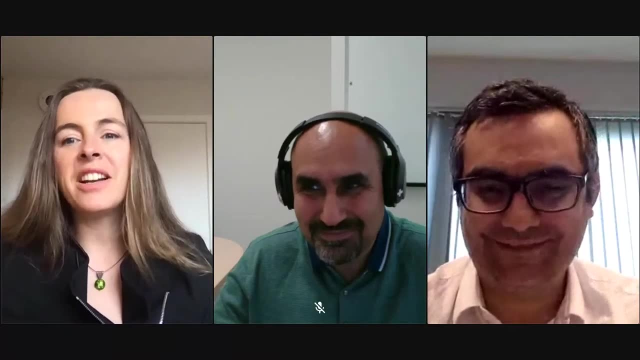 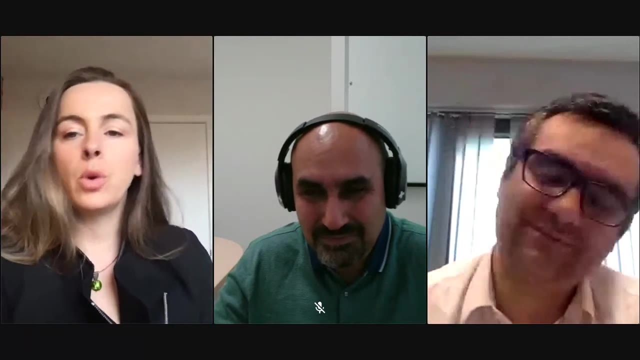 but first visit. you go in and you say you had cancer. That was a line that probably got me the faculty position in engineering physics. We're not there yet, but clearly this is where I'm heading, but there are no shortcuts, and so this is where 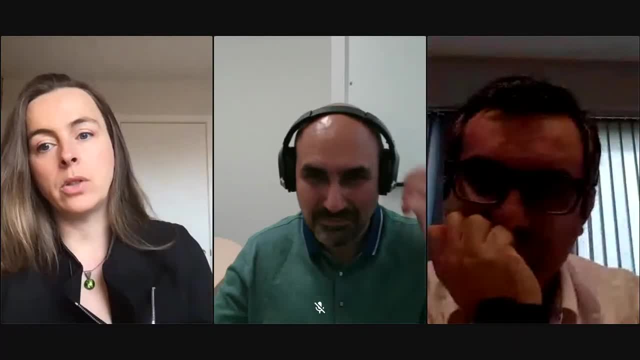 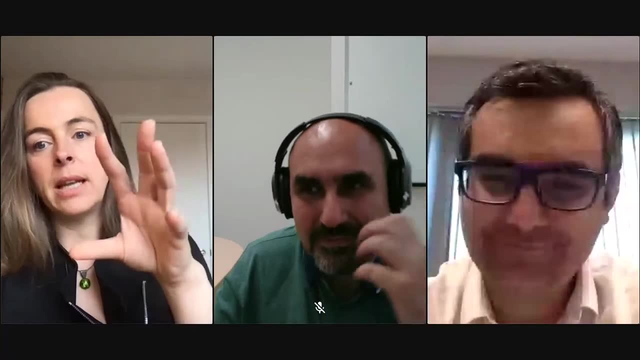 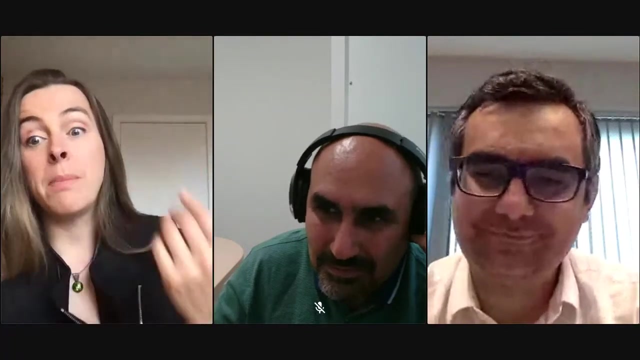 being an engineer is and surrounded by doctors, so you always want to be talking to doctors all the time, but here, surround yourself with material scientists, with experts in fiber optics. so I found Nicolas Godbout and just listen to the new technologies, MEMS people, just to be able to. 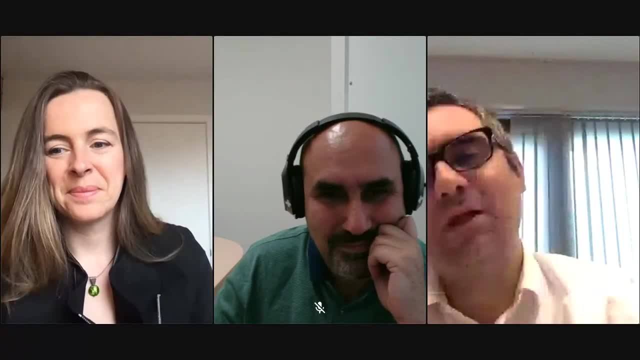 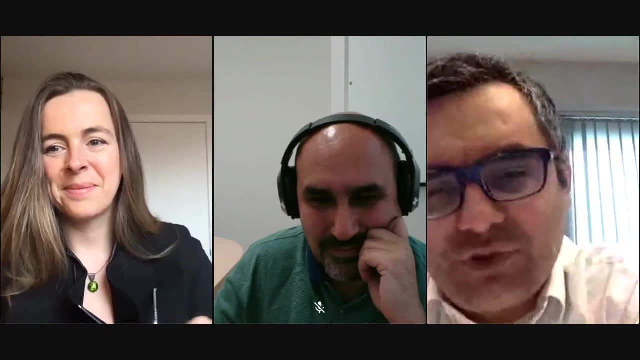 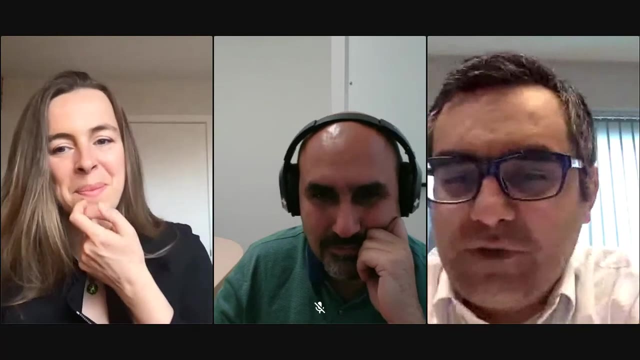 enable that Very interesting. and the other question. Mike has another question, which was my question too, and then he's asking about the effect of movement on the images. so we're dealing with organs that are moving in the body: blood flow, person breathing, etc. 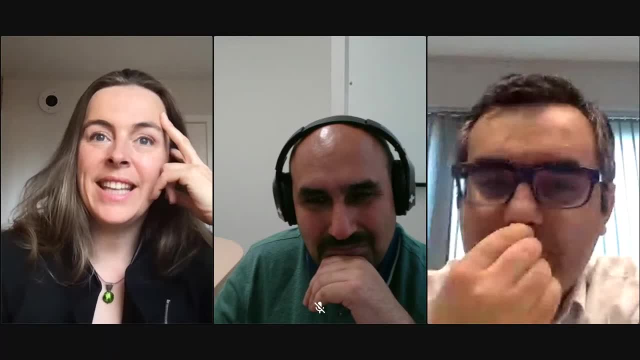 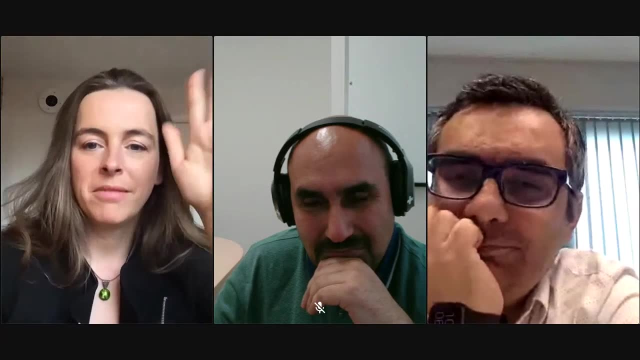 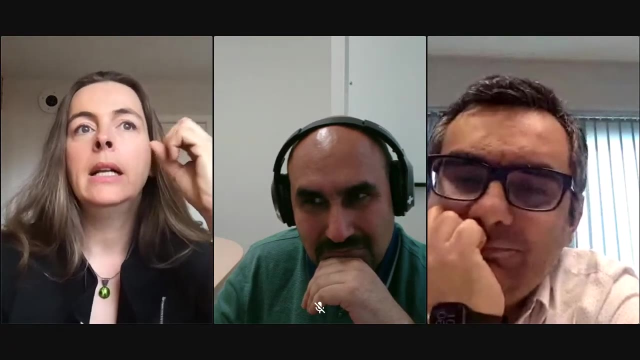 What are these effects on the measurements? Yes and no in OCT at a million A-line per second, you're covered. This is fast enough that you're going to be faster than motion. typically, The problem is with our spectroscopic data. if you're doing, 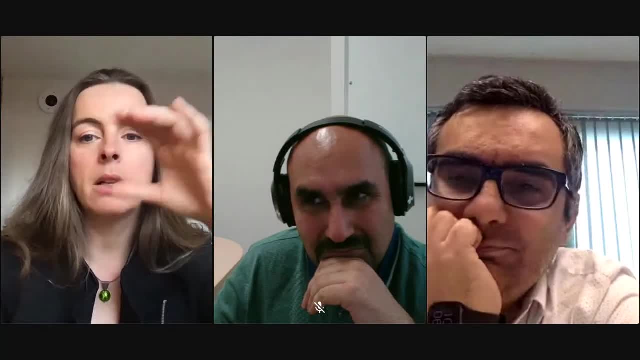 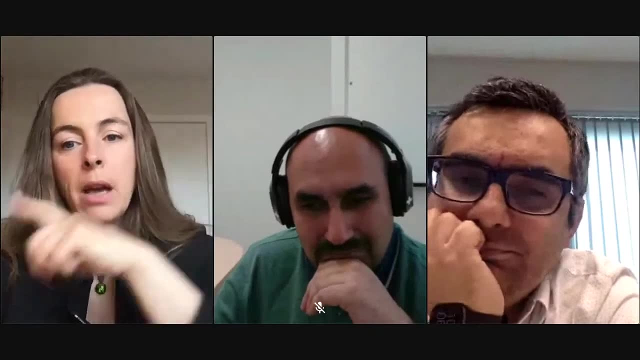 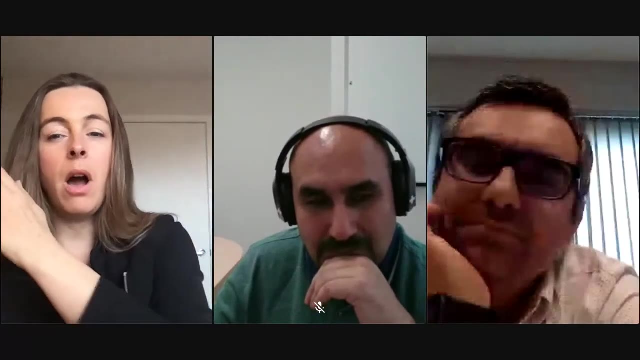 even if we have a hundred times more signal, spectroscopy has really, really weak SNR. so this is where the work of my other student, Xavier Tendu, is so important. so he said: okay, in the lab we're going to do hyperspectral imaging, we're going to get all the 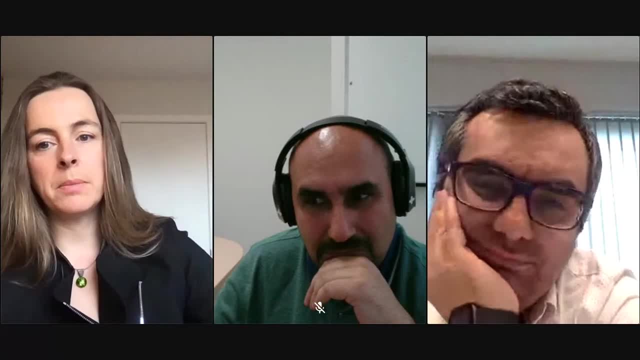 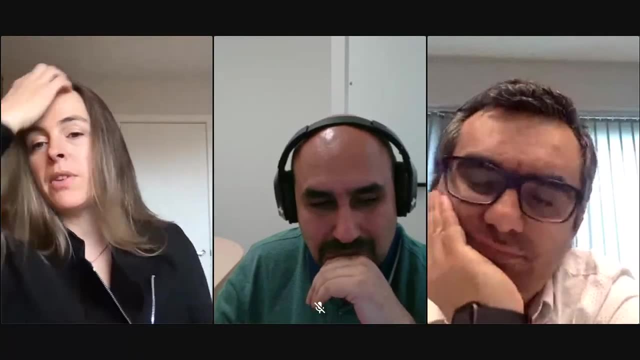 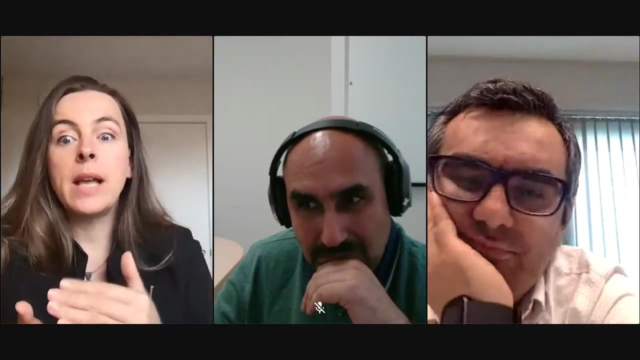 wavelengths and we're just going to learn everything we can from that system. but hyperspectral imaging, generating so much data, processing, the spectrometer required for that, I'm not going to call it impossible, but it's going to be impractical because it slows down your OCT. 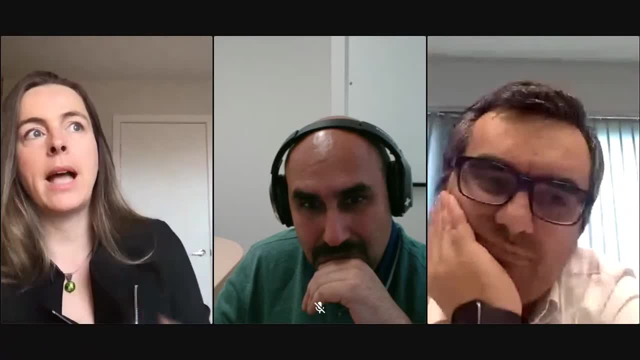 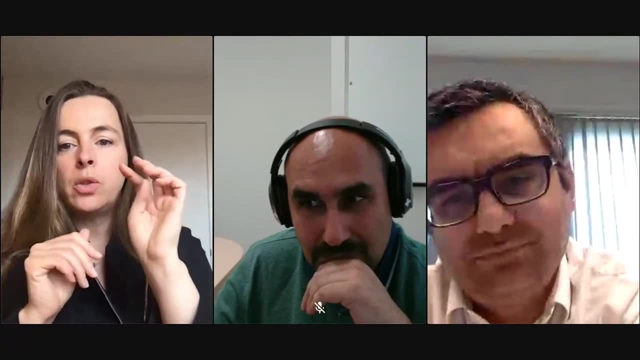 your OCT can never catch up with it. so what Xavier is doing- and I didn't have time to present- is to say: okay, so in the lab we have the hyperspectral system. let's find which 3,, 4, 5 bands that we need. 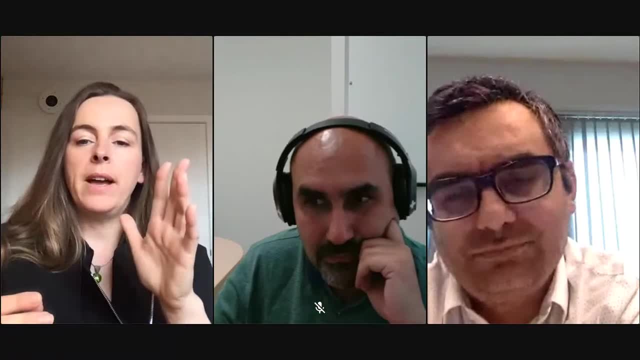 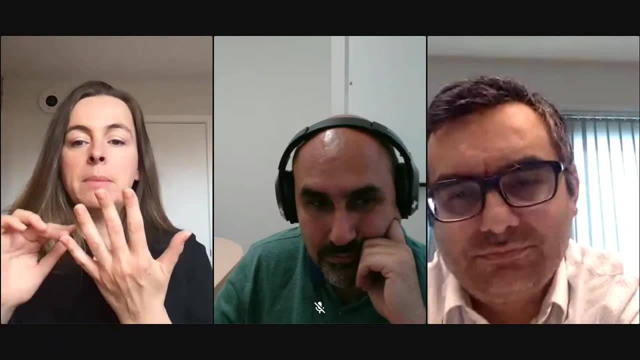 and then we're going to make a multispectral system. that is super fast. so what he does is he, as opposed to have a white laser, he sends a laser with 5 colors that he modulates in frequency and does a simple transform. so now his multispectral. 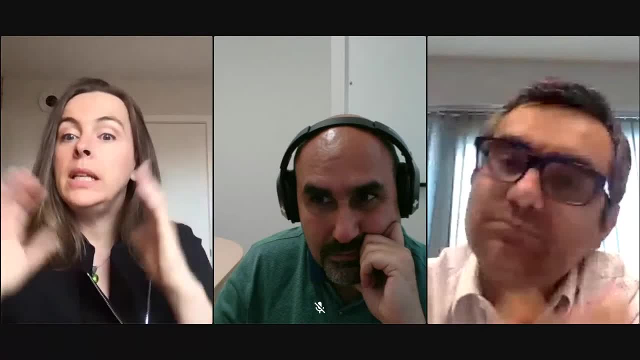 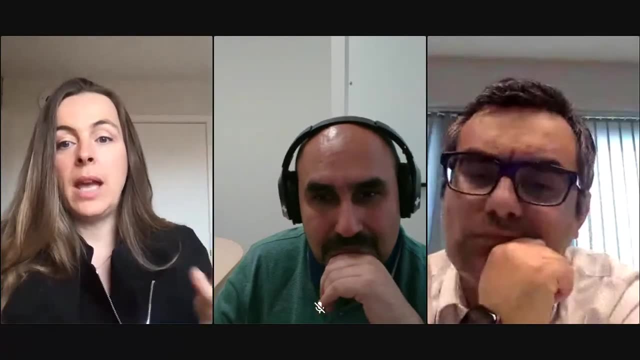 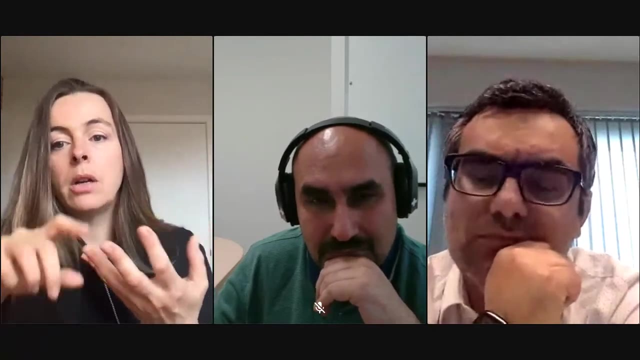 image is as fast as OCT, but you need to have the hyperspectral system in the lab to work out everything you can from the tissue. you select the required band for your application. are you looking for oxygen map? are you looking for color? what are you? 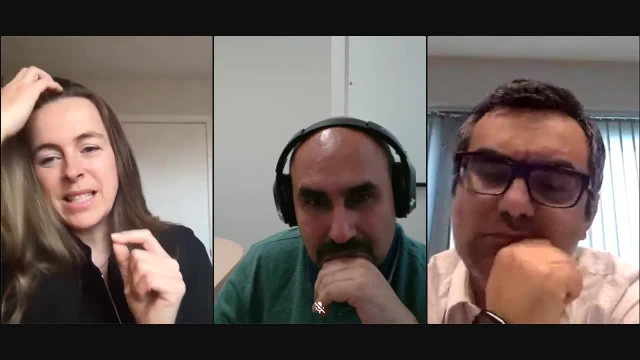 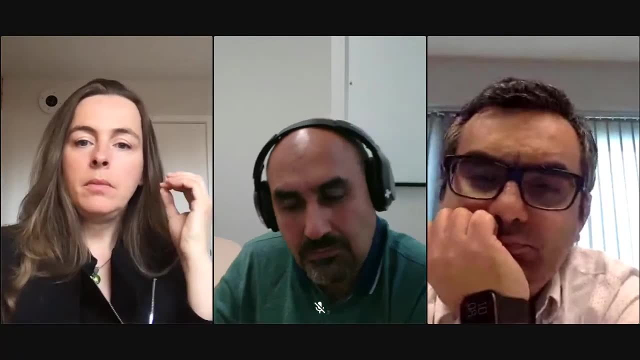 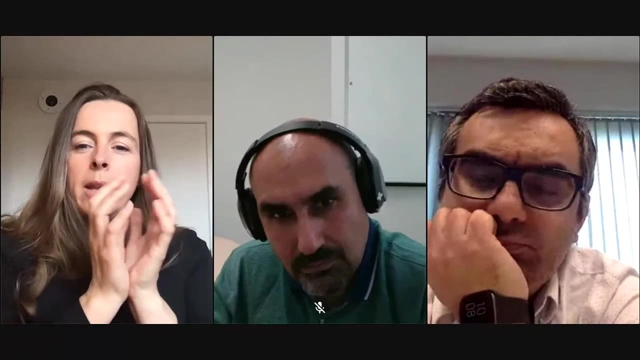 looking for you customize this, and so this is, I guess, a message for everyone. it's not a one fits all approach, and this is why I love working with Castor so much is because we didn't say we're going to work on this one organ. 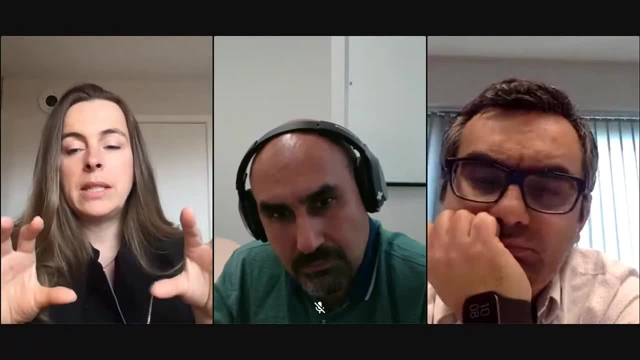 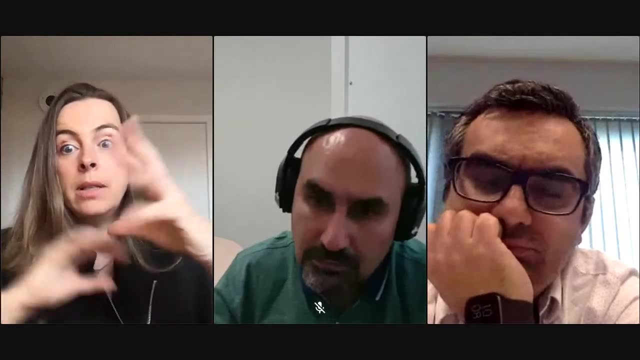 and make a full instrument. we are having enabling technology and we say: let's find the best people in the world to do lungs, to do eyes, to do cardiac and now. but I don't have to be the expert in everything I'm much happier to do. 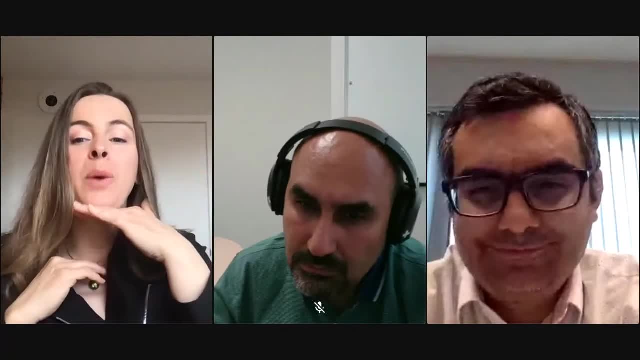 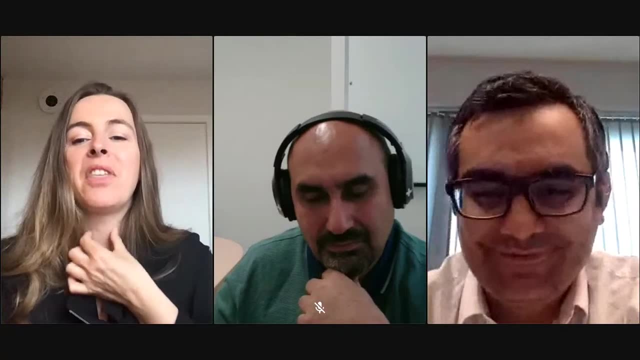 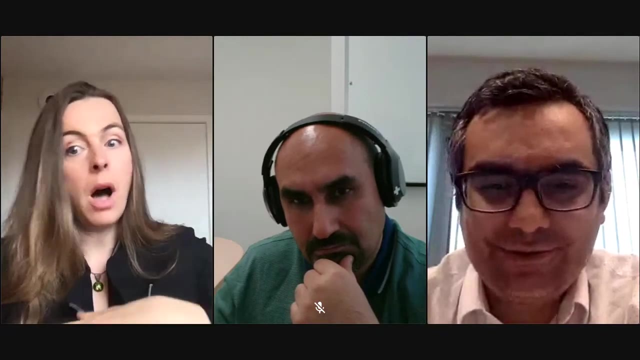 head and neck. arguably, I'm only doing neck. Frédéric Leblanc is doing a fantastic job at the brain, so I'm staying with parathyroid and vocal folds, but the technology assists and enables people to do all sorts of fun stuff: gastro, cardio, brain and so on. 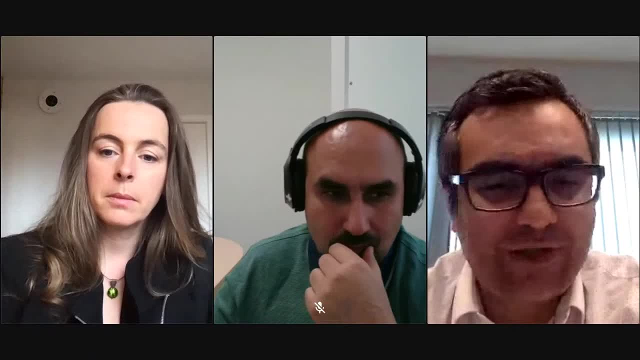 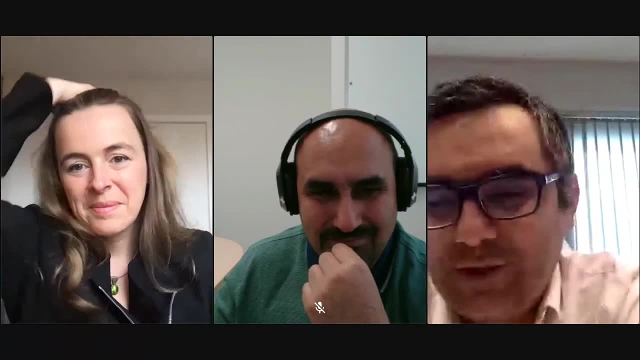 neuro and so on. that's great, and we have many people from different backgrounds here on the call as well who might be very interested to work with you on this interesting technology. Hooman is one of them, I'm sure. so, Hooman, do you have any? 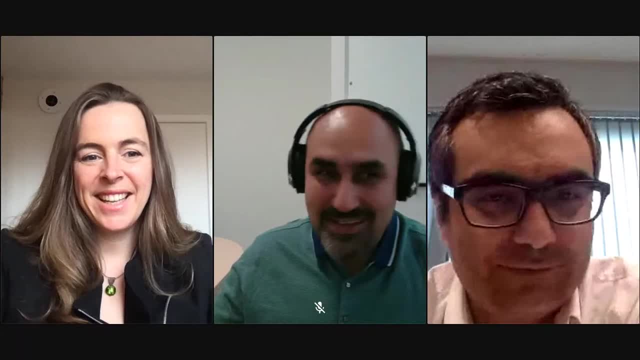 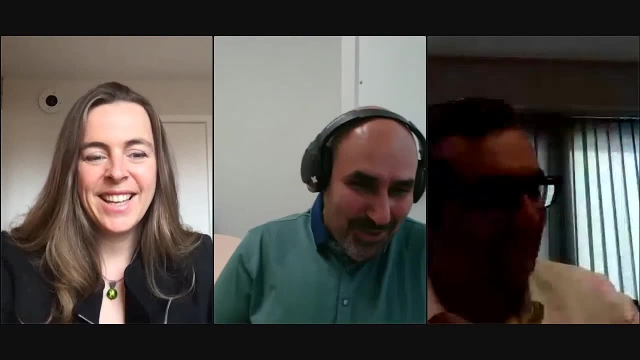 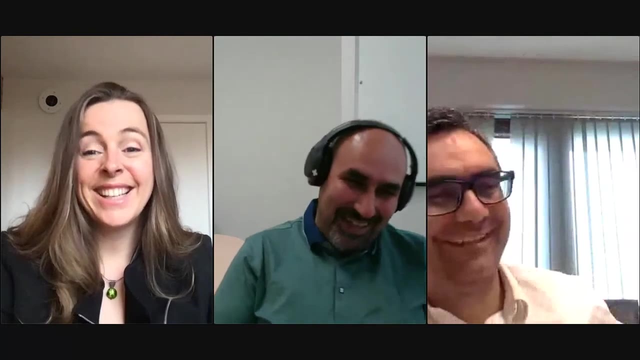 questions to ask. I don't have questions, but I really enjoyed and I was learning and I just want to also go back to my PhD, when Caroline was the chair of my committee and you know she gave me lots of homework to read about convocal microscopy. 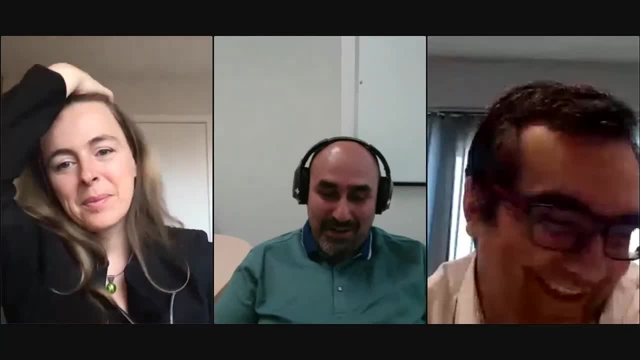 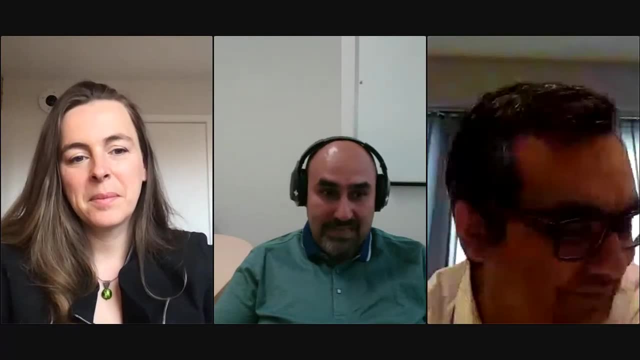 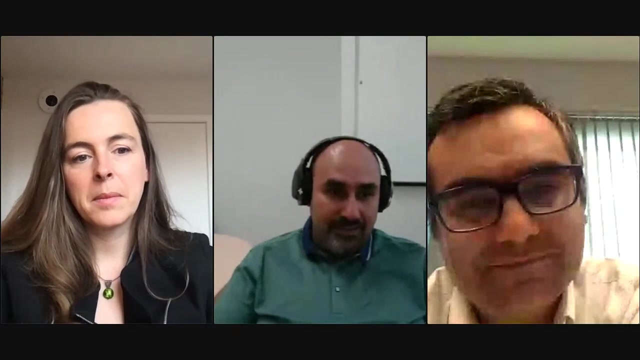 and all the modalities and the stuff. so from that time I really learned a lot about the physics behind the imaging and I'm now asking my students to do that because they go to the microscopy facility here. but if they don't know the behind the scene, 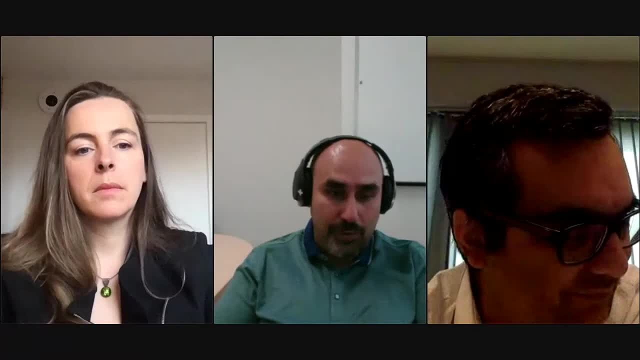 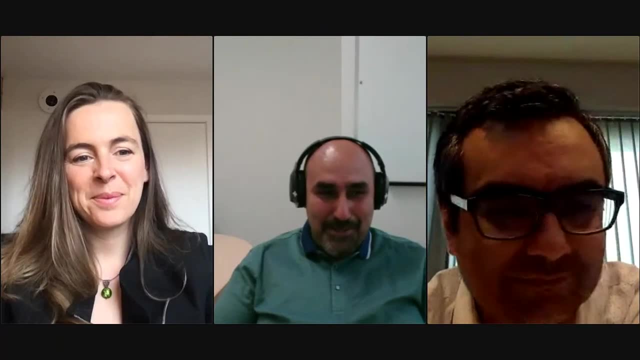 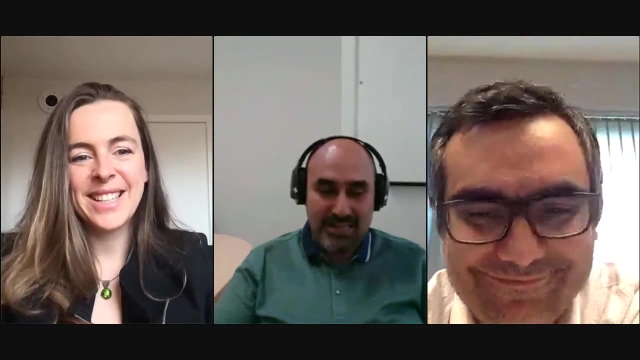 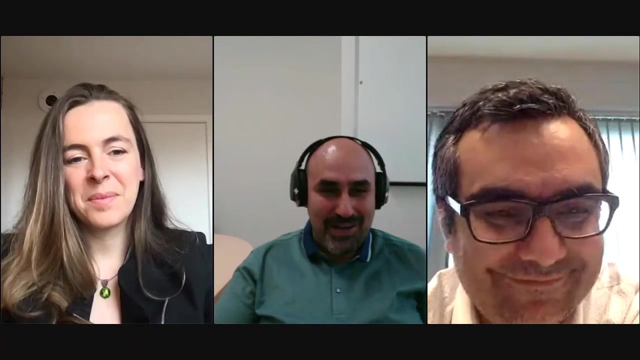 they can't really choose the right objective and the right modality and all this stuff, the fluorophore. so that was really helpful. thank you, Caroline. we can talk offline about some kind of collaborations on cardiac, on cells and on tissues. so, Mohsen, and if you have anything, 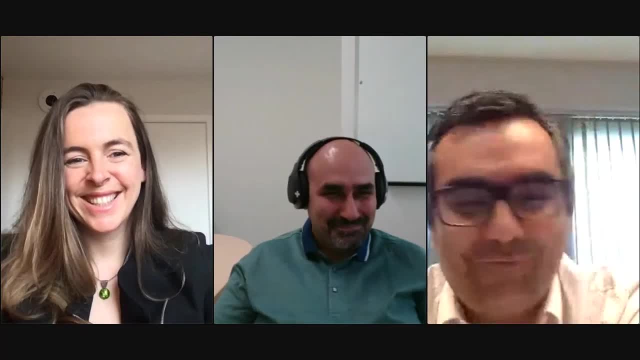 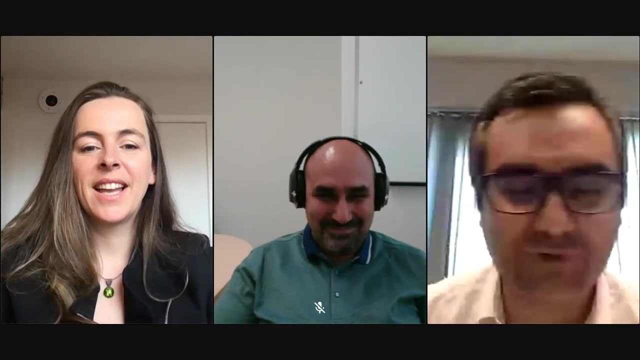 to add Mohsen or Caroline. you can go ahead. I don't have anything. one more question, Hooman, because I wanted to give you this opportunity. you know that I ask questions a lot, and if you don't ask me to stop, then I'll keep asking. 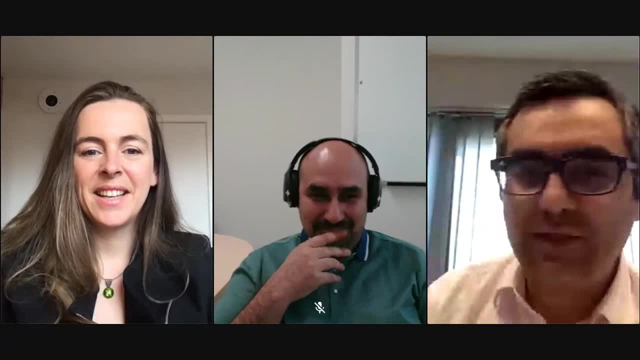 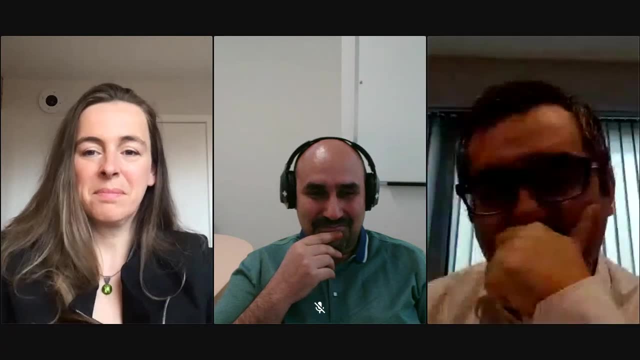 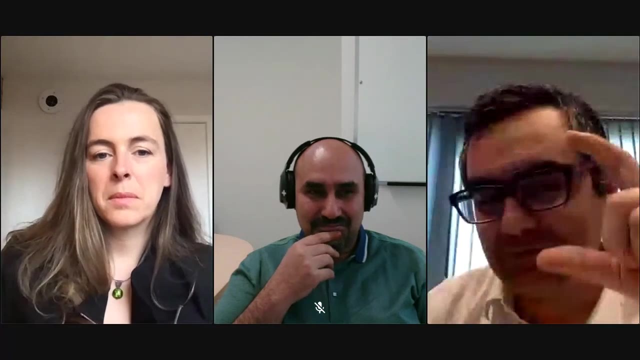 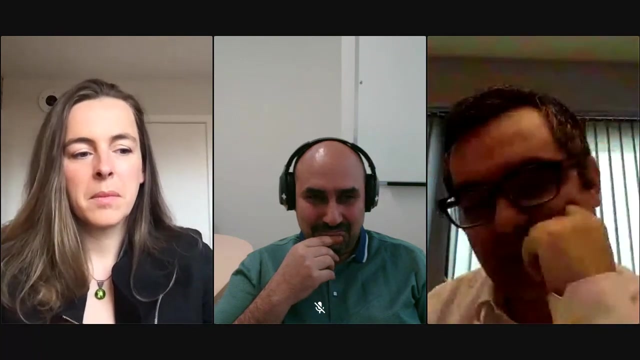 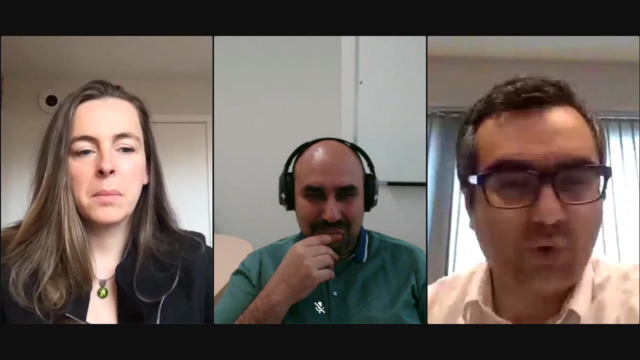 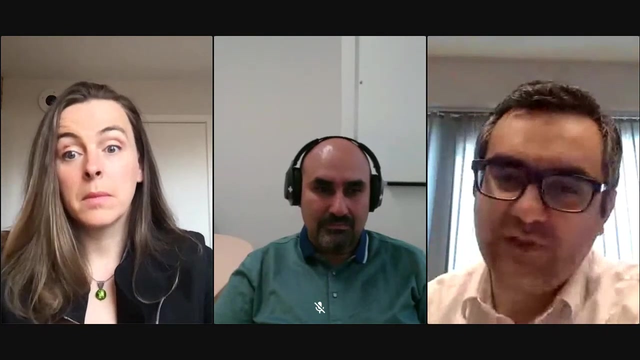 so this is very interesting about the microscopy. it is a very interesting thing about the microscopy. it is a very interesting thing about the microscopy, which is about how to use microscopy and I think, the way that microscopy is used in the, in the, in the, but they do not have the capability to do confocal. so do you see this? 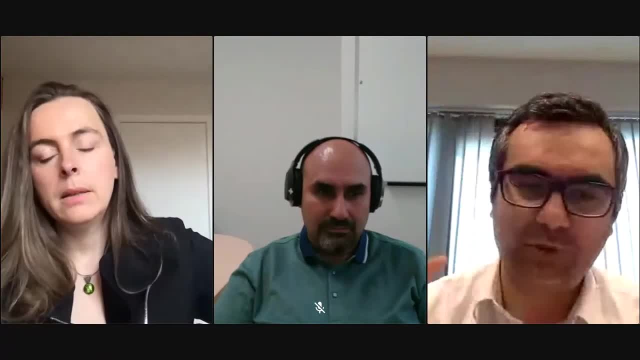 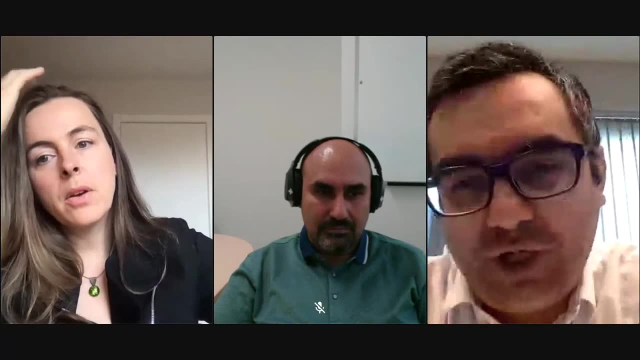 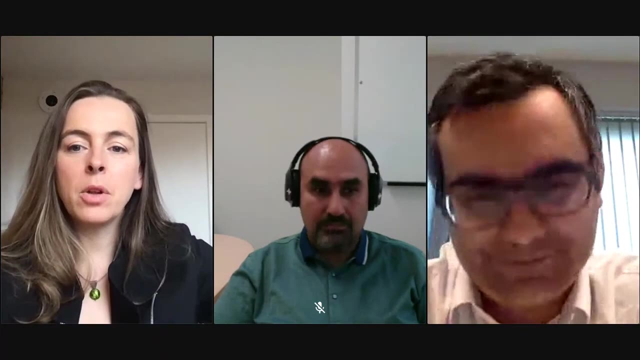 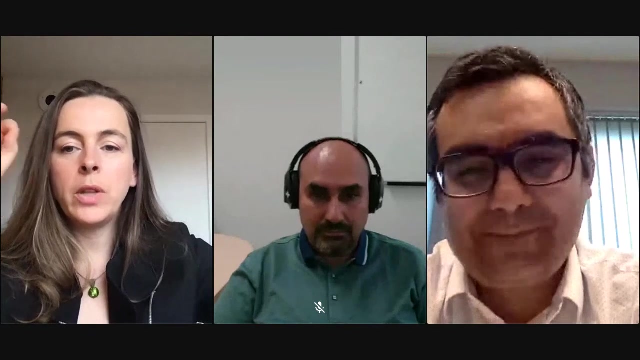 technology being used, as you know, being integrated into this low-cost mini microscopes. I think this is this is a great direction. the field is going using holographic and lensless microscopy and I think the pioneer- and this is that UCLA. I do an Oscar he's doing like just great, so we were, we're in the same lab. 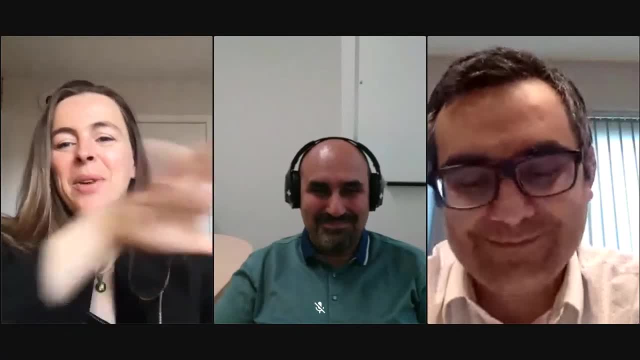 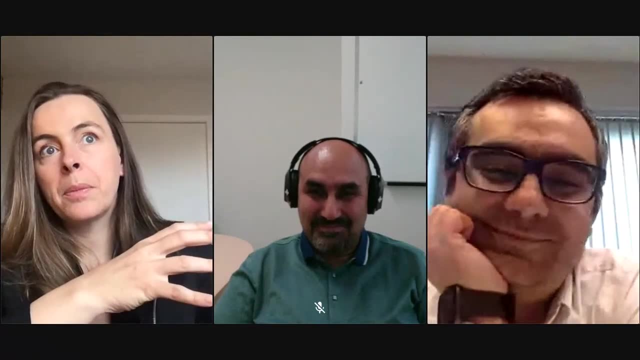 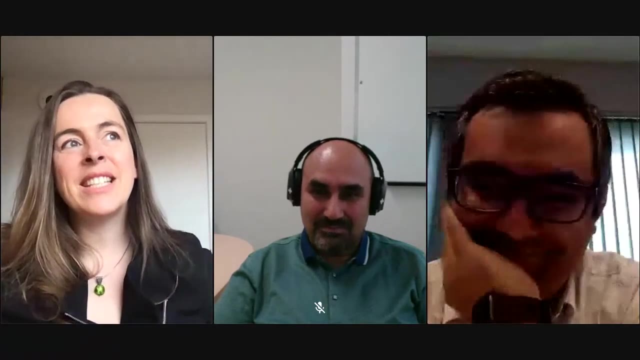 during his postdoc and my PhD, but it's always the same crowd who. so he's exploiting light a different way. so I'm sort of killing the phase and he's exploiting it. so, but as long as this is why the physics is so great, physics is 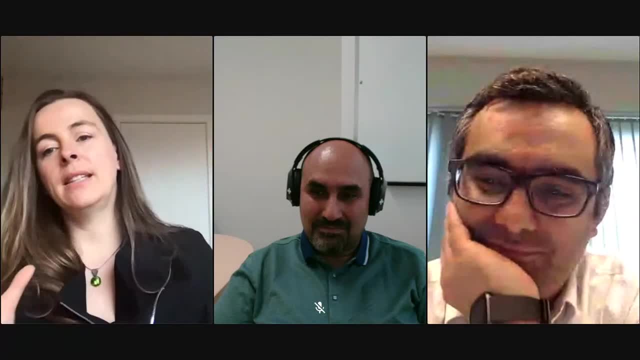 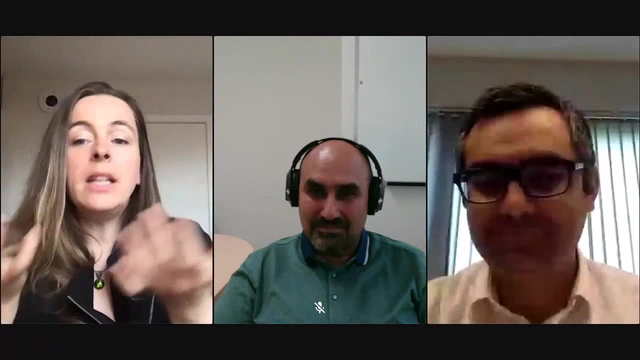 your tool set is your palette of colors, right and? and you have the phase, you have the amplitude, you have the wavelength, you have the gating, so and then, and then you exploit it whichever way you want. I decided to kill the phase and he's exploiting it, but 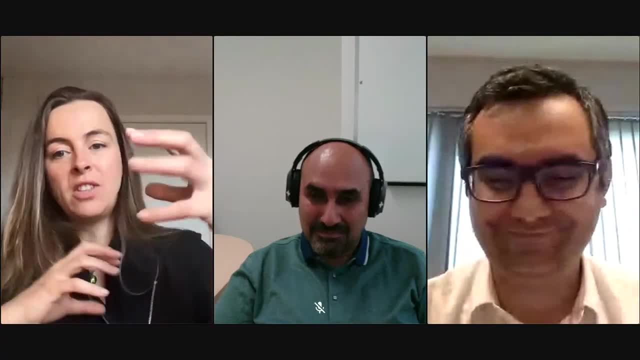 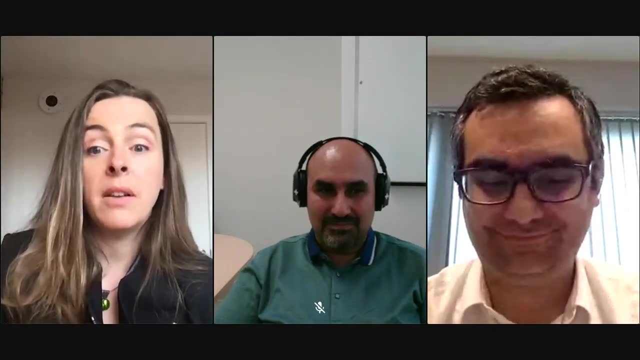 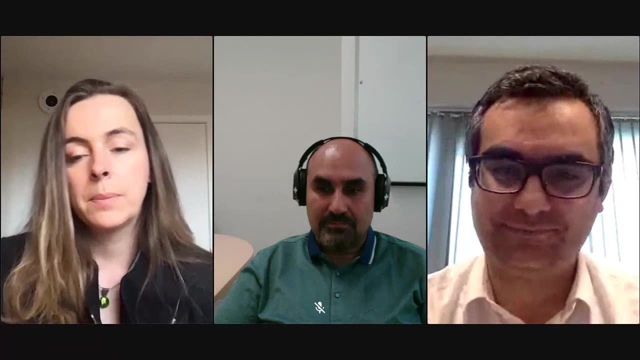 both. again, there's no one-fits-all answer. you need to look at your application and and I think if they were for for cell incubators, I would definitely go the lensless approach and get the optical sectioning for confocal you using items technology. I see okay, good, but I'm quite familiar with either guns. 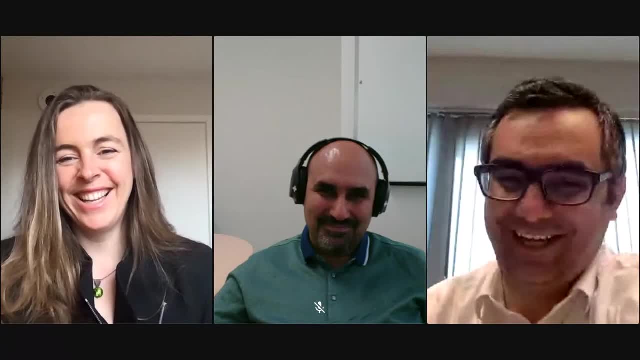 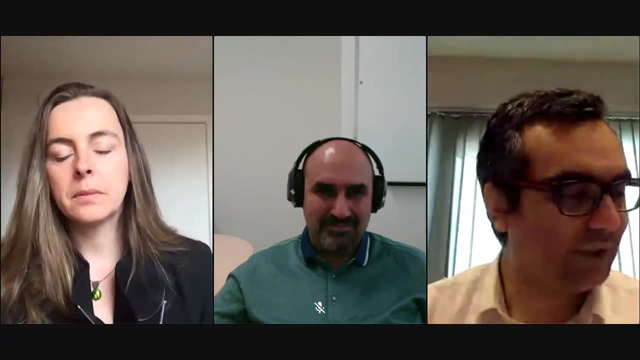 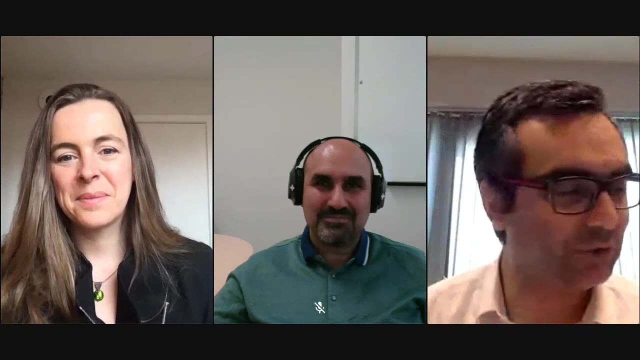 technology is working on this, also this sensor arrays as well, which is very interesting to me. well, so so I think I already asked my questions. you answered many of my questions yet during your talk, and that's a that. a good talk is that the presenter answers the question why. 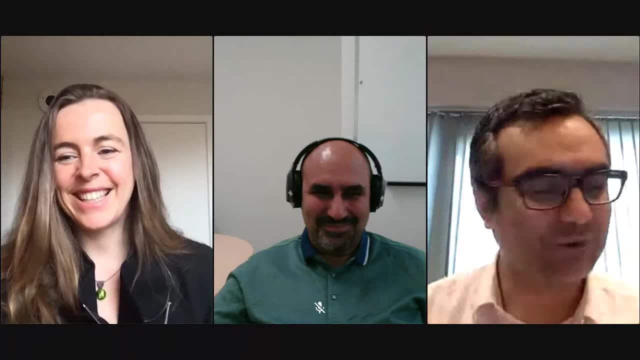 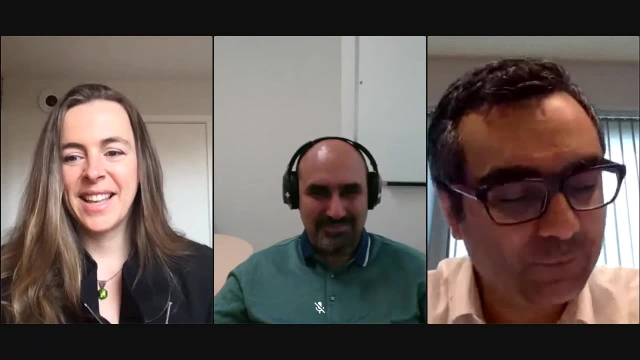 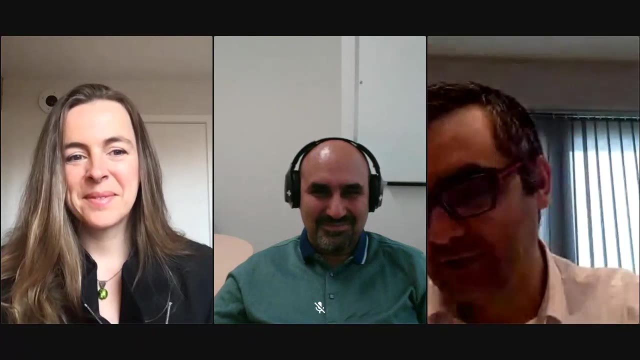 they're talking, giving their presentation. it's very interesting, so I'd like to thank you again for your for accepting our invitation. we we were very delighted to have you today with us. I really enjoyed your talk and then seems that many of the participants are also. they have enjoyed your time and 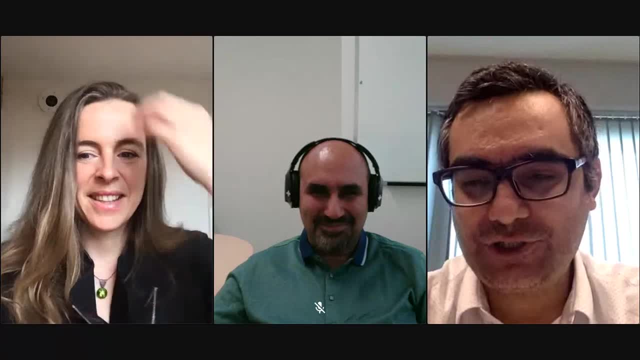 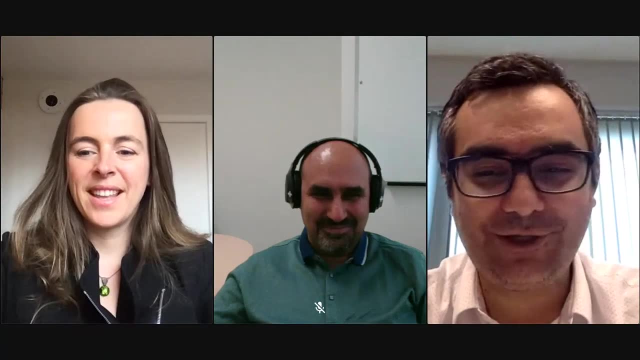 then you stimulated us to think about different technologies, so we will be in touch with you. I'm sure Michael will be in touch with you, so I think we should have it like you know, I think, whom and Michael, you and myself, we should have a separate meeting and then discuss, because I see a lot of